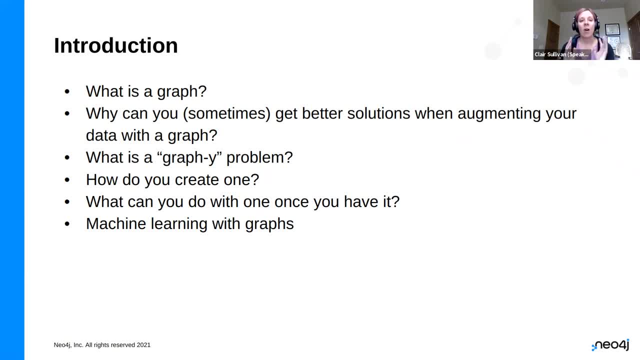 one of the links is a GitHub link, which will have all of the slides, the notebooks that I'm showing, etc. So stick around for that. So we're going to start just with the basic introduction. what is a graph? But then why might you want to use one in a normal data science? 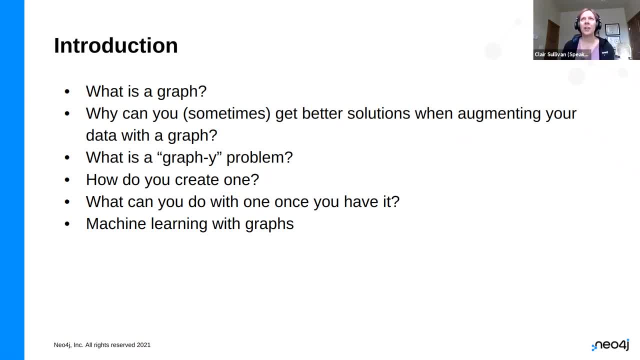 workflow. And then what is a graphy problem? I think there's a there's you know a perception that graphs are. you know what you do with social networks and stuff like that, And hopefully I'll be able to motivate you that it's actually a lot more than that. We'll talk about how to. 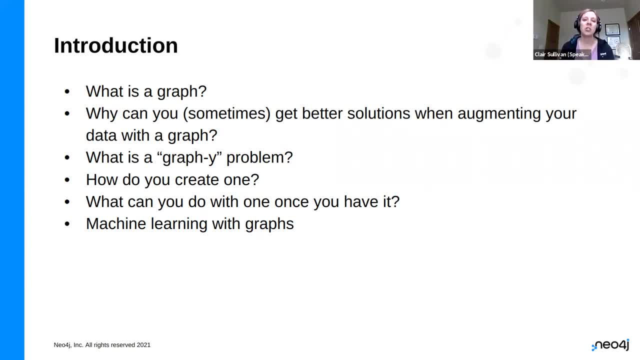 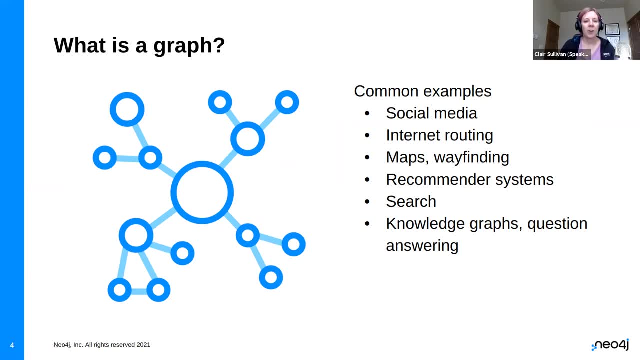 create one, and then what do you do when you have it, and then how you can get into machine learning with your graphs. So let's just dive right in. We all know about social media with graphs And you know we've got this concept of nodes, which are these: 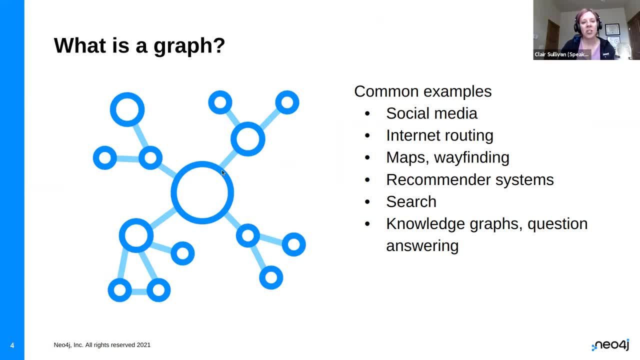 circles and they're connected to each other with edges or relationships. those are the lines connecting the circles. So you know, we think about who are our friends or our followers on. you know, pick your favorite social networking sites, But it's a lot more than that. So we're 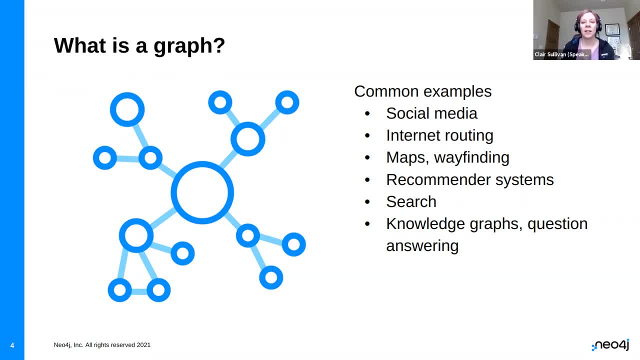 going to talk about some of the terms with with this and how we can calculate some good stuff. Internet routing is another great example of a graph understanding what network connections are going where. maps and wayfinds That's. that's pretty much how Google works. is Google Maps works? is with graphs? recommender. 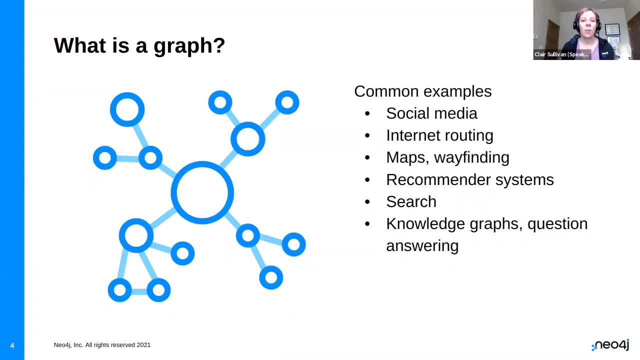 systems. Now we're starting to get a little further outside of the more obvious places. I'll show you a recommender system example in a little bit. Search, all of search with Google, is based on this next bullet point: knowledge graphs, question answering. these are really hot areas right now in 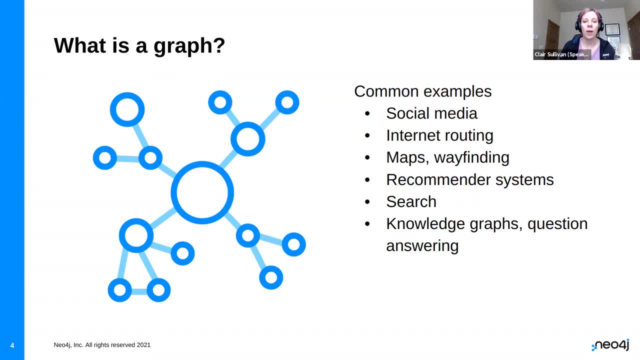 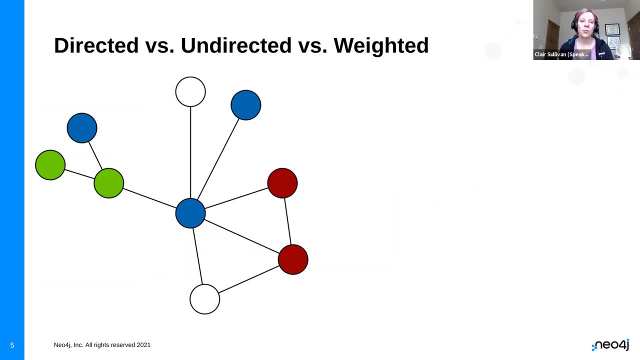 graphs and, in natural language, processing. So we'll talk about that a little bit as well. Just some terminology. Here we've got some terms that we use with graphs, such as directed graphs, undirected graphs, weighted graphs. what I'm showing here, I have nodes and relationships, And you see that those nodes they're 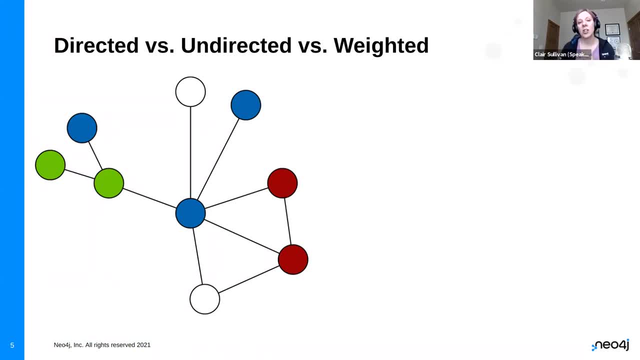 connected by relationships that don't have an arrow, And what that suggests to us is an undirected graph. An example of an undirected graph might be something like Facebook. if you're friended with somebody on Facebook, they are friended with you, So that is an undirected graph. Now we compare. 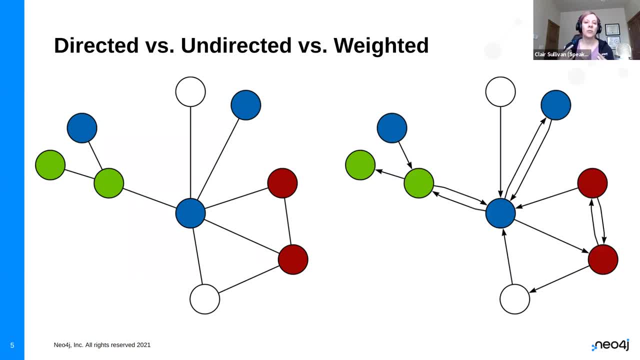 that to a directed graph where you can see. now I've replaced those edges or relationships with arrows And the arrows indicate the directionality of the relationship. So, for instance, this would be like Twitter: somebody can follow me on Twitter, but I don't have to follow them. If you look at the 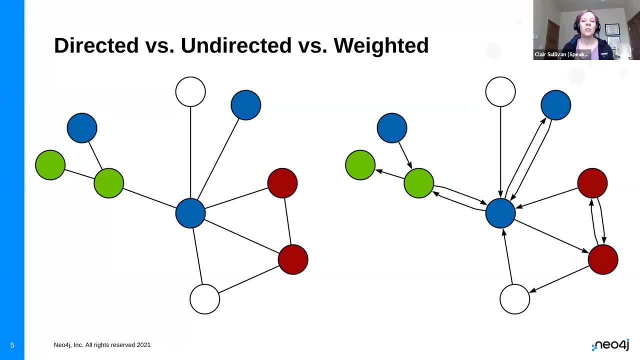 the far left of that graph with the blue and the two green nodes. I can see that the blue node is following one of the green nodes is following the other nodes. I can see that more central green node is following the center node and the center node is following them, And then I can see that the 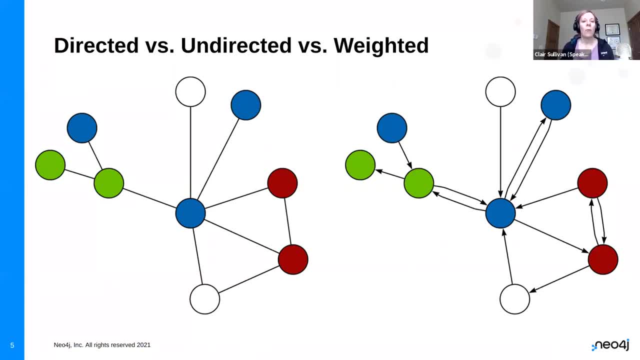 left link is a little different than the right link, So again, this is a Twitter like model. then we can talk about weighted relationships. So in a weighted relationship we might be indicating the strength of that relationship. Maybe the larger number indicates the strength. So the strongest relationship. 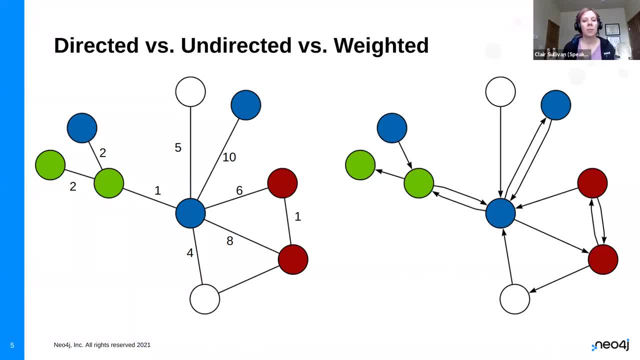 here is that central blue node to the upper right blue node. it has a weight of 10.. That's really great. Or maybe we do it the other way around and we talk about: Well, how long does it take me to drive from one place to another? I see those two nodes are two red nodes are connected by a weight. 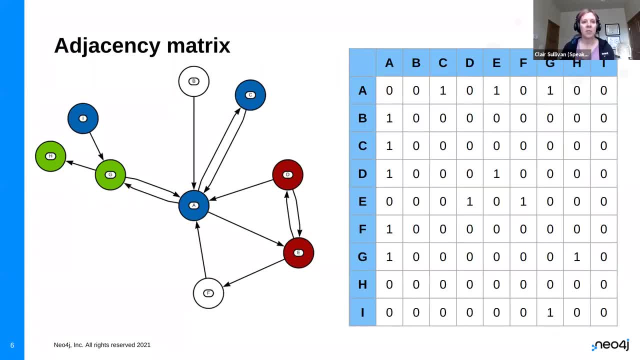 of one. So you know, that's kind of how we can use these different types of graphs, but how would we do math on them? So what I'm showing here- and this is going to kind of be the crux for a lot of- 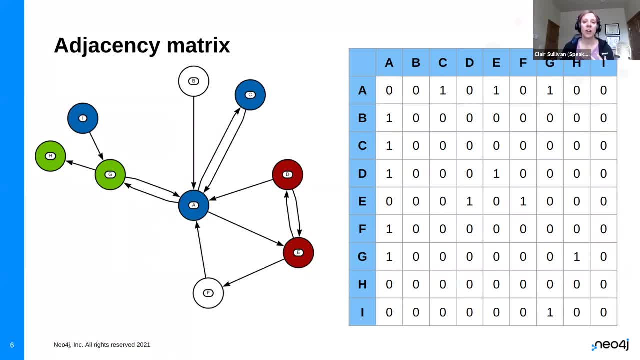 machine learning is, we can convert those graphs into a matrix, a matrix of, say, ones and zeros, or maybe you could replace those ones with what the strength of the relationship is. So I've given each node a label: A through H or, I'm sorry, A through I, and if there is a 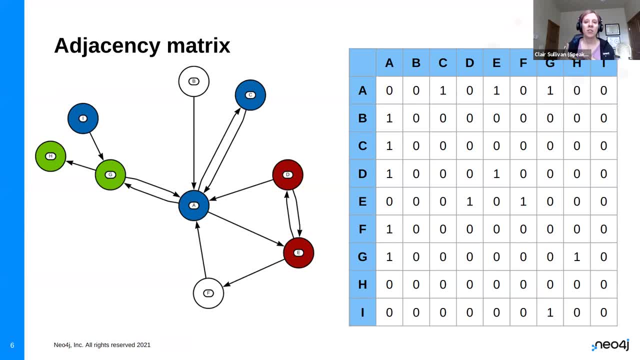 connection between two nodes. what you see is that there's a one in the column, So, for example, that top row A is connected to C, so I have a one there, whereas C is also connected to A. So I look at the column and I can see that one relationship there as well. I can see that H is not well. 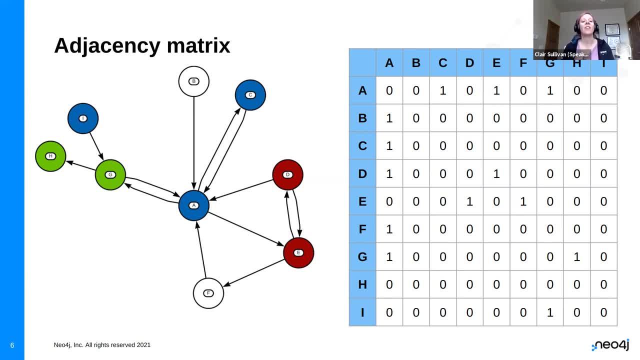 H has an error in it. H does not have an error in it Why? Because what I am showing is that this is a directed graph. H does not have an arrow going out of it into another node. So that's why, in a directed graph, 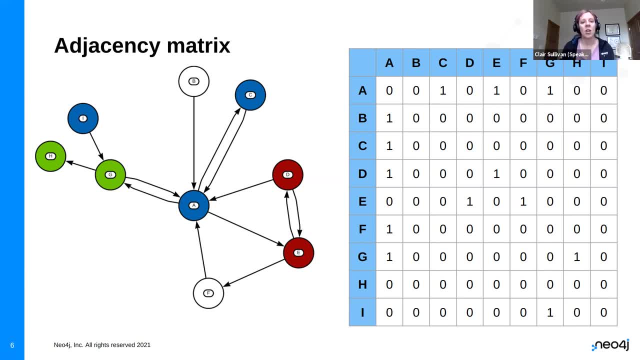 I don't have any values of one within H. Now we can talk about several different things with this graph. We can talk about degree. Degree would just be the number of arrows coming in and out of a node. So you can see that A, for instance, has a very high degree. We can further simplify that. 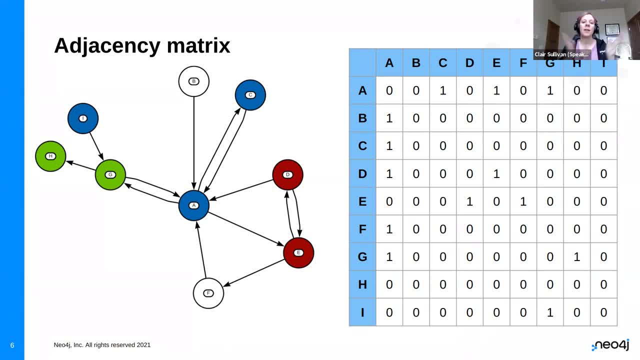 to in-degree or out-degree. In-degree is how many arrows are coming in. Out-degree is how many arrows are coming out, And then we can talk about the number of arrows coming in and out of a node, And there's all kinds of things that we can calculate based on this. But let's talk about 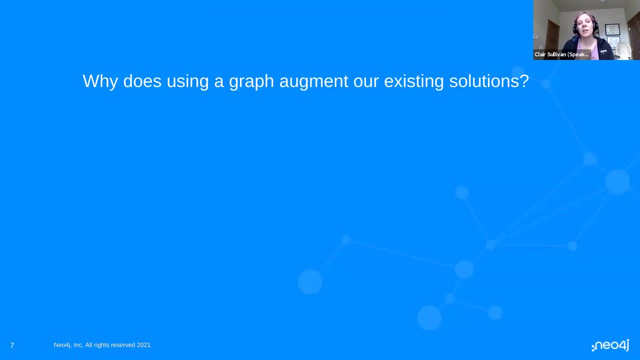 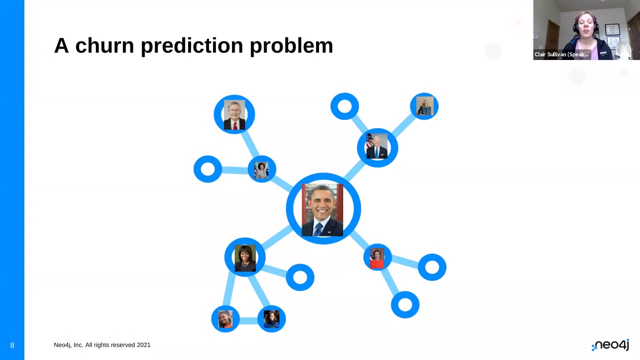 why we care. Why does using graphs potentially augment our existing solutions? I'm going to talk about two common machine learning problems today, and why a graph would do better. So I've created this simple social network here. I have Barack Obama in the middle And the nodes that are. 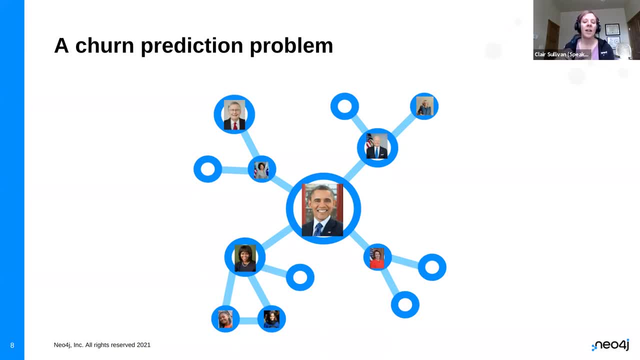 connected to Barack Obama are Michelle Obama. Nancy Pelosi is kind of that small one down about the four or five. I have Joe Biden in the roughly two o'clock position And I've got Elaine Chao, who's Mitch McConnell's wife. Let's assume that there's a relationship between Barack Obama and her, And then I'm going. 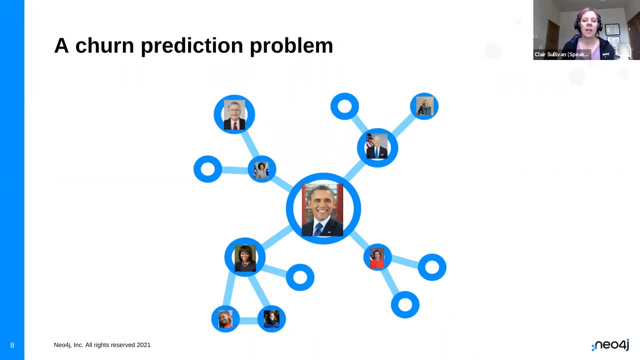 to have this concept of the importance of nodes, And we'll talk about what that means in a minute. But in this graph, Barack Obama is hugely important because his node is big. It's represented by this big node, And I have medium-sized nodes and I have small-sized nodes. Now, one of the things that we 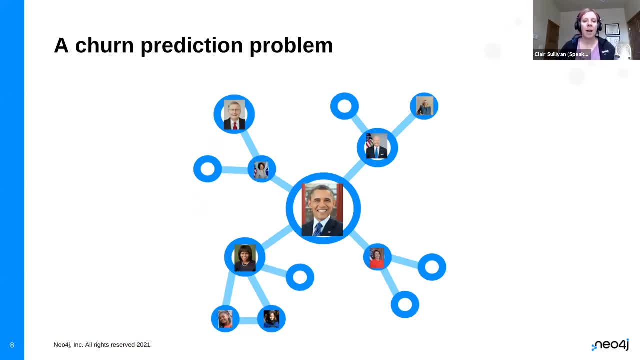 can do is churn predictions. So we might have a lot of data about each of these characters And that data is presented as a vector. We've got embeddings And we try to use those embeddings to determine what's the probability of any one of these nodes in the graph churning Well, that's. 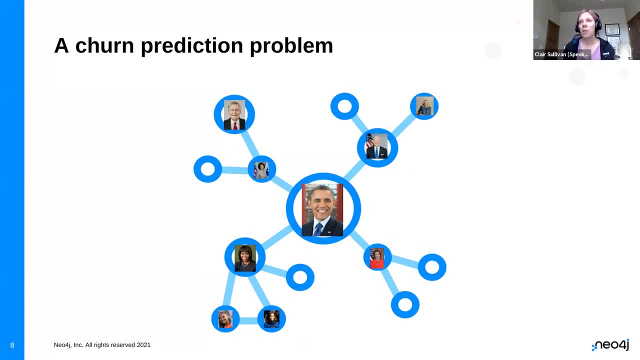 great, And we can do that, And we can come up with a model based on supervised learning. We know that people with this particular vector tend to churn more than people with this other type of vector, And that's great. The catch, though, is, if you think about social networking, let's say, one of these people decided 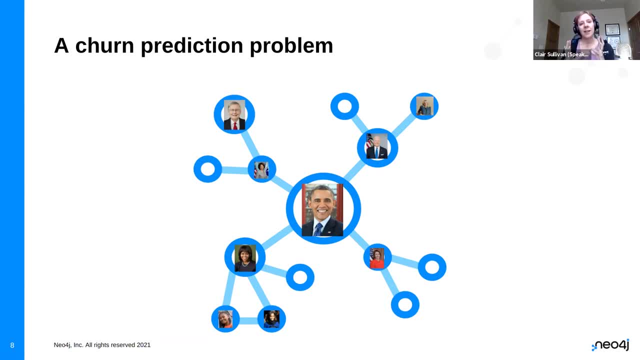 to churn The idea around a graph is this idea of homophily, which is that the neighbors in a graph tend to behave similarly to their other neighbors. So, for instance, let's say, Michelle Obama churned in this graph. Well, we have Sasha and Malia Obama there And they may say: you know what? 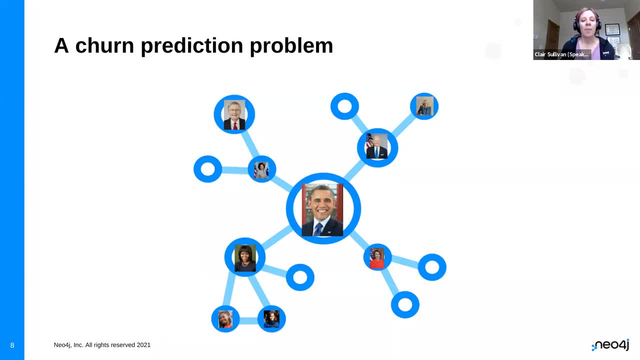 I'm not going to stick around because my mom just churned. Barack Obama can say: you know what? My mom left this platform So, yeah, it's time for me to get out as well. Now, what this has demonstrated is the importance of relationships within this graph, And those relationships within a graph. 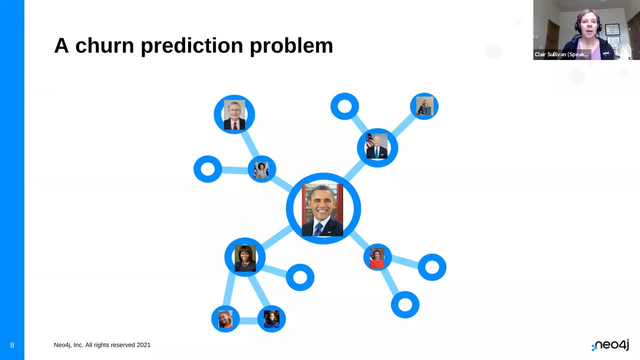 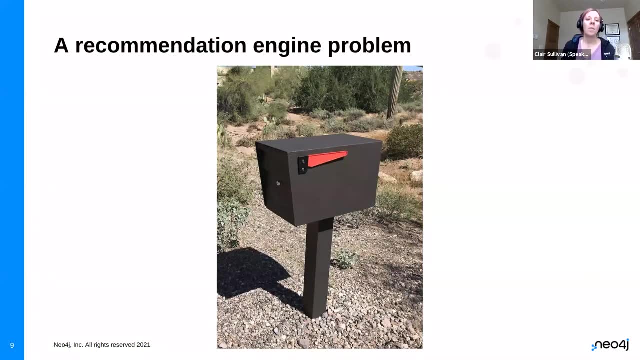 are treated as a first-class citizen. Let me show you another example, which would be a recommendation engine problem. So recommendation engines, they power so many things like sales and whatnot, And I'm going to give an example here. I'm going to give an example here of a mailbox. Now you might say: why am I showing a mailbox? 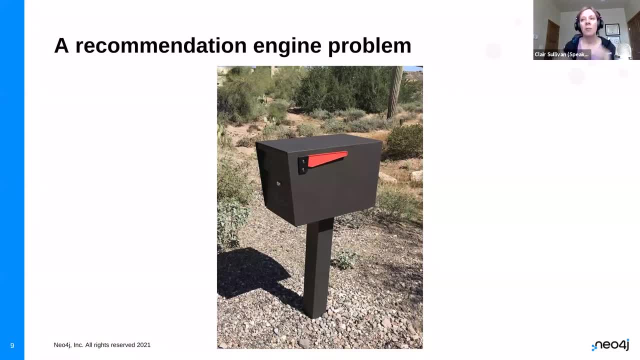 This is actually a real problem that I encountered when I was building my house here in Colorado. So I was building a house And a certain hardware store knew I was building a house because they could look at my purchasing patterns And they could say: OK, well, Claire purchased. 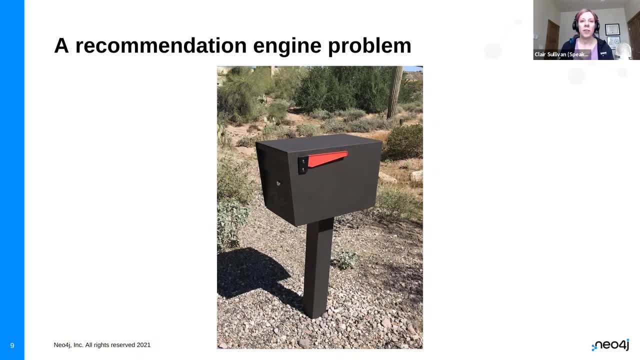 a bunch of nails and a bunch of wood. That sounds like Claire's building a house And they could recommend things to me for building a house, such as a mailbox here. And it makes sense to introduce me to a mailbox because if I'm building a house, I likely 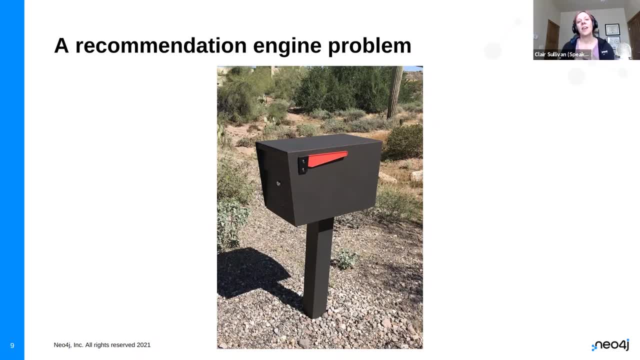 am going to need a mailbox at some point. Now, here's the kicker, though: is that I didn't buy that mailbox, or any mailbox. And why didn't I? Well, the reason being that there is no mail service where I live. Everything that we do is via post office boxes. However, our local hardware store 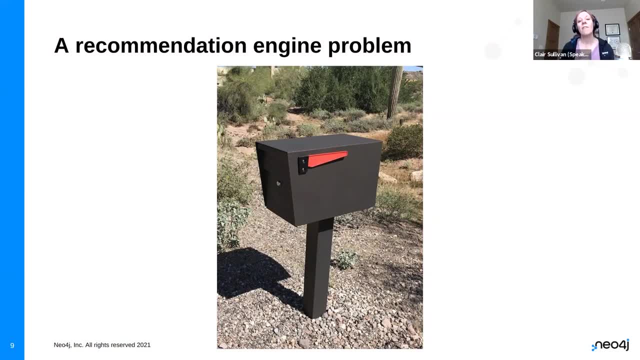 said, oh, there's a lot of people building houses up here, Great. And they actually have a whole row in this hardware store of mailboxes. And I said, well, why didn't I buy that mailbox? And they said, well, that's collecting dust because nobody here has mail service. Now, had we added some more? 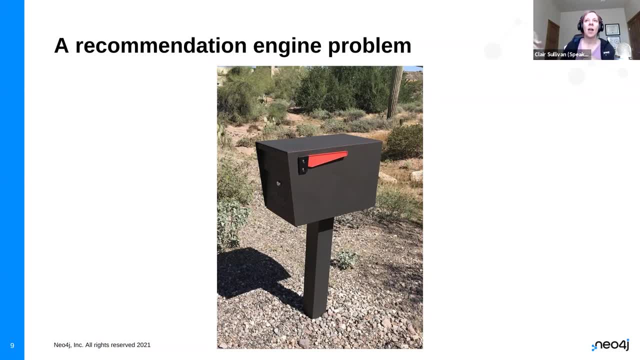 information into this data, Had we added relationships? For instance, Claire lives in this area here with all of her different neighbors, And none of her neighbors purchased mailboxes. So maybe the mailbox isn't the right thing to suggest to Claire. So these are two places. 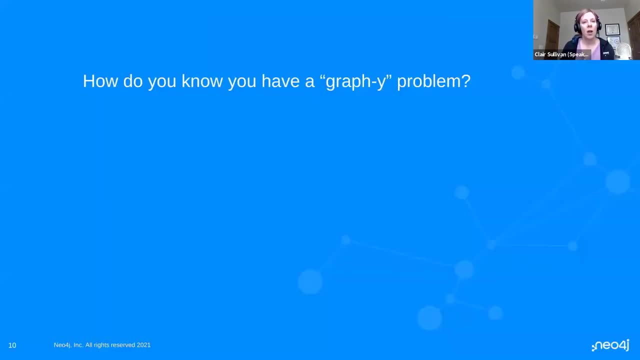 where relationships really would help us solve more problems. OK, But what type of problems? How do you know? you have a problem. that is graphy- And I use graphy in quotes. That's just kind of my silly made up term, But there's a lot of data that we don't ordinarily think of as being a 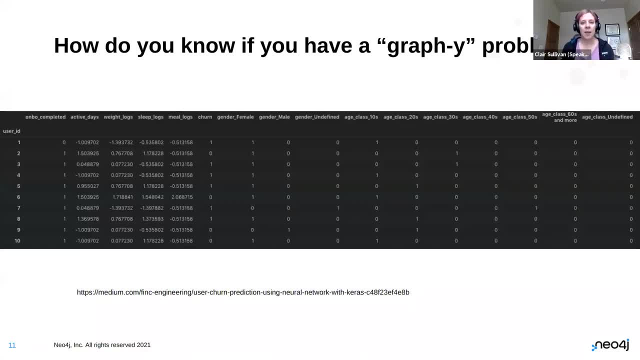 graphy problem, So we're going to look at this table here. This is normal tabular data that we're all used to using, And this is a churn example that you can find on Medium. And again, we talked about the importance of relationships, But let me give you a hint of when to know that. 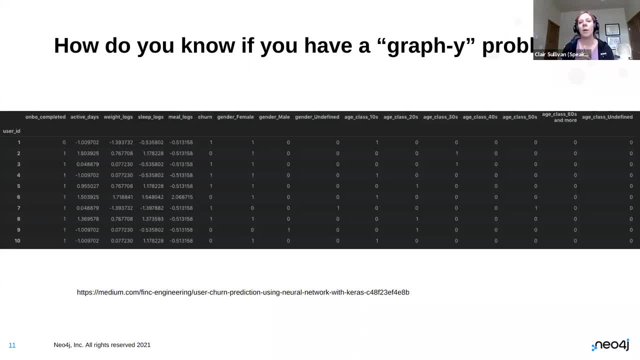 you should suspect you have a graphy problem. A lot of us use SQL. I'm going to be using a different database today, But think of it like a SQL database, except it happens to be a graph database In SQL. if we start having to do a bunch of SQL, 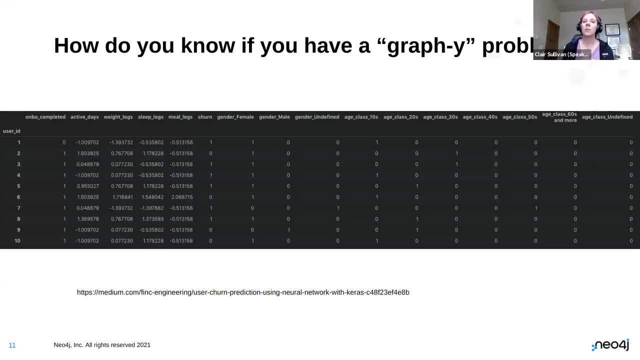 joins that might indicate that we have a graph. Now, SQL joins, as we all know, are slow, And especially if I'm having to join multiple columns on multiple columns within tabular data. One thing I had experimented with a graph database versus a SQL database, trying to just 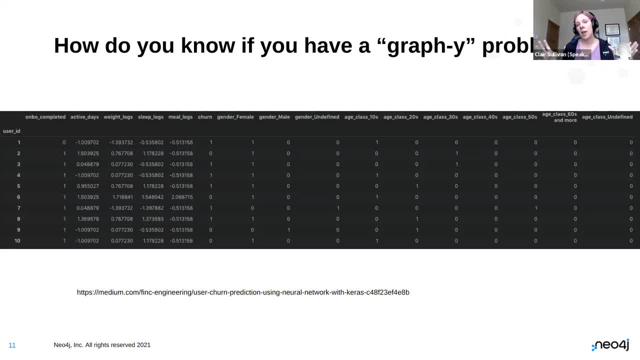 do traversal of these two databases And when I looked at a SQL database, the same join took me 1,000 milliseconds And it took me microseconds within the graph database, Because the graph database is set up to handle those joins and to navigate relationships. just for how databases 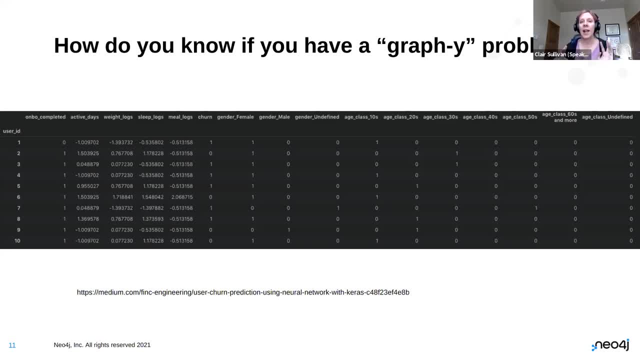 are stored. Now, I'm not a database person. I will tell you that if you're going to ask me what the nitty-gritty is inside of the database, I'm going to have to direct you somewhere else. But just as data scientists, let's keep in our hands. 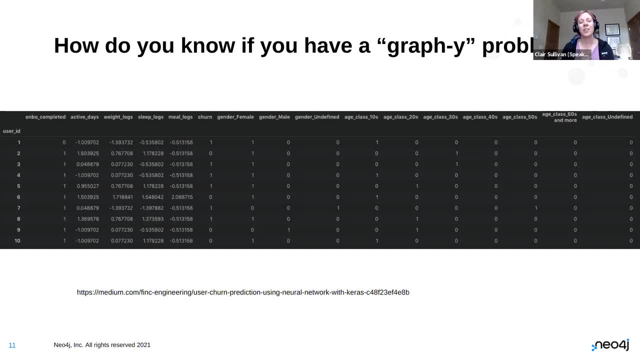 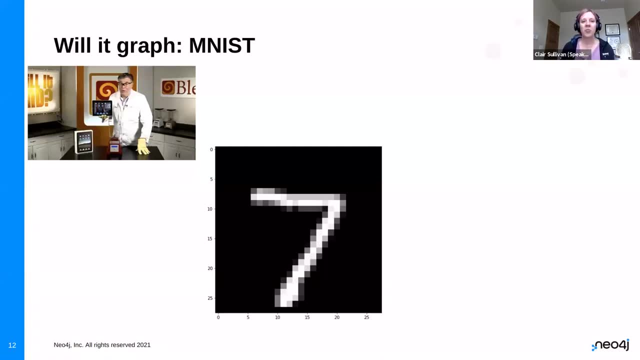 SQL joins, and particularly several SQL joins, should maybe be a hint that we have a graph problem. So we're going to engage in will it graph similar to? will it blend, for those of you who are familiar with that. And I'm going to start with one of our classic problems. 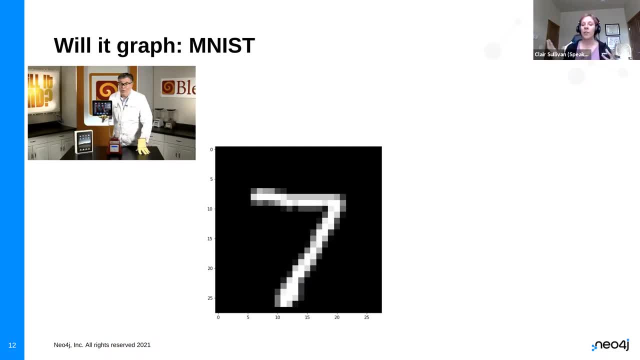 the MNIST problem. I think everybody who does any sort of computer vision problem, deep learning, we all look at the MNIST problem, classic problem: Will it graph? And the answer is yes. Here we have turned that image into a graph. Okay, Now you can see here. pixels are related to 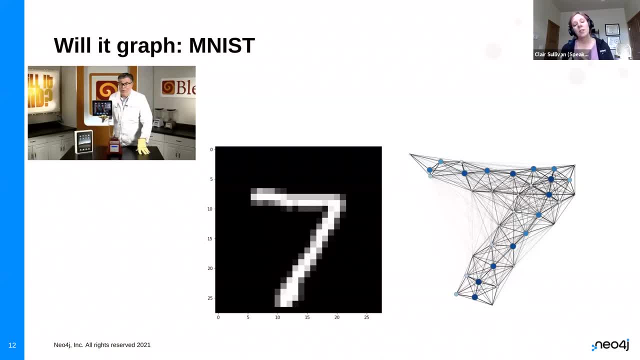 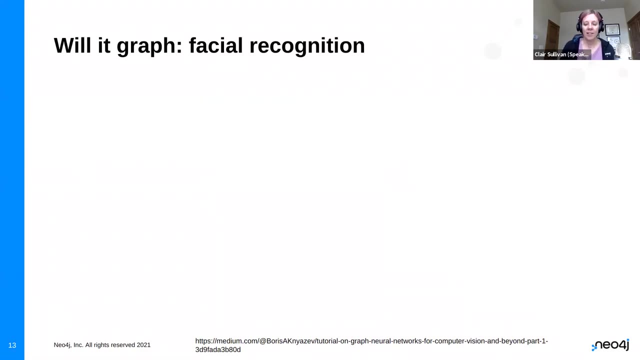 other pixels, Okay. So if I have one pixel that's bright in this image, we might suspect that neighboring pixels would also be bright. So, yes, you can absolutely look at MNIST with a graph. Okay, Facial recognition, Will it graph? Well, yes, it will. Let's look at these faces here. I 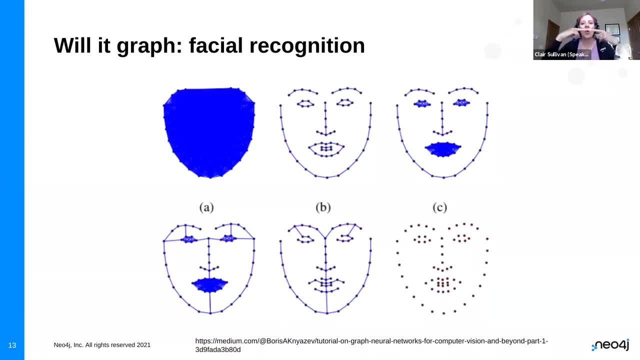 have nodes that represent a graph. I have nodes that represent a graph. I have nodes that represent the outline of a face and the nose and the mouth, And I can connect these points in any number of different ways. The point is that you know, say my nose, my nose is got. you know it's not going. 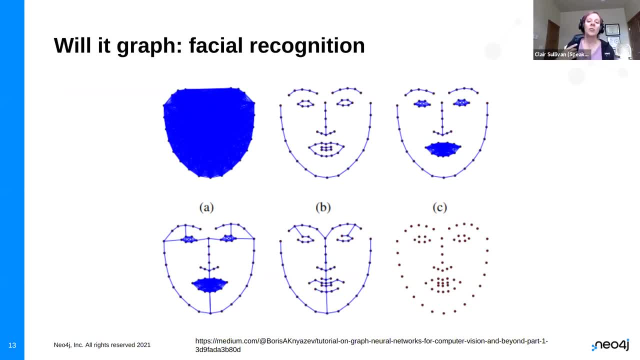 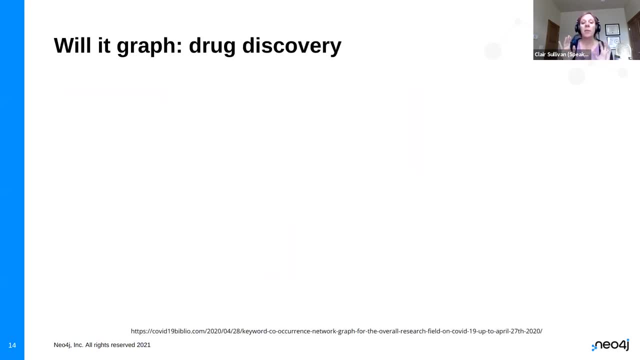 to all of a sudden stop until we get to the bottom of my nose. So again, this is the haemophily associated with facial recognition. Drug discovery: Probably this one's not going to be a surprise. Yes, it will graph. And here's two examples of that. First, we have some sort of molecule. 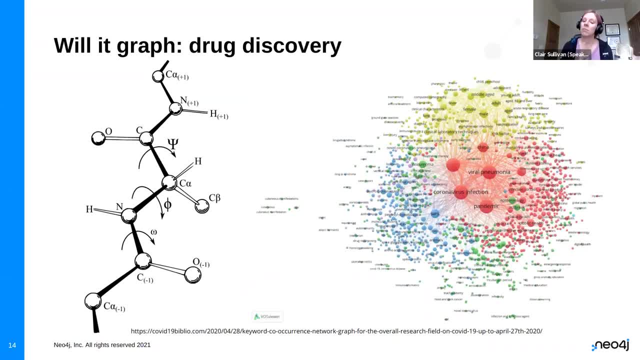 on the left. I'm not a chemist, Don't ask me what that molecule is, But I have different atoms connected through different other atoms. I have different strengths of connections, Like I might have double bonds between, like my carbon and my oxygen, And those can all be represented in a 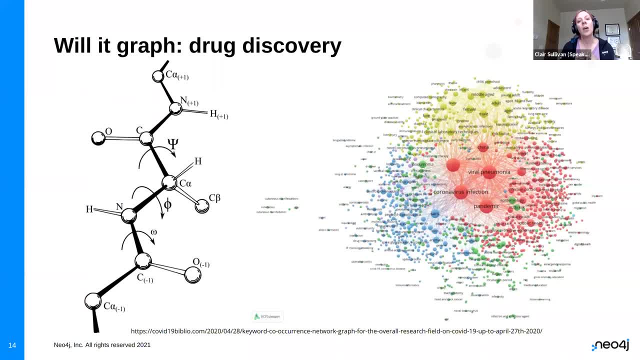 graph. Next example to the right here, What I have is I have a whole bunch of publications on COVID. This is obviously a hot topic And looking at what were the key words in all of those publications And so what you see here around- coronavirus, right in the center- you know that's obviously an 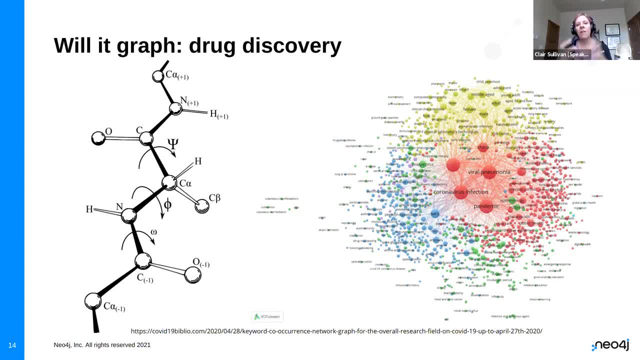 important node. I've got pandemic viral pneumonia. Now, if I start actually zooming out here, you'll actually see some medications that you could use. You'll see hydroxychloroquine in this graph. if you get in close enough, You'll see corticosteroids. So you know, looking at where, 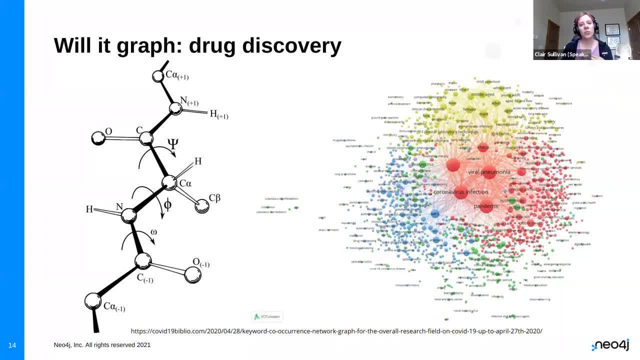 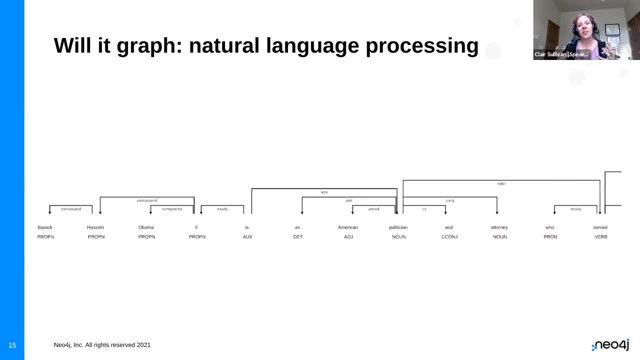 are the important drugs. pharmaceuticals within this graph could be a hint for successful treatments for COVID. Okay, Natural language processing- Will it graph? This is a fun one. I really like this one, And the answer, of course, is yes. You're probably figuring out the pattern here that all of these 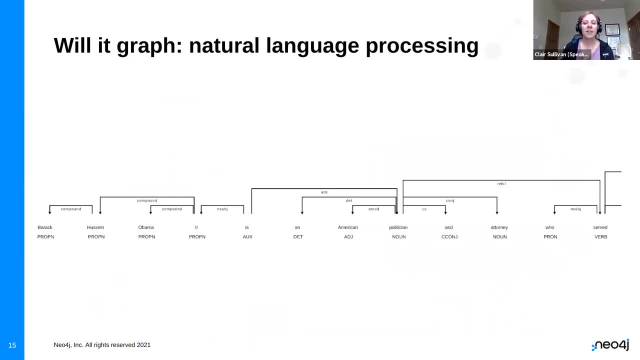 will it? graphs are going to be. yes, Here's an example. This is a sentence out of Wikipedia's, the first summary sentence for Barack Obama, And what you see this is the dependency graph. So we're looking at what words are dependent on what other words. Okay, And you know, here we have. 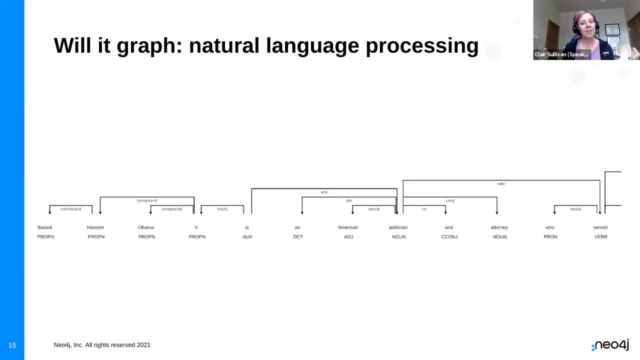 central nodes. Everything is coming out of like the word is. Is is considered to be the root And I apologize, this text is super small, But if you look at all of those arrows coming out, it's because is is a very important word, the root of the sentence, the most important verb in the sentence, And then I've 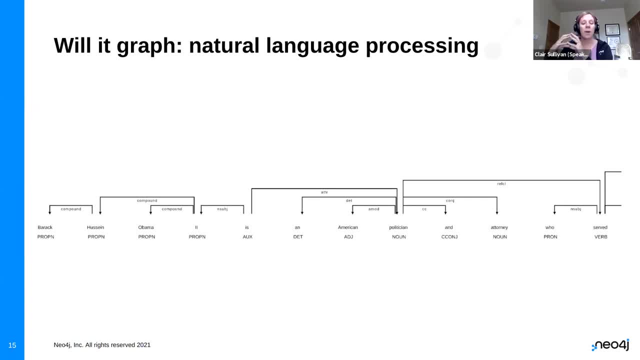 got a lot of arrows. I have a high degree associated with the word politician, So we might assume that Barack Hussein and politician are two words that should go together. So, yes, natural language processing, Absolutely. Here's a fun one: Body composition. 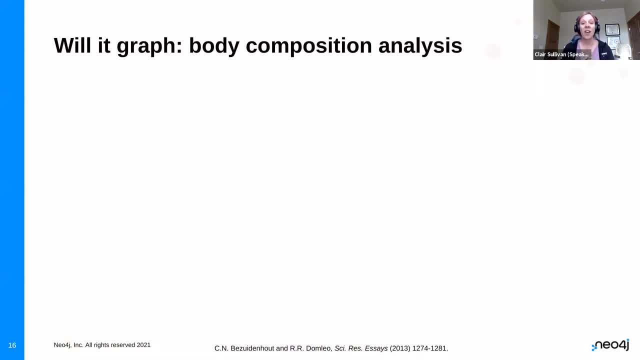 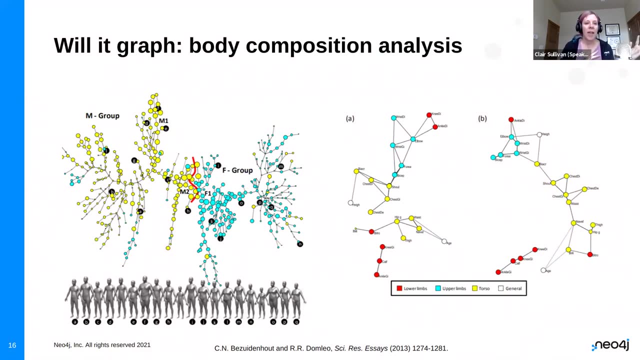 Analysis absolutely will graph. I didn't know that until I was preparing these slides. So if you look on the left, you can see different body shapes And they are broken down. looking at things on the right, like the upper limbs, the lower limbs, the torso and in general, 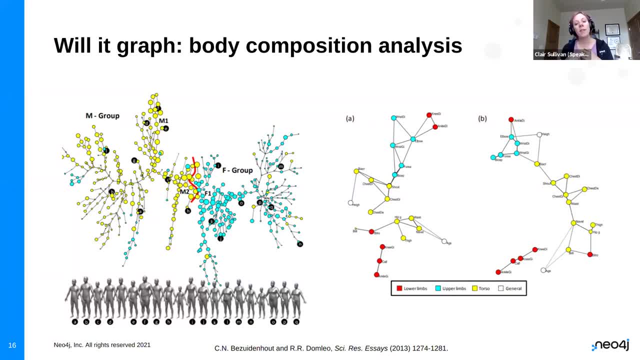 Those words, I apologize, are very small, But you will get a copy of these slides and the link to the reference for this is at the bottom of this slide. So we can see the wrist diameter, the elbow, The chest, chest diameter. Now, if I take all of this information, going back to the graph on the left, 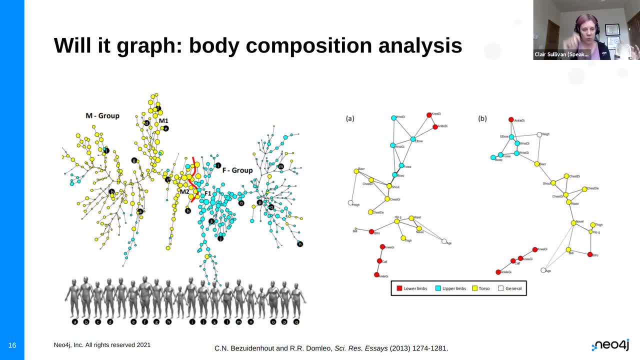 what we can see is that there's a distinct difference. You could draw this red line to separate which body compositions tend to be associated with a male body type versus a female body type. And don't ask me if we get outside of this bimodal version of gender here. but 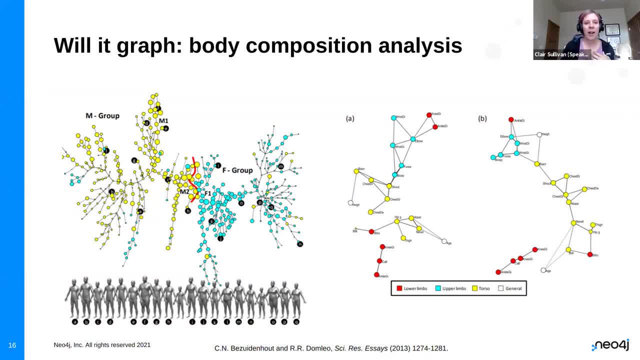 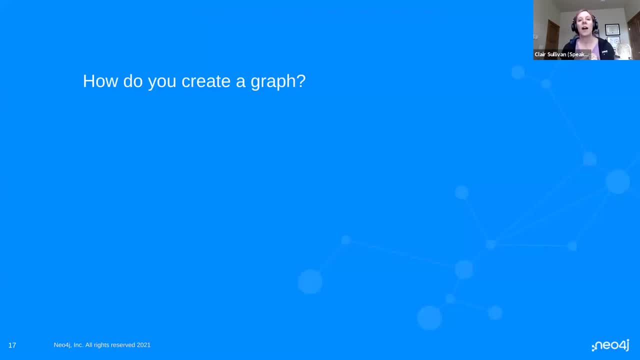 just looking at body type, those separate out rather nicely. Okay, That's all just intro. Let's go into how do I create a graph, Because I know everybody's going to want to get into this and want to get started with graph analysis, graph data science, graph-based machine learning. 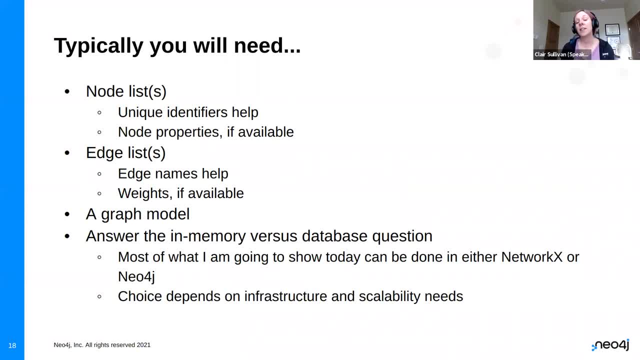 So I'm glad you asked: how did I create a graph? Well, there's a few things that you're going to typically need. You need a node list, Okay, So you're going to want some sort of list. CSVs are great starting points. 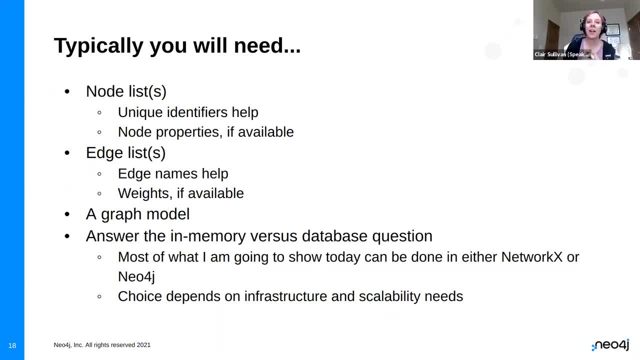 Of your nodes. It helps to have unique identifiers on them. It helps to have properties associated with them. If you have them, like the name of the node, maybe there's properties like the. you know, if I was talking about states like states in the United States, what's the name? 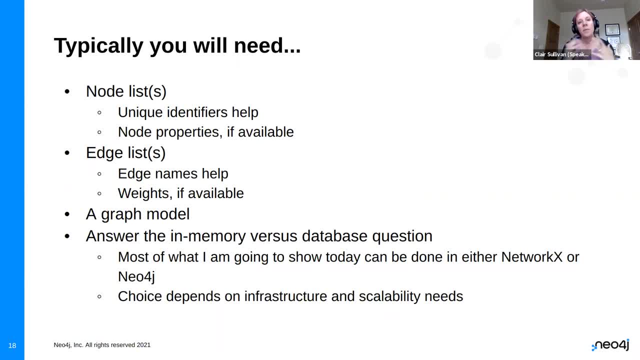 of the state. I could have geo coordinates for the state. Like we have a node list, We're also going to have an edge list And again edge names will help here. So I'm going to say node one is connected to node two through some type of relationship And again we can add our weights. 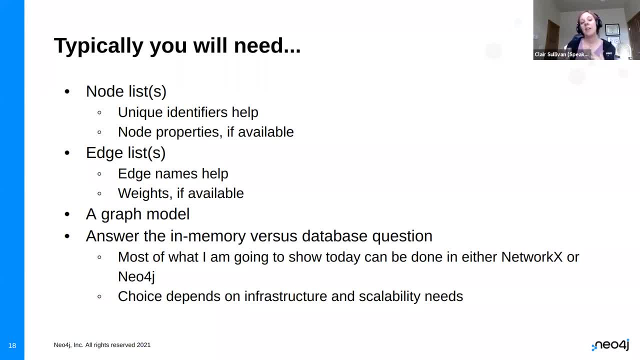 in here. Once we know what that data is, then we're going to develop a graph model around it And you know, you can think of those similar SQL models where we've got this table joins to this table to make that other table. This is kind of the same thing with a graph And I'll show you. 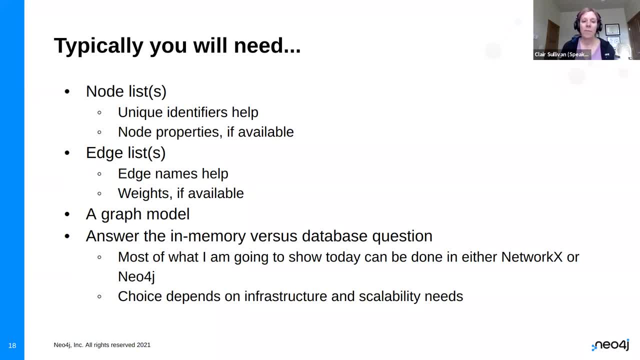 an example in a minute about why that's important, that we do that properly. And then, lastly, we just want to figure out where we're going to put it. Now, everything I'm going to show you today I wanted to let you know this can be done a variety of different ways. There's a common. 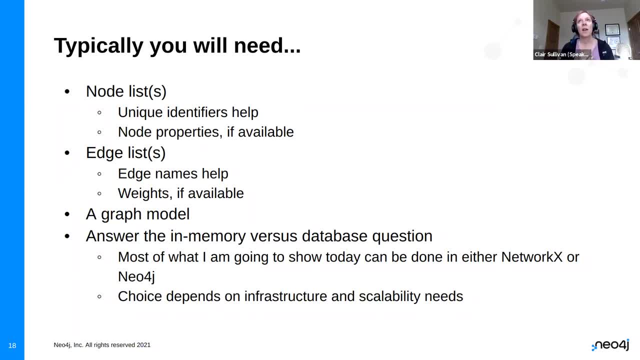 package in graphs or in Python called NetworkX. A lot of people start with NetworkX. There's several different types of graph databases, such as Neo4j. I'm going to be using a database today. I personally prefer databases because they scale better, But this is again a choice that depends. 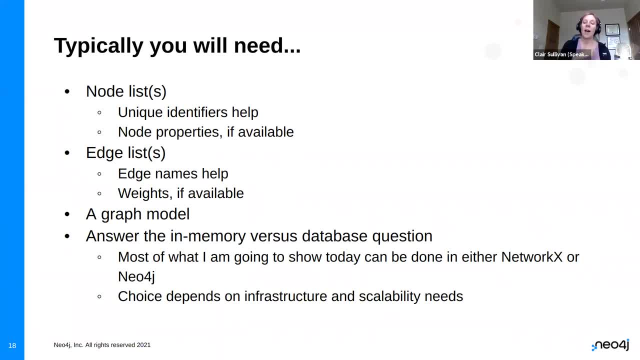 on your infrastructure. This functionality that you have in NetworkX you also have within Neo4j. I'm going to show you. I'm going to use Neo4j because one of the reasons is because there's a nice visualization tool So you can see what the graph looks like. There's more intuition that will 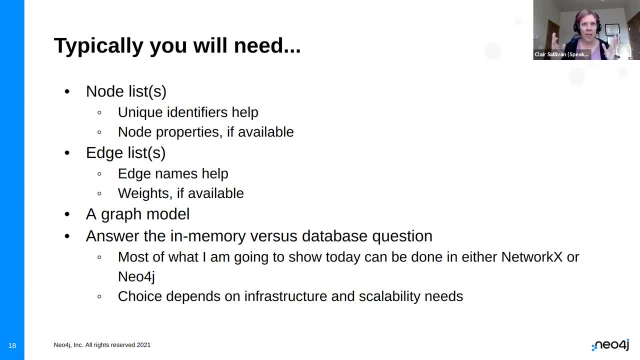 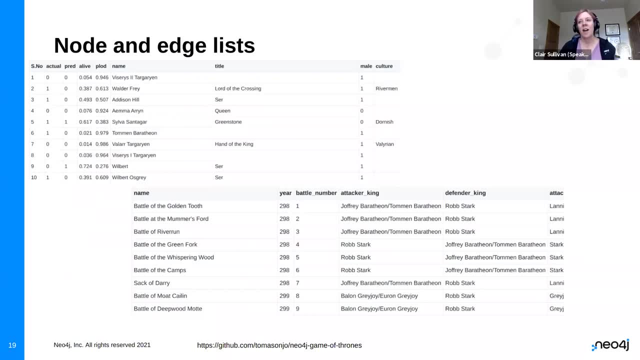 come from just being able to see a graph, But again, the choice is yours. Okay, So this is just an example of node lists and edge lists, And one of the starter problems that a lot of people use is Game of Thrones. Now I'm going to throw out there. there's Game of Thrones spoilers here, So 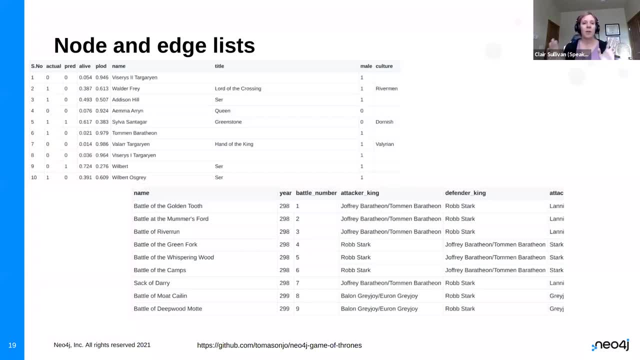 you know, if that's going to be a problem, I'm going to throw out there. there's Game of Thrones, It's going to bother you. It might be a good idea to log off, catch up on Game of Thrones and then. 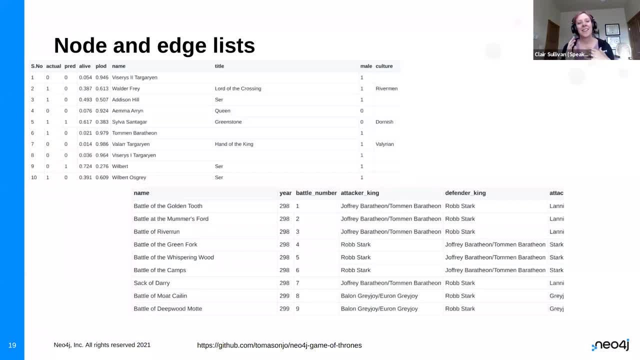 you can watch the video. But in all seriousness, Game of Thrones books one through five. somebody went through all of the books and started looking at who had what relationships with whom within these, who appeared in which books. So the node list is what you see on the upper left And you 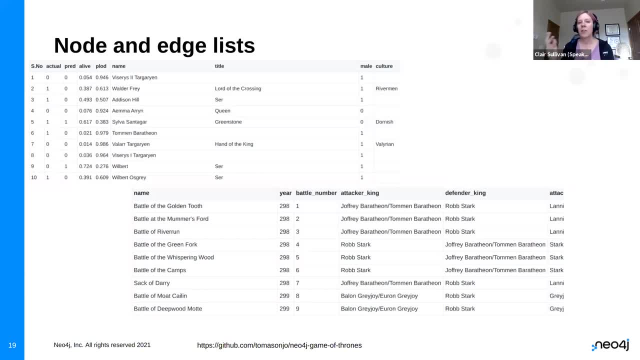 can see. it's got names and titles, male or female, cultures, things like this, And then on the lower right we have the edge list, And then on the upper left we have the edge list, And then on the upper left we have the edge list. So we can see- and this is actually cut off a bit, but we can see- 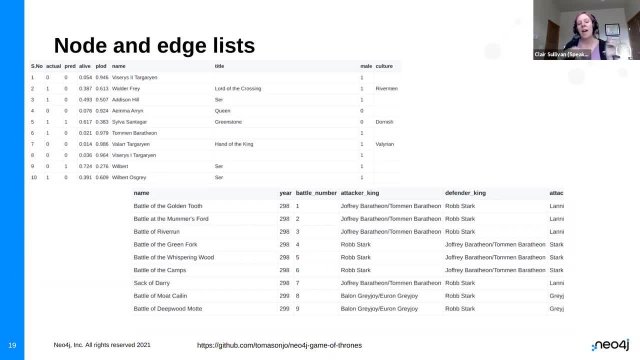 the name of the. there's a battle here, And so I have the name of the battle. When did it occur? Who was attacking whom? Who was defending? So this is the general idea. You're going to have to have these things ready to go. if you're going to start doing graph stuff, You'll note at the bottom of: 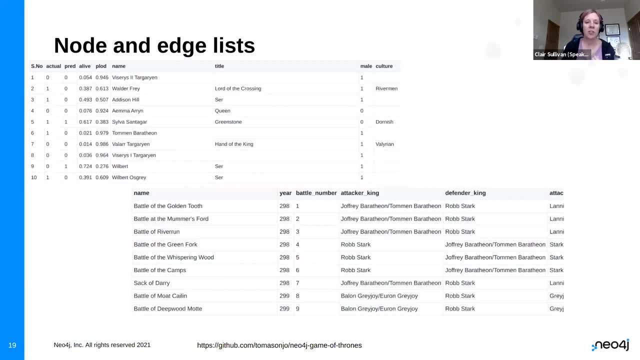 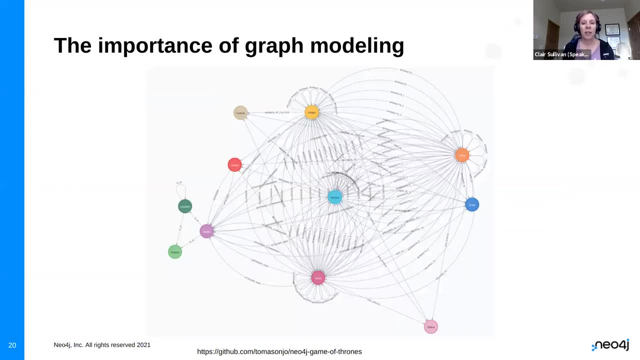 the slide. there's a GitHub repo that gives you this data. I'll also show how you can automatically get it within Neo4j. Okay, Graph modeling. Now I'm not expecting you to be able to read this text here, but it's very important, as you start setting up your graphs, to understand what nodes are going to. 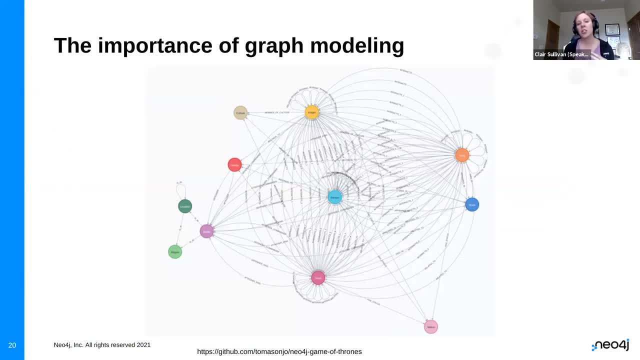 have what kind of relationships with what other nodes, And in my view, the best way to do this is to sit down with a whiteboard and start connecting things. So at the very center, even though it's kind of hard to see, here is that kind of cyan color node and it's got the 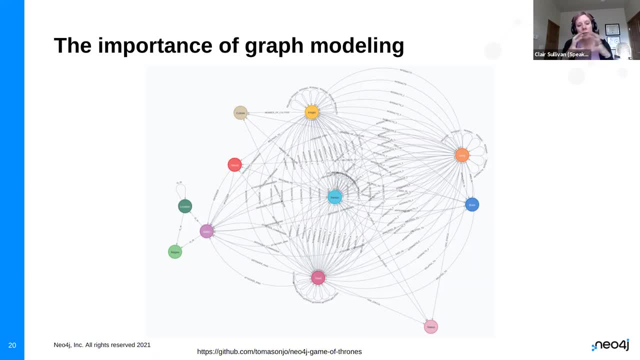 label of person. So people are going to be labeled as this cyan color. I've got dead people which are kind of 630 on this chart. I've got battles- Those are purple. I've got houses in red. Houses are kind of like at about 10 o'clock. I've got knights. 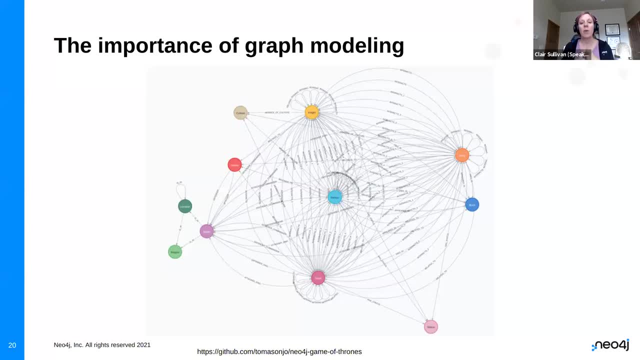 and kings and all of this stuff. Now, you'll notice, though, I have people, knights and kings, And you could have one person with multiple labels, and that's totally fine, totally allowed. And then I have my relationships between them. I've got interacts with 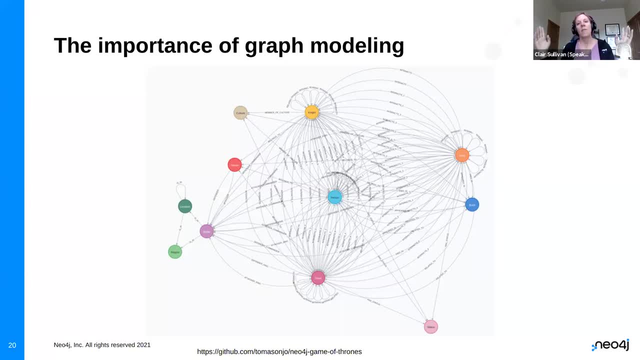 this is broken down into just kind of an overall: interacts with versus interacts in this book, interacts in that book, interacts in another book. We have belonging to house. We've got a whole bunch of different kinds of relationships here And it's always a good idea to try and filter. 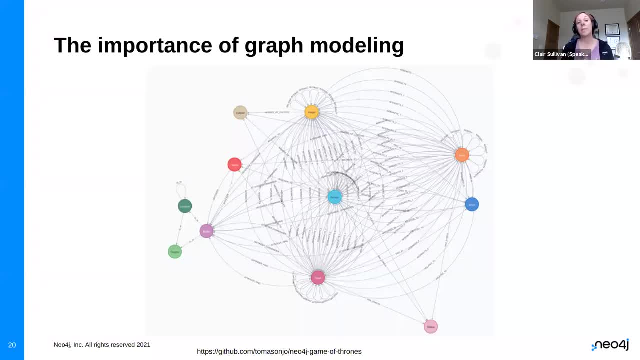 on these things as much as you can, Because when you start dealing with really big graphs- by really big graphs I'm talking about billions of nodes, I'm talking about tens to hundreds of billions of relationships- It really matters that you can filter through that. 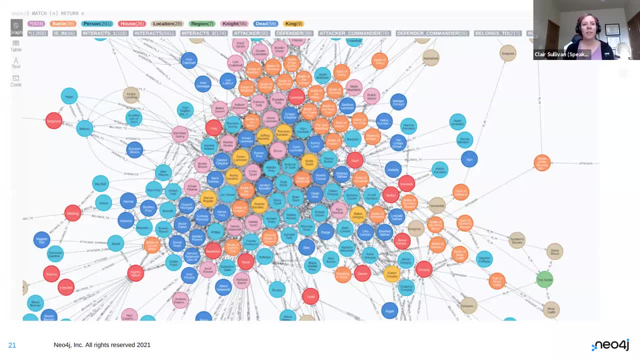 Effectively Okay. So just really quick. this is what our graph is going to look like, And in just a second I'll show you some code behind how you can create this graph, if you want. We see people. We see this really dense cluster here, Not quite in the center, but slightly off. 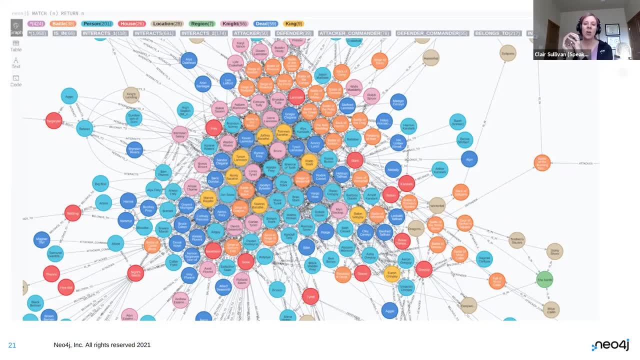 to the right just like an inch. There's this red node. It's called Stark. So that's the house, Stark. We've got Freys and Lannisters, We've got all kinds of people here. This is how your graph, as much as I, could get onto the screen. there's actually like 2,400 nodes, and 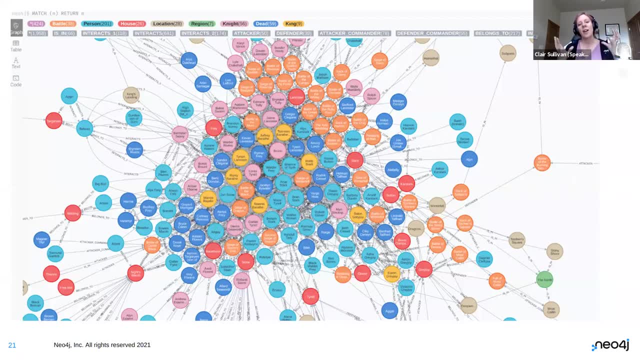 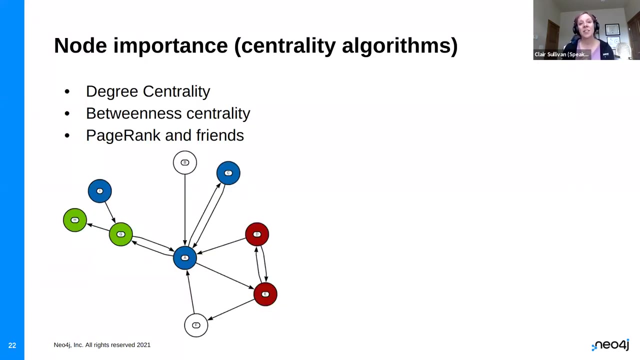 16,000 edges or something like this in this graph. So your visualization. it starts looking like a cat's hairball. So it also helps with visualization if you can narrow down what you're looking for. Visualizing graphs is an art in and of itself. Okay, What can we calculate this? Well, there's. 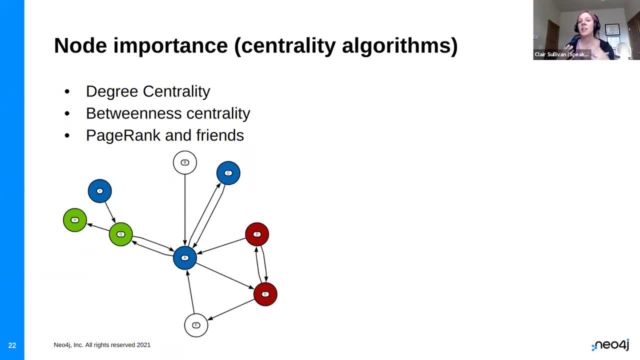 a whole bunch of things that we could look at. We could look at node importance or centrality algorithms. Which node is the most important? Which node is the most important? Which node is the most important? Which nodes matter more to us? Obviously, there are characters within Game of Thrones. 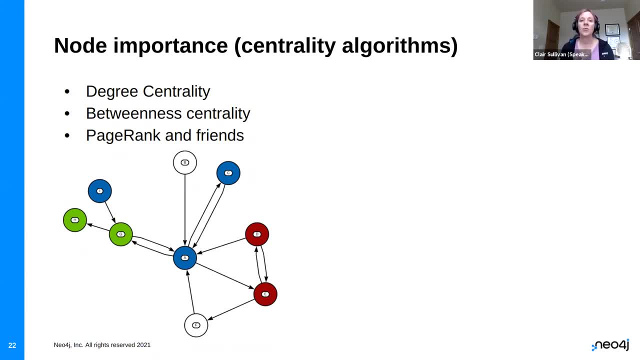 that are more important than other characters. There's several different ways we can measure this. This functionality exists just as functions you can call in Network X, in Neo4j, Degree centrality. Let's start with that. Degree centrality means how many, it's just degree. 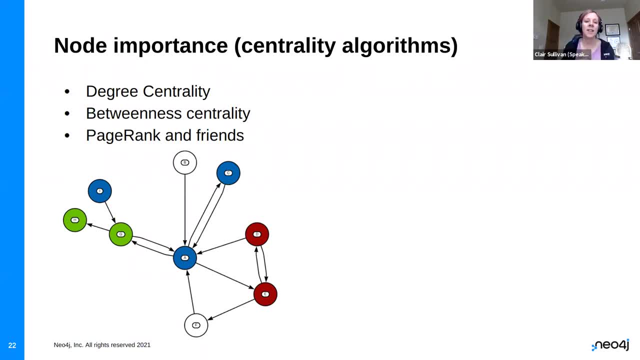 which nodes have the highest degree. So in this sample graph, A has the highest degree because it's got a whole bunch of arrows coming in and out Betweenness centrality. I love betweenness centrality. It's a lot of relationships with A. It doesn't mean that A is the most important. 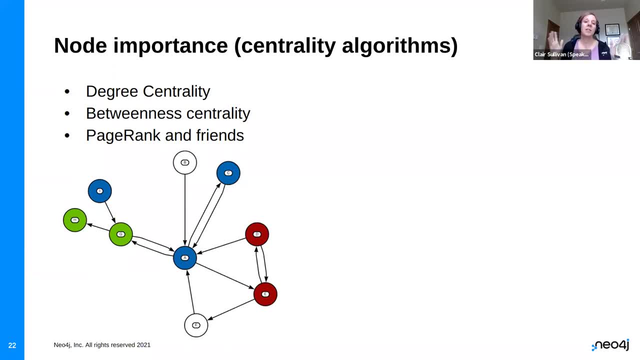 person. Think about an office and you've got the big boss And the big boss. you know there's a lot of people who want to talk with the big boss, But do you want anyone? do you want everyone to be able to reach out to the big boss and get a meeting? And the answer is no. They have to go. 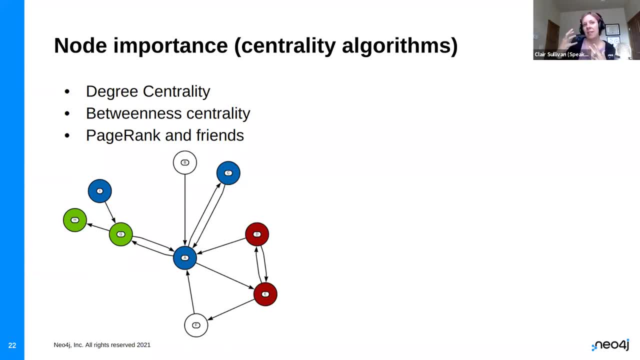 through the big boss's admin. Now, the admin may not be the thing, the person with the highest page rank, as we'll discuss in a minute. The admin just might have the highest degree centrality, or what we call betweenness centrality. The admin is who you go through. 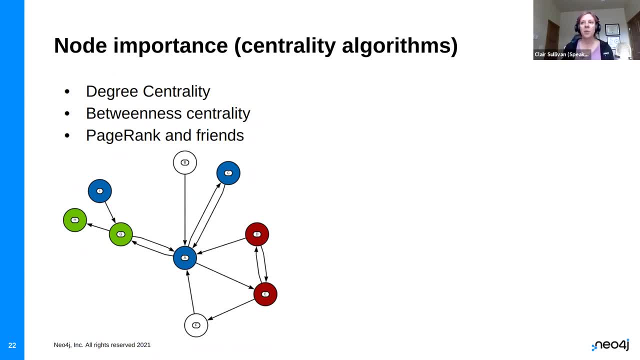 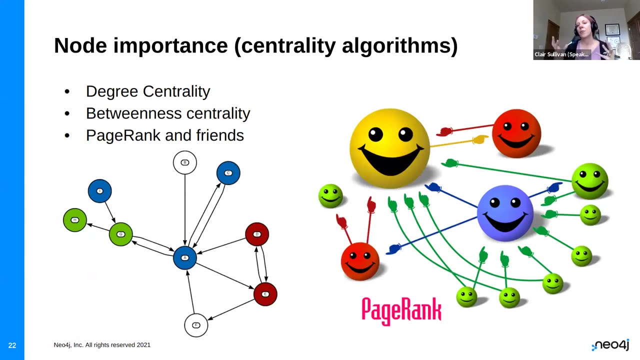 to get to that important node. I was asked: please could you mention the alternative to network X again? And yes, it's called Neo4j And I will show examples with Neo4j coming up here in just a minute. Okay, So page rank. we're all familiar with page rank. Larry Page, who you 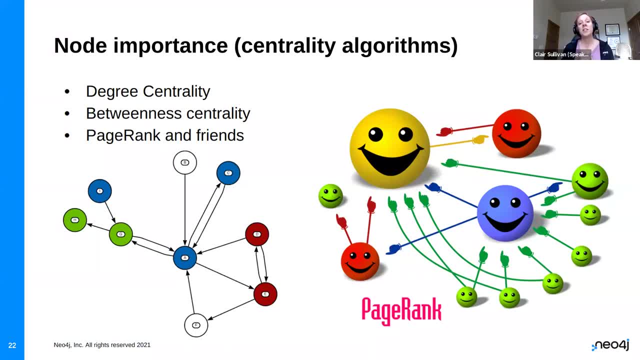 know one of the core people within the original Google invented page rank, And what it does is it looks at how many links are coming into a web page versus how many are going out, And you can see here my nodes are colored based on their page rank. So the larger nodes are colored with. 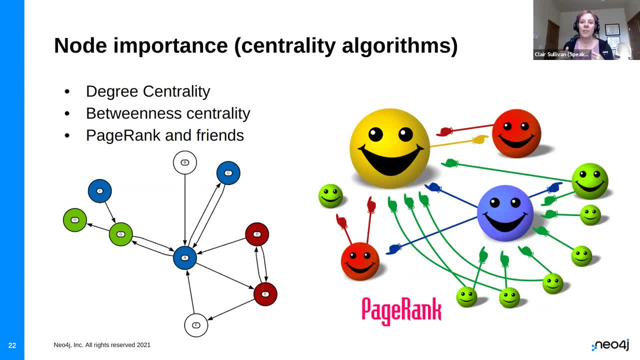 or the larger nodes have a higher page rank. So I can see, for instance, my blue node has kind of a medium page rank And that's because of a lot of things. a lot of web pages link into it. Maybe they're not very important web pages, but there's a lot of them. But then I see a lot of web. 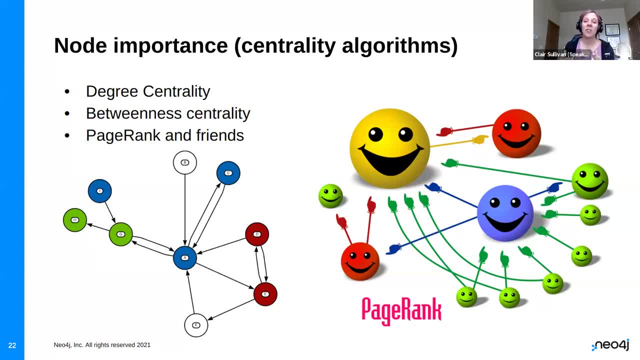 pages are linking in, only in, to that yellow node. The yellow node has only one link out. So the fact that everybody's referring to that yellow node means that the yellow node has the highest page rank here. But you see that red node on the top right, that's actually got a bigger page rank. 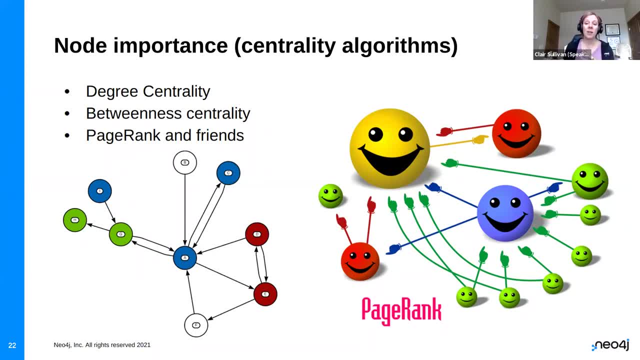 than some of these other nodes. It's got a proportionately larger page rank than that blue node if it had more links to it, But it's bigger because that's the only thing that yellow node with the highest page rank links to. So that's how we do. 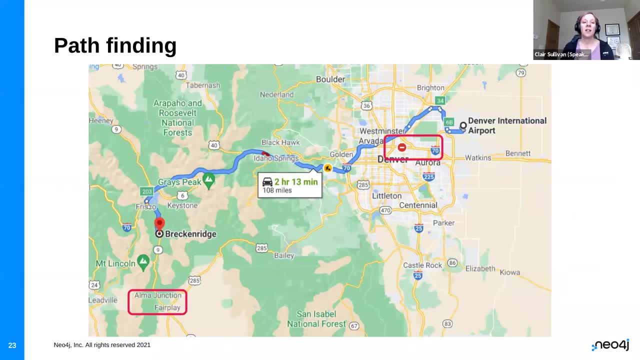 Pathfinding- another great thing that we can do in graphs. There's a ton of pathfinding algorithms out there. Pathfinding- that's an art unto itself, But here I'm showing my path between Breckenridge, where I live, and the Denver International Airport. Now Google is able to tell me how. 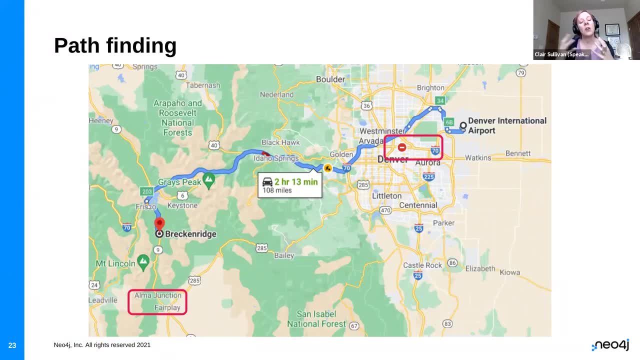 what's the fastest way to get there? through pathfinding, because it knows how to weight each of the nodes on the path. So those nodes are given by the little white circles. okay, Now you'll see a couple things here. There's two different ways I could get to the Denver. 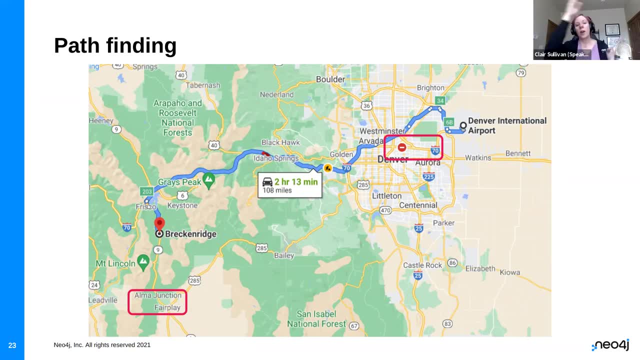 International Airport. I could go the loop up top or I could go the loop on the bottom through. that highlighted Alma and Fairplay. So why did Google route me this way? Because I'll tell you this isn't actually the fastest route. You can see that there's that red box in the kind of upper. 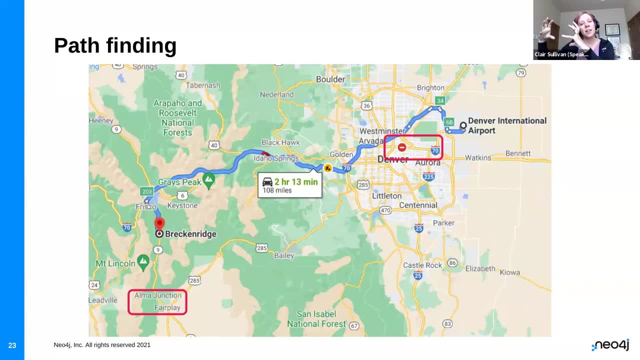 right section. That's actually usually the fastest way to get to Denver International Airport, But the problem is it's closed And Google knows it, And so Google routed me up and around Now. the other thing I'll tell you was that I created this graph during the middle of the week, Because I live in a resort town. 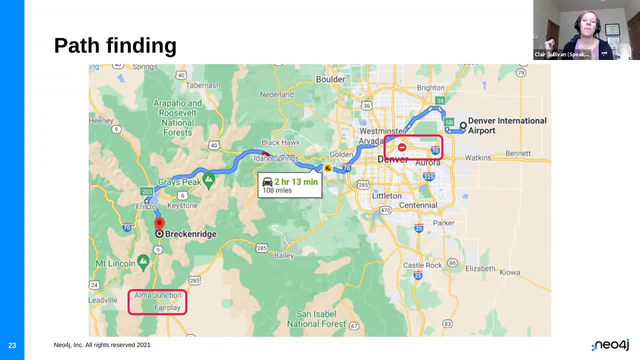 everybody's coming up here on the weekends and everybody's going back home at the end of the weekend, And so sometimes what you'll see is that the fastest route is actually to go down through Alma and Fairplay. So that's just Google understanding real-time pathfinding with a. 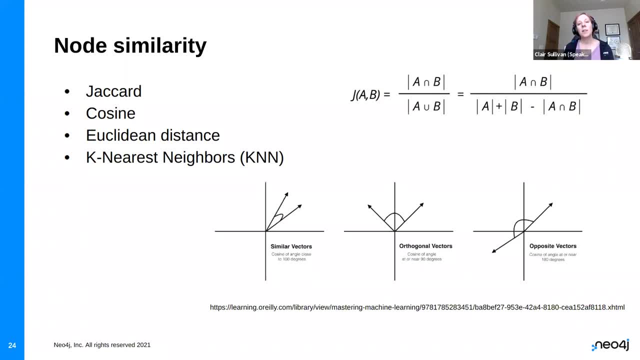 weighted graph. So node similarity is another thing that we can do. Now this typically requires us turning nodes into vectors, And I'm going to show you how to do that in a minute. It's a super fascinating thing. So node similarity we can think of. we've got embeddings and how do we compare them? Well, we can look at. 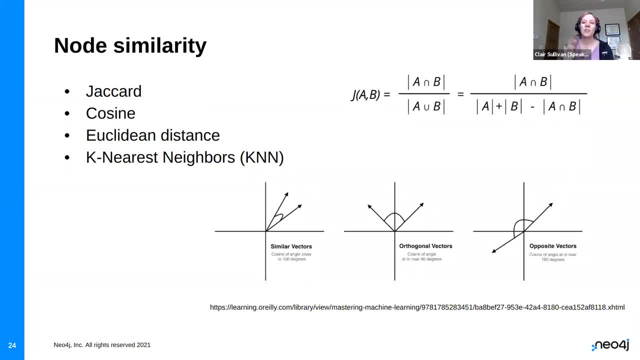 Jaccard similarity. How many nodes do two nodes have in common? And that's given by the upper right on the slide. But then we can think about all kinds of distance metrics like cosine similarity, Euclidean distance. We can look at K nearest neighbors, particularly in an unsupervised context, And that's all. 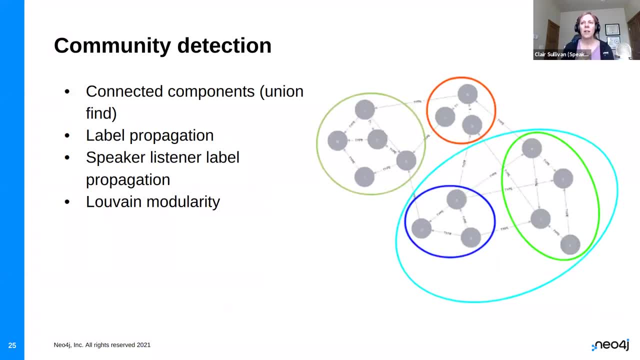 possible within a graph. And then I think this is the last thing I wanted to mention, but before we get into some actual code, here is community detection. Actually, I think I'm going to talk about embeddings first, But community detection- How do I find my people? How do I find my people? 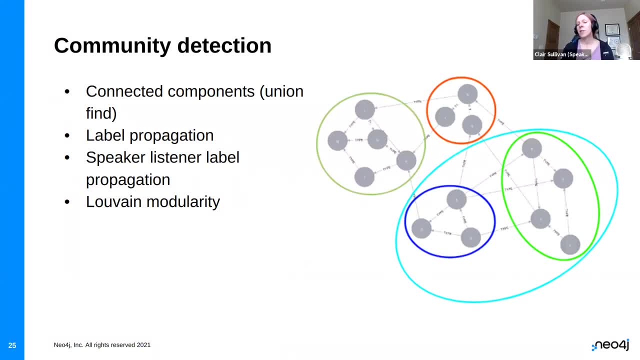 within a social network Or you know. there's a lot of work showing how different politicians vote with each other And, like in the United States, it's pretty easy using community detection to separate out Republicans and Democrats. So we could detect whole communities. We can detect. 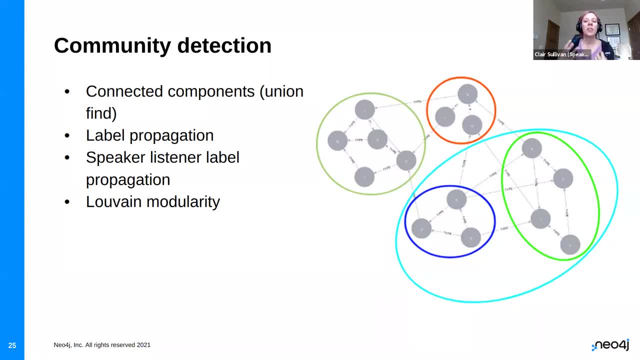 sub-communities. So sub-communities would be things like the blue and the green circle, with the whole community being the cyan circle. There's a whole bunch of different ways to do this. They're listed here: NetworkX does it, Neo4j does it. I'll show you in Neo4j how to do it. 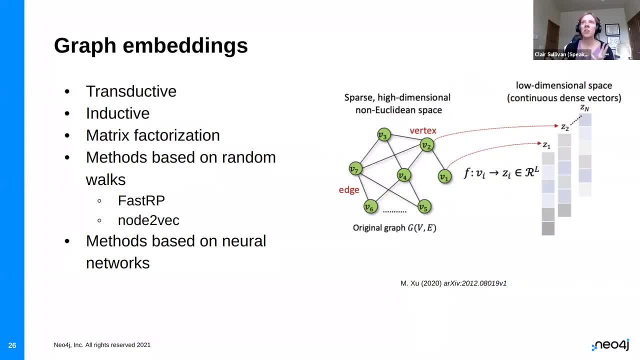 And then the last thing is graph embeddings. Graph embeddings: there's a whole ton of ways that you can convert a graph to a vector, But they tend to fall into two categories: transduceive or inductive. Transduceive means I take the whole graph. 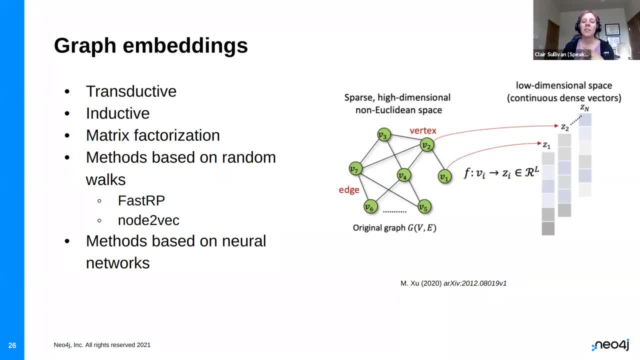 and I train on that and I create vectors around that. Inductive means I can take my graph and I can update those. as a new node comes in, I can provide an automatic vector to it without having to train the whole graph. Benefit is obvious that I can handle new data as it comes in. The drawback: 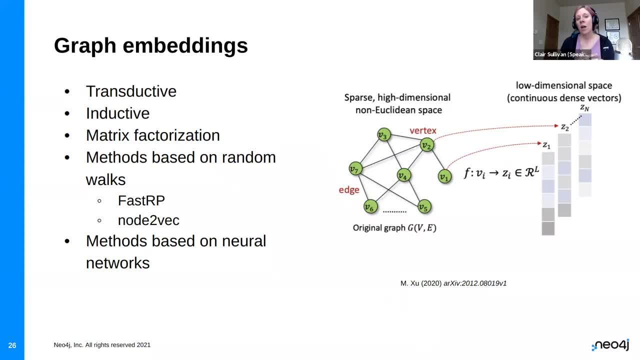 is inductive. I can handle new data as it comes in. I can handle new data as it comes in. Transduceive mechanisms tend to take a lot more time. We could break these down further. Matrix factorization: I showed you that adjacency matrix earlier. Great for doing math on smaller. 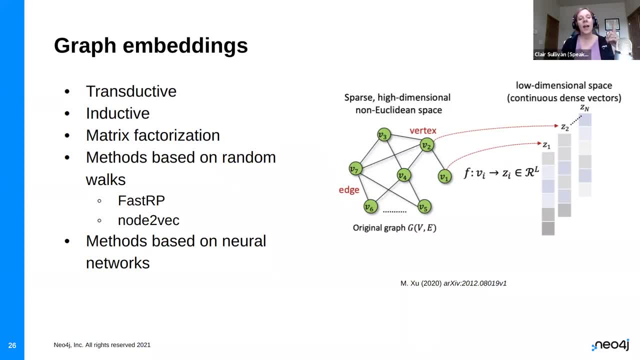 graphs. But if you consider the fact that every node has a row or a column, that's an order node squared problem- Not our favorite thing to do- So they don't scale well. Then we have all kinds of different embedding methods based on random walks. Now, if you think about those of 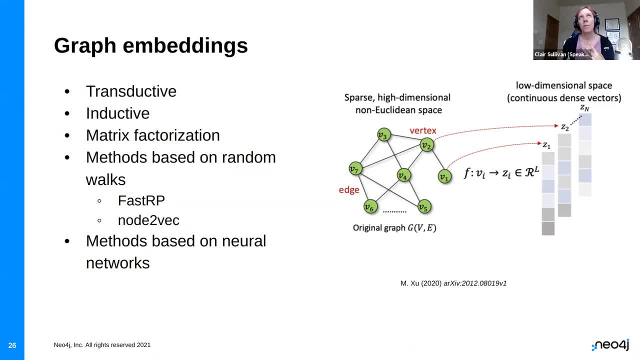 who've done some NLP before you might be familiar with word devec, where we do this skipping around a sentence and moving these little skip grams across the sentence. Great thing. And there is an equivalent within graphs called node devec. Node devec does similar skipping around, but there's 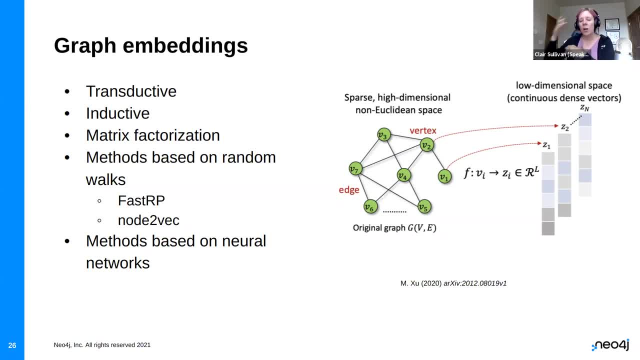 no sequence of things like words. So generally, what you're doing is you're doing random walks around a graph to try and say, okay, I walked, I did 10 walks, 10 hops, 10 times. So you know my vector is going to be based on what nodes did I hit along the way And then 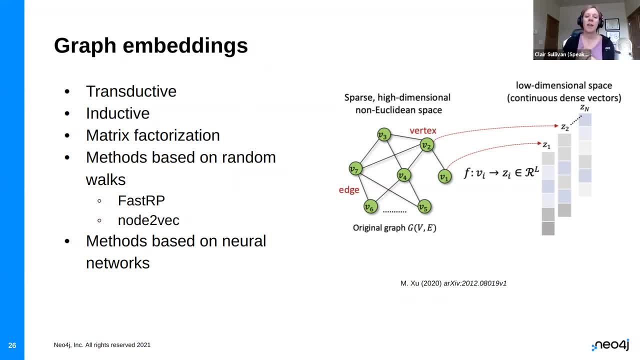 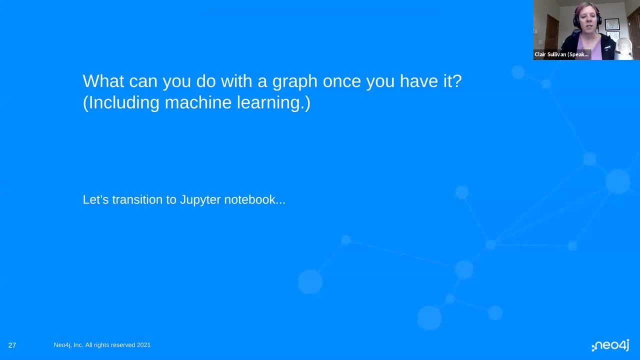 of course, everybody asks about deep learning. There are definitely methods based on neural networks: graph convolutional networks, graph neural networks. There's tons of them out there. Okay, Let's, okay, Let's, we're going to transition. now I'm going to go over. 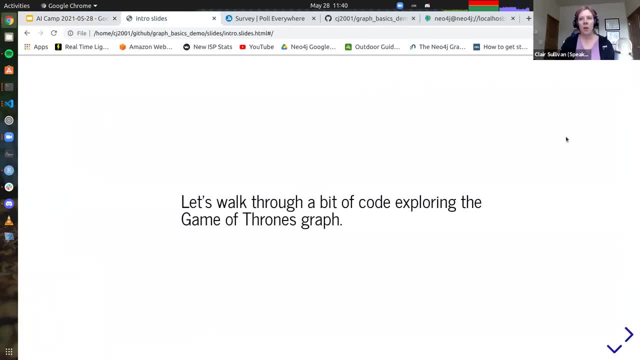 I've prepared a Jupyter notebook to kind of look at this stuff. So what we're going to do is we're going to just go through a bit of code exploring that Game of Thrones graph. Now, if you go get the slides- there's discussions here about how to set up. 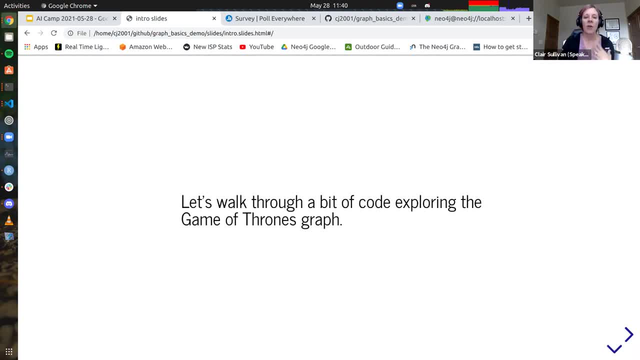 your connection to Neo4j. I'm not going to spend a lot of time on that right now, But it's in. it's in that Jupyter notebook using the official Python driver for Neo4j. And again, just think of Neo4j as a database. I could be giving a similar talk on SQL, or you know. 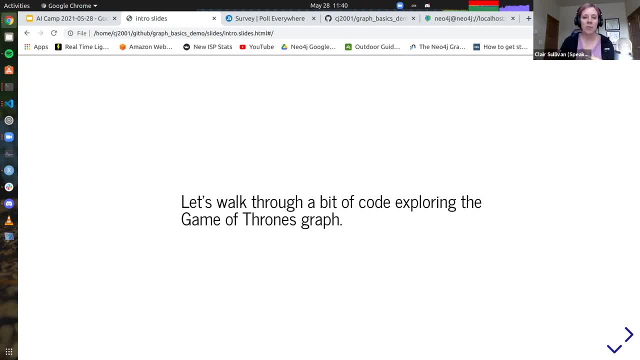 any other database that we might be interested in. It's just going to be a database for us. Okay, Let's do some data science Now. I told you before that it's usually a good idea to break your graph down into the bits that you care about. Okay, So, because otherwise? 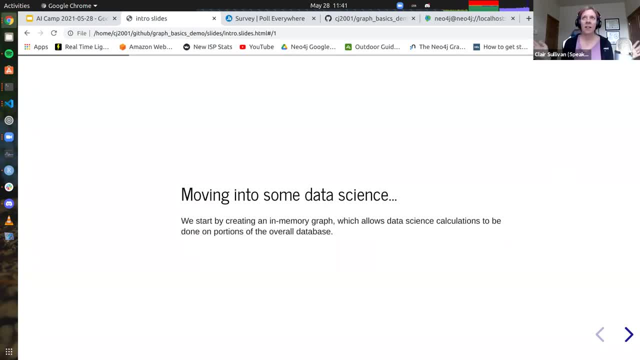 if you're dealing with a super huge graph, you don't want to calculate everything on it. You're going to, you're going to crash your system. It's just going to be too much as that graph gets big. So we're going to come up with, we're going to narrow down our graph into, say, people, Okay, So. 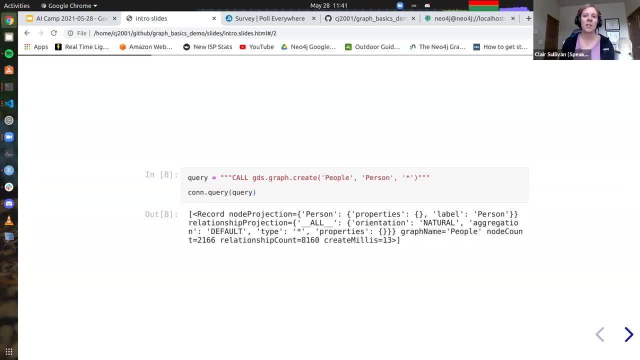 I have a query. Now you'll recognize this. It has- it has very similar context to a lot of Python vectors, to different SQL databases. So here I've specified a string that's called a query and we're going to be using this thing, GDS, which is called the graph data science library. It's 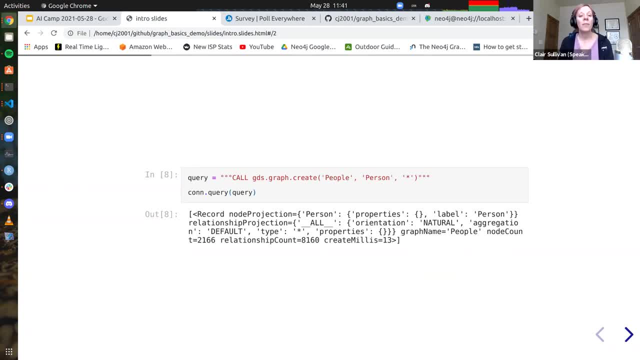 what's built into Neo4j to do all of our fun stuff. Like I said, there is an equivalent to network X, but we're just going to go straight into the fun stuff. Okay, So, GDS, we're going to create this graph and the name of the graph is going to be called people. Okay, So we're going. 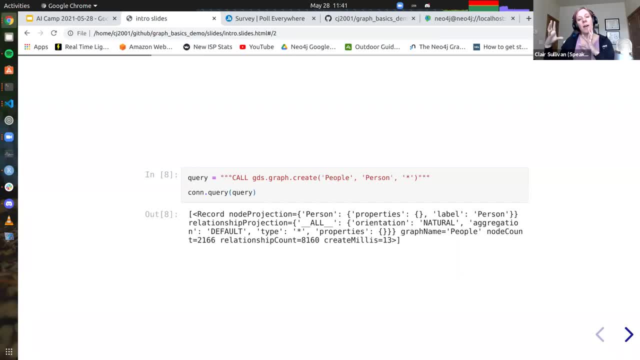 to have all people in the graph. That second thing is specifying which nodes we want. So I want all nodes. And then after that the third entry. there is: what edges, what relationships do I want? I'm just going to say I want all of them And I'm going to run a query and I can see that I have. 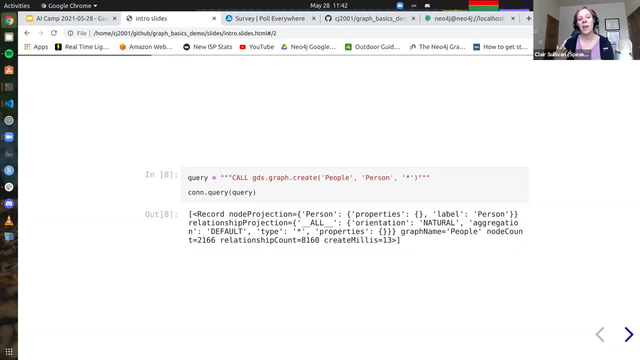 if you look at the last line here, I've got a node count, So I have 2,166 nodes and 8,160 relationships. that came out of this graph. Okay, cool, So let's do some calculations on that. Let's calculate page rank. Okay, So we're going to look across all people in this graph. 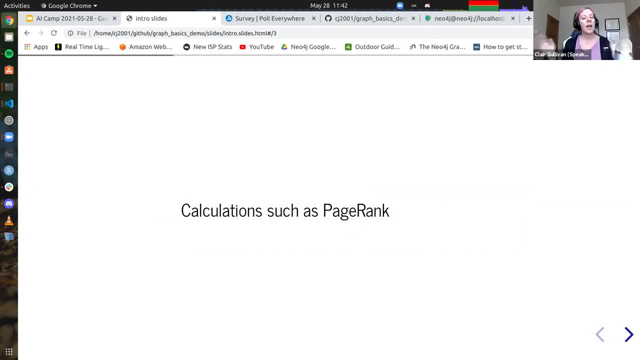 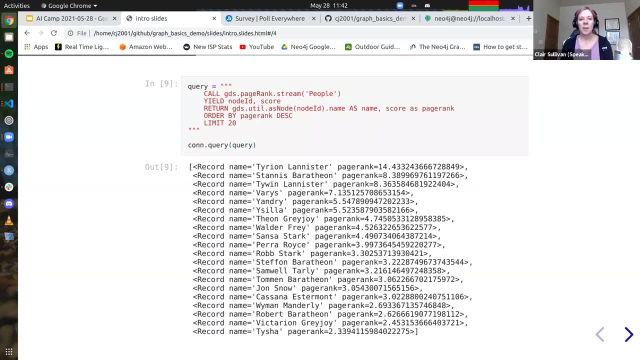 across all every relationship that they might have. We're going to find who are the most important people, Okay, Based on page rank. there's all kinds of other things, Okay, So some of these names make sense here: Terry and Lannister, Stannis, Tywin, Lannister Varys, but now I'm 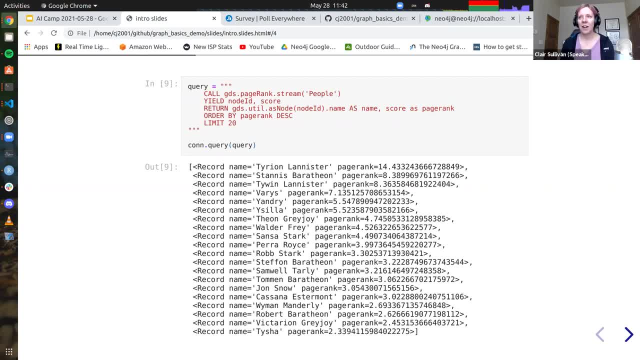 starting to get into some names. I don't know who Yandri or Ysilla are, or anything like that. So you know, I'm just going to say I'm not getting, I'm not buying these results. Well, the reason I'm not 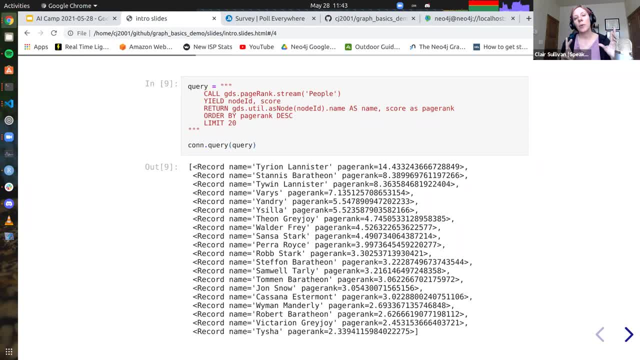 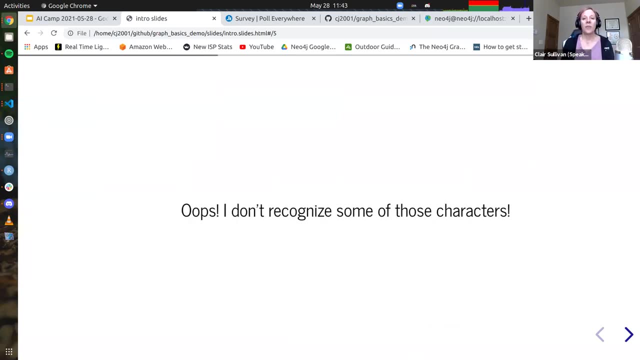 buying these results is because we specified every single relationship was going to be part of this graph called people. Okay, Not the best way to go. Really, I am only caring about which people interact with which others. So yeah, oops, I don't recognize some of those characters. So 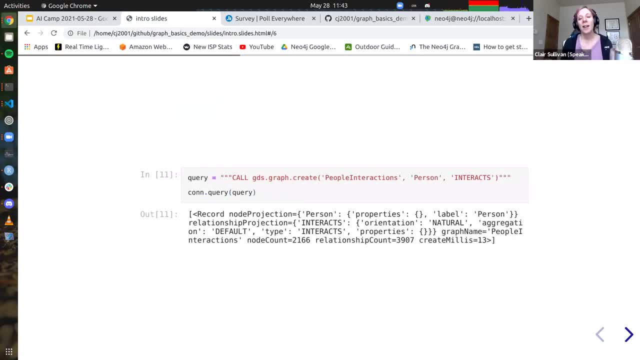 let's make this a little bit more refined. I'm going to create a new graph and it's going to be called people interactions. And now I'm going to look at node types called person and only the relationships called people. So I'm going to create a new graph and it's going to be called: 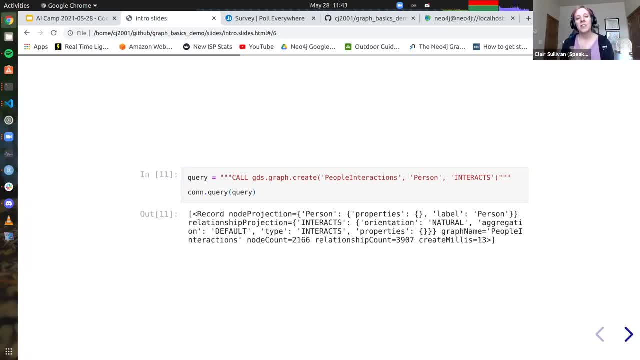 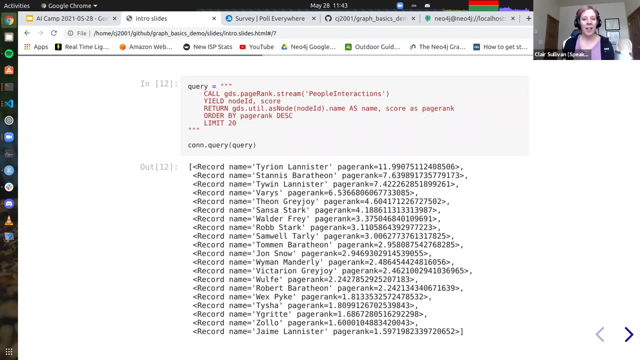 interacts. Now I could break this down by season two, but you can see my relationship count went down. I have 3,907 relationships that we just created this in-memory graph on. Okay, Now I'm going to run page rank on that. Now my list starts making more sense here. I recognize most of the 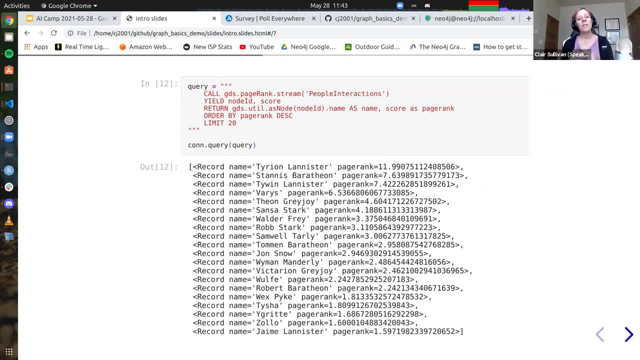 names on this list until I start getting a little lower here. So I'm starting to feel better about this calculation here And I should tell you: any algorithm you're going to run on a graph for data has a whole whole ton of special knobs that you can turn. Okay, There are hyperparameters upon 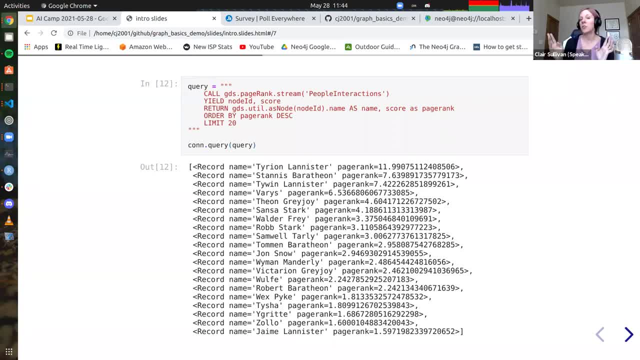 hyperparameters in these things. Right now I'm just showing default hyperparameters, but you know definitely, whatever way you want to run the graph is you know whether it's a network X, whether it's a Neo4j, whether it's in something else. you definitely need to spend some time on. 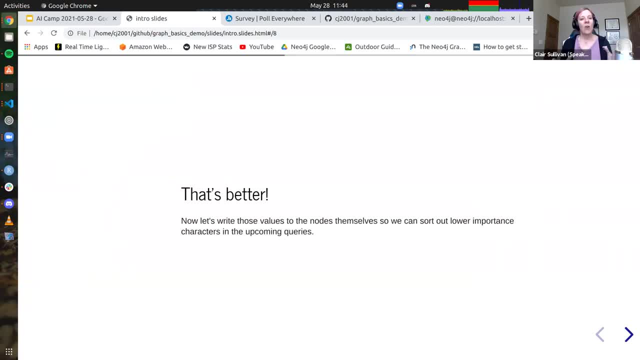 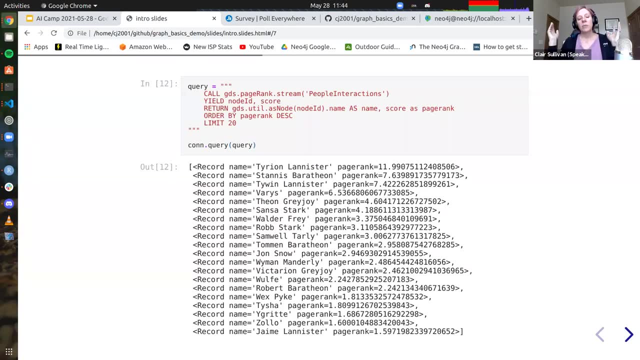 those hyperparameters. Okay, cool, Now I've got these page rank things. like you could see here, page rank equals, you know. whatever it equals That, just output it to the screen. But you know, someday I'm probably 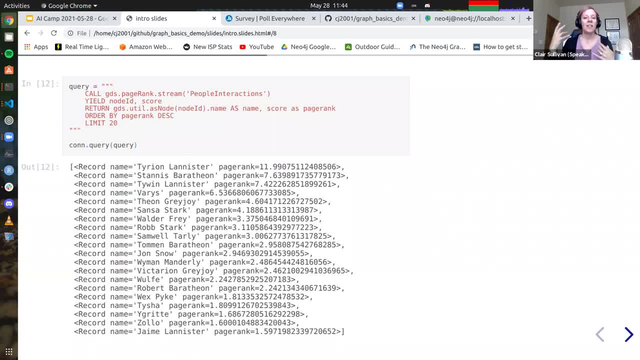 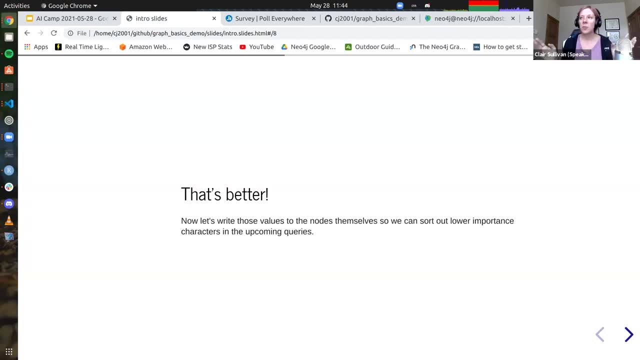 going to want to use that information somewhere other than just having it sitting there in my head. So what we can do is we can write that value to the nodes themselves, because I'll tell you we're going to do some calculations coming up here And you know I don't want to sift through. 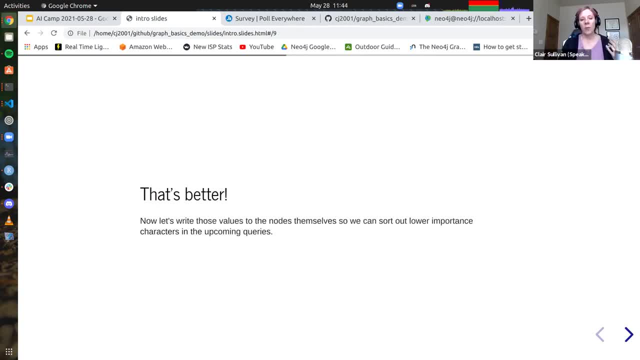 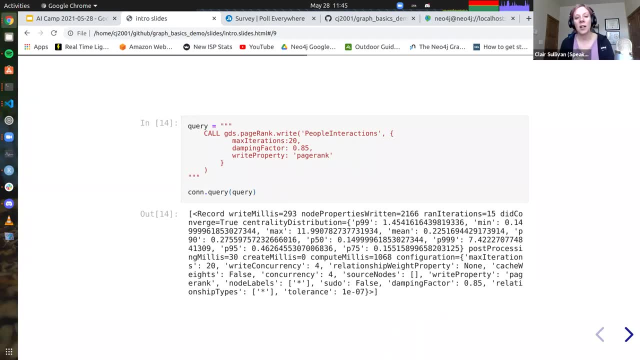 all of these names that I've never heard of before. So we're going to write it to the graph. It's just this page rank dot write, so we can write over all of these things again, And then we're going to do some hyperparameters. 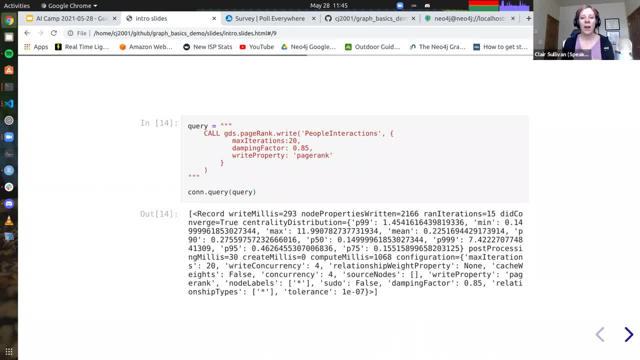 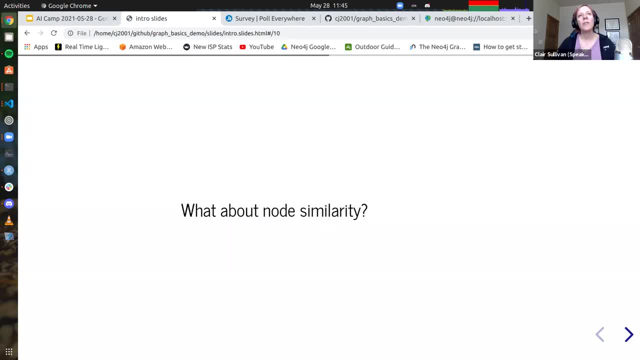 So I've got the top here. This is the top edge of the node, And then we've got the top edge, and you know, we've got the top edge of the graph. That's right. here is a little bit more of the thing, But now we're going to go over and we're going to do some linear regression. You can. 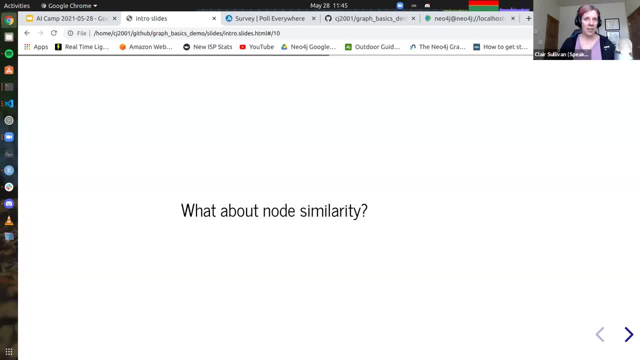 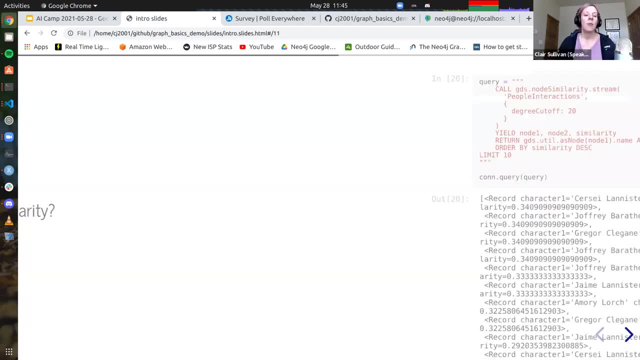 see a few hyperparameters here. That's all well and good. You get some information about how that right went. You know how long it took and how many records were written. Okay, cool, which is given by that. call GDS node similarity stream. Stream means go to the screen. 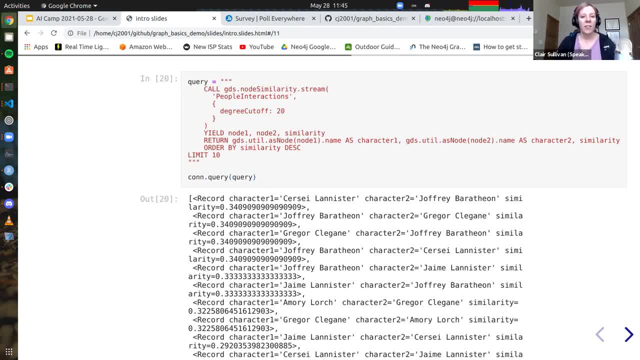 And I'm just going to return who's most similar to who. So at the very top I see that Cersei Lannister and Joffrey Baratheon have a high similarity. Makes sense if you know the story. And then I see Joffrey Baratheon and Gregor Clegane. It's repeated there They have 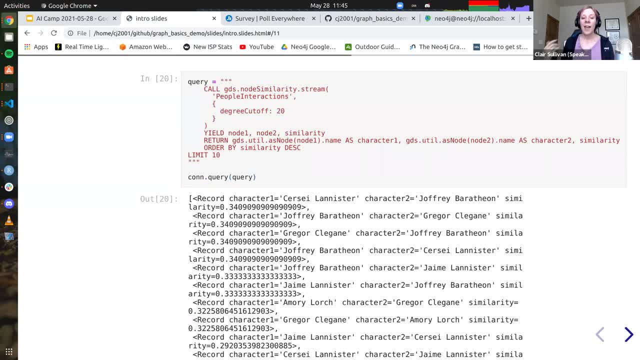 you can get rid of duplicates in here if you want. But you know, again, that makes sense. It's Jamie Lannister Joffrey Baratheon, Jamie Lannister Cersei. Again, all of that makes some. 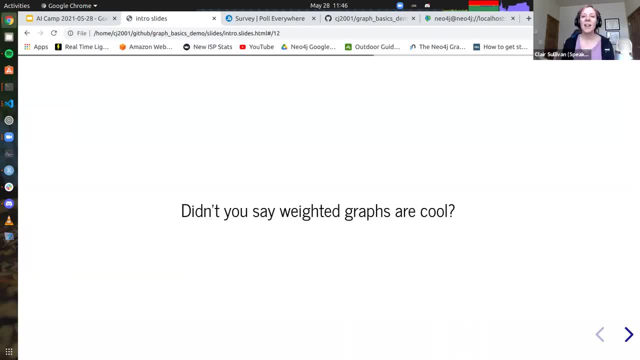 sense here. Okay, But didn't I say that weighted graphs were cool? If you can create a weighted graph, awesome, Always do it. So I haven't created a weighted graph right now, but there's actually weights within this data, So we're going to create a new in-memory graph. Okay, This looks a little. 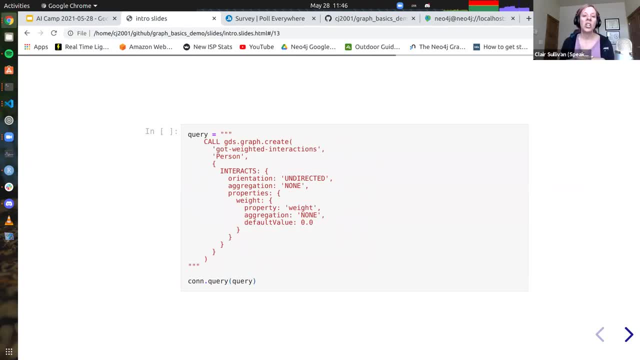 more complicated. Don't worry, It's not that bad. It's going to be called GOT- weighted interaction. So again, we're looking at people interacting with other people. But if you get in and you look at the actual properties of those relationships, there is a property called 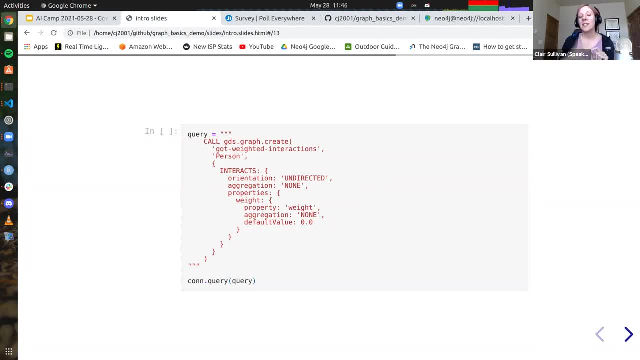 weight in there. Okay, So we're going to use that weight. We're going to tell it there's a default value because, you know, sometimes, as we all know as data scientists, 90% of the job is being a data janitor. Okay, We have to clean our data. clean our data, clean our data. So. 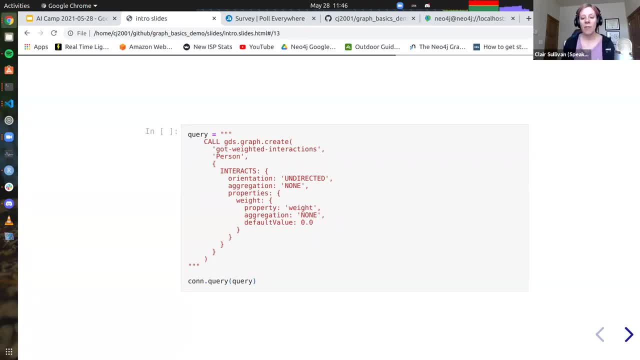 not all of these edges have weights, So we want to give a default value wherever we can. Okay, So now we're going to do, we're going to detect some communities based on that weighted graph. Again, community detection is one of those that really can benefit by using the weights. 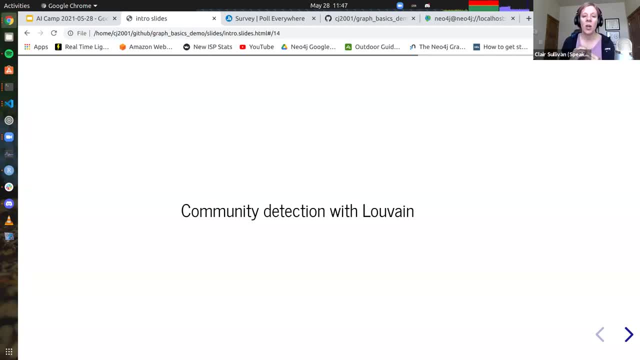 which relationships are more important than which other relationships. So we're going to use what we call Louvain community detection, And it's a mathematical thing. I don't have time to go through the math on it. There's plenty of resources out there. Wikipedia is your friend on this one. 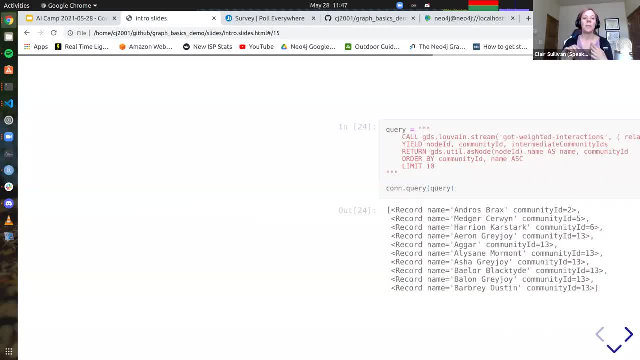 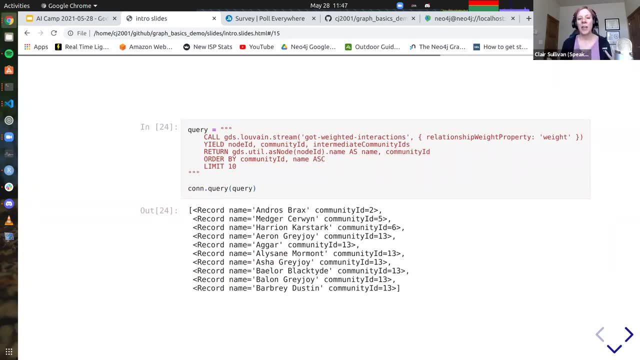 But let's just do Louvain community detection. It's probably one of the most common types And we're just going to stream to the screen what the what, the detected communities are. And again you know- I'm getting names here- that I don't really know that well I can see, you know. 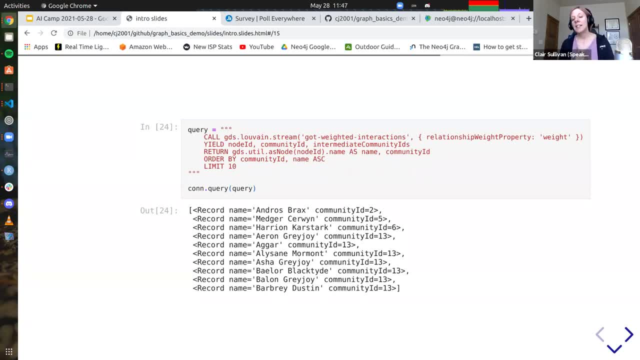 you're going to get this integer for your community ID, And I can see in here that community ID 13 has Asha Greyjoy and Bailon Greyjoy. Okay, That kind of makes sense, I don't know. Oh, Aaron Greyjoy. 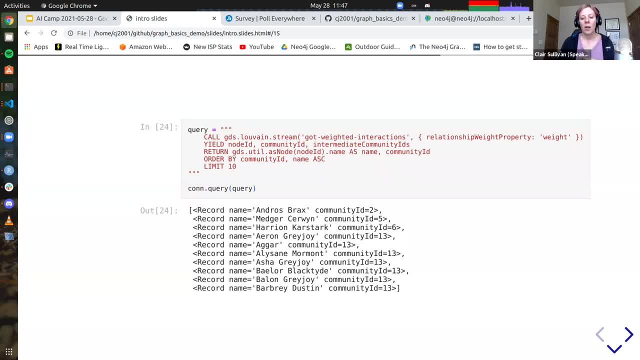 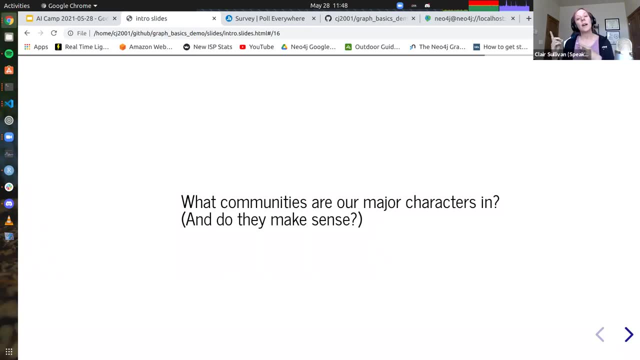 Okay, I got Greyjoys in community 13.. All right, let's let's try to look at who the major characters are and what communities that they're in. So this is where it mattered that I wrote the page rank to the nodes, because 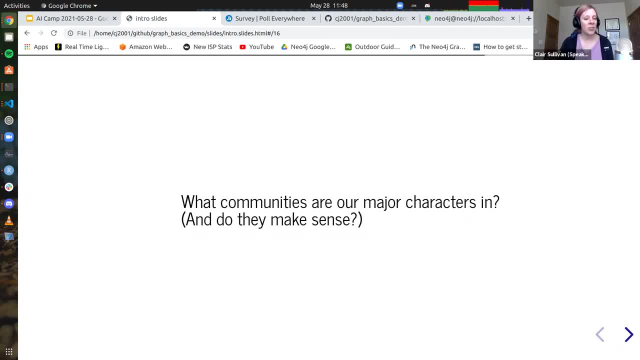 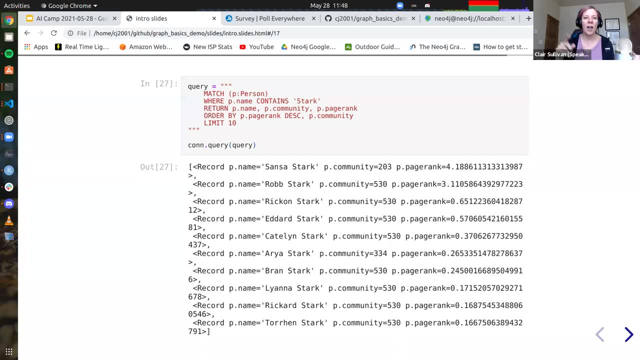 I'm going to start by page rank here And let's, let's just see what we get. We're going to do this again. same community detection here we've got. we've created this query up here which is in a 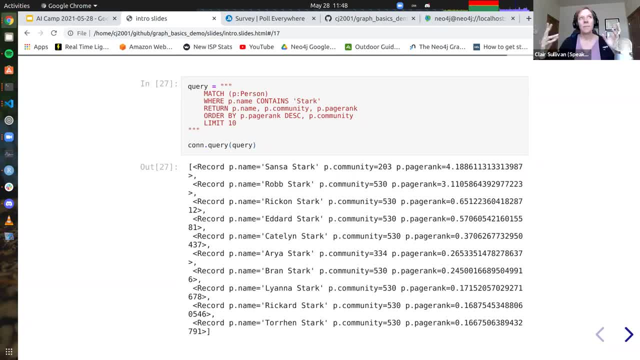 two SQL, you'll find. you'll find that there's. you do these ASCII art things So like the round parentheses mean a node. I can get square brackets. that means an edge, but whatever, Here are people sorted by their communities and their page ranks, So I can see that I've got a. 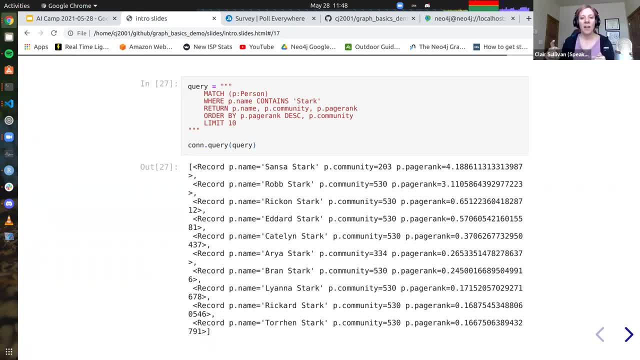 bunch of Starks- Rob Rickon, Eddard Catlin- and they are all in the same community, but Sansa Stark isn't, And that's probably because, as we remember from the book, she leaves those guys in the first book, So she's off doing her own thing. And then I've got Arya. 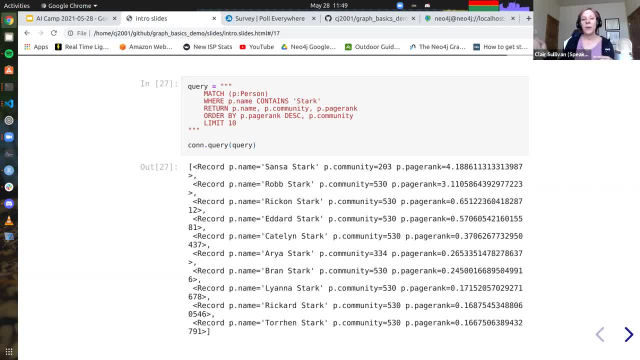 Stark here, who has a different community, But again she left, she's off doing her own thing gallivanting around the countryside. So these communities make sense when you, when you look at how they came out. And again, I sorted this by page rank just to make it easier to understand. 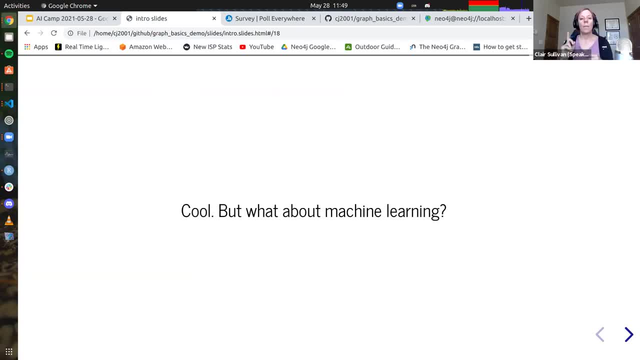 Okay, Okay, Cool. But what about machine learning? Now, frequently when we have a graph- not all the time, but frequently- we're going to have a graph that says, okay, I'm going to do this. We're talking about an unsupervised learning problem. We could get lucky. I could you know? 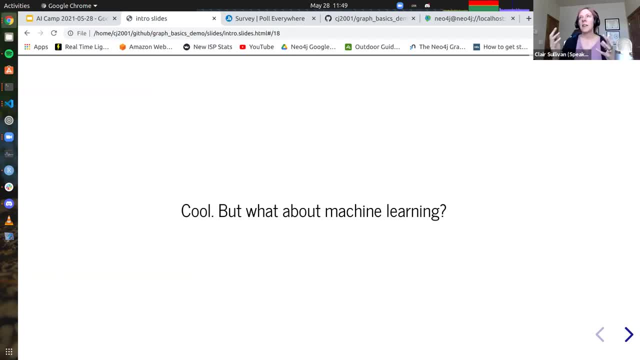 I could have run this saying: you know, of all these characters, Stark versus not a Stark, Or you know in persons, in the North or not in the North. Okay, But for the sake of today, because we don't have a lot more time, I'm going to show you just some quick. 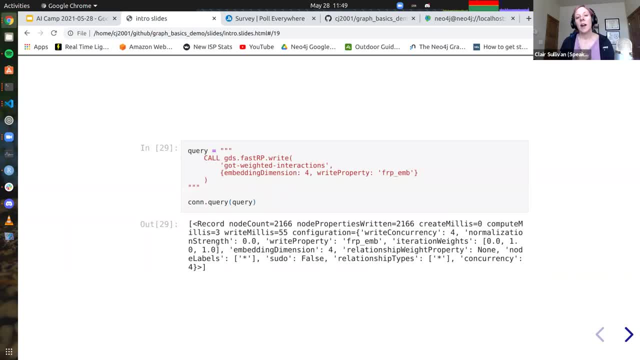 unsupervised learning things that you can do. First we have to create our embeddings, though That's the first step in any machine learning, So I'm using an algorithm here called FastRP- Fast Random Projection. It's just a random walk And we're going to walk around. 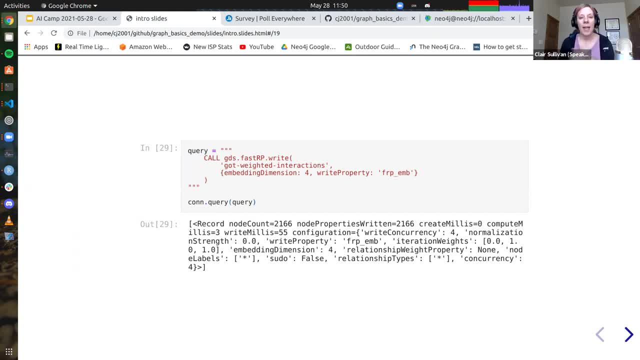 that weighted interaction graph And I'm going to specify my embedding dimension here. So I'm just going to create a four-dimensional vector for each of the nodes within that weighted interactions graph. Okay So, and I'm going to write it out to a property called FRP. 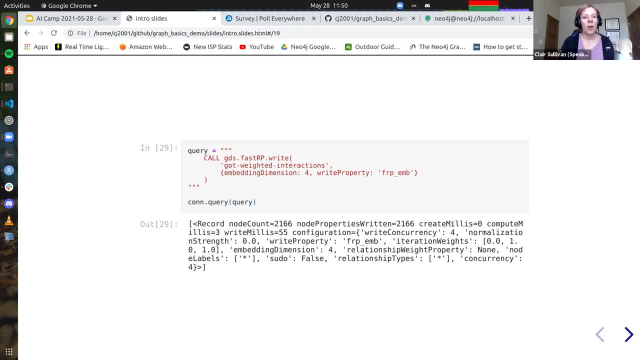 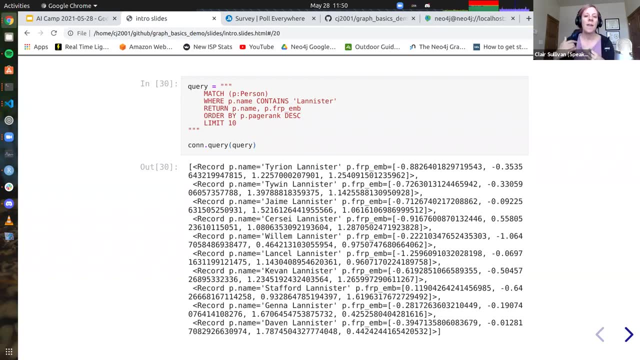 and Fast Random Projection Embedding: Okay, So we're going to run that, Okay. Now let's look at what the embeddings were for some people, ordered by PageRank And you can see: I've got Tyrion Lannister and there's my four-dimensional vector. I've got Tywin Lannister, another. 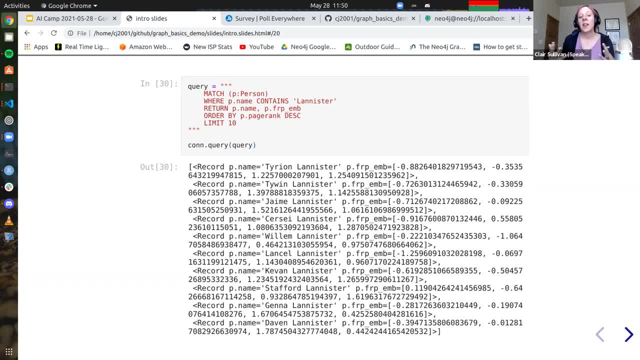 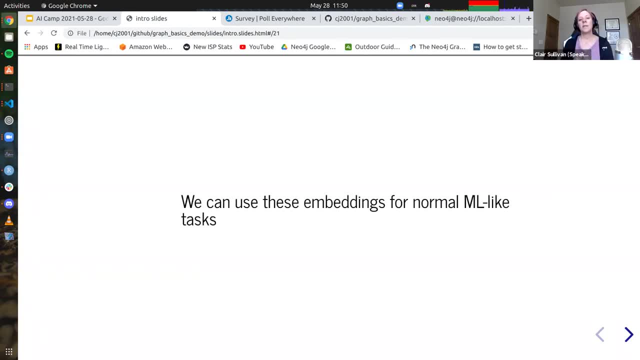 four-dimensional vector. That's all That. all looks like it ran. Let's go now and look at what that means. Okay, What can we do with these embeddings? I'm going to just do some normal machine learning tasks, Like again I said, this is going to be unsupervised machine learning. 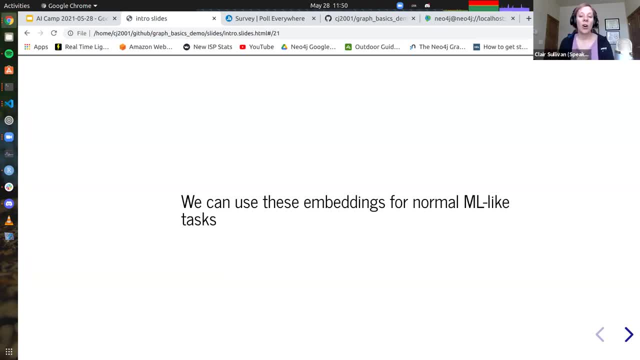 But we'll. I'll kind of give you a hint of where this can go for doing supervised machine learning. Okay, So let's do cosine similarity on two characters, Tywin Lannister and Jamie Lannister. So just like normal cosine similarity. 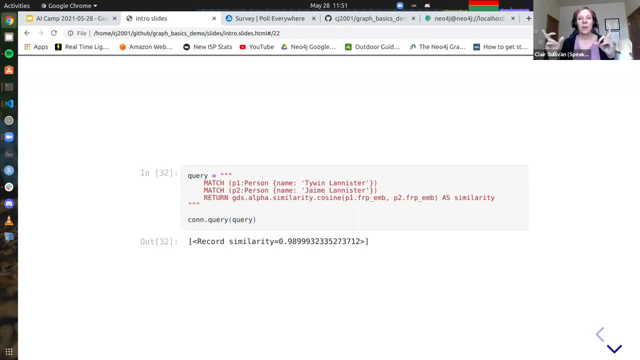 I take their two vectors, their two embeddings, I compute the cosine between them And I see that I have a similarity here. that's pretty high, You know, similarity of 1.0 being completely identical, similarity of zero being not so close at all, And okay So. 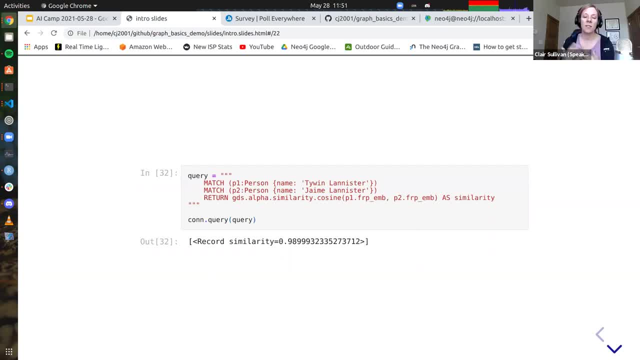 I see a high similarity between these two characters that I that we know. Now I'm going to pick one of these characters and somebody who I had absolutely no idea who they were, So Harma. I think Harma might've been one of the hill tribes people. I don't actually. 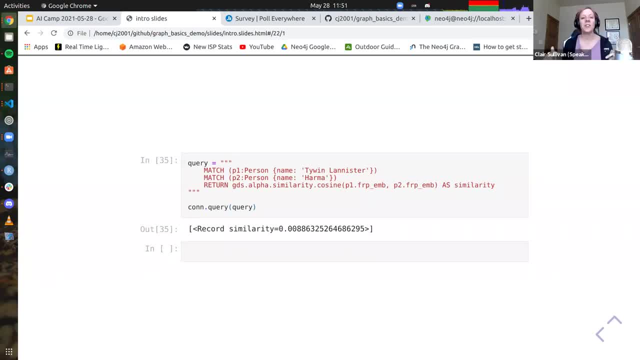 remember, And you can see Tywin Lannister has an incredibly small similarity when compared to this person- that I have no idea who they are. So the idea of using embeddings takes us back to the machine learning that we all know and we all love Anything that you could. 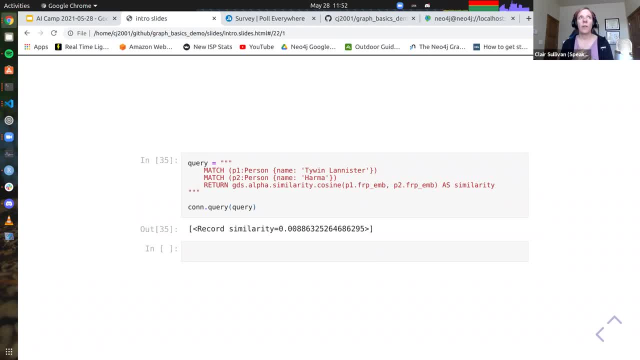 do with a normal vector in machine learning. whether your favorite package is scikit-learn or Keras or whatever, anything that you can do with an embedding in that package, you can do with graph embeddings. So that takes us to the idea of, you know, having supervised. 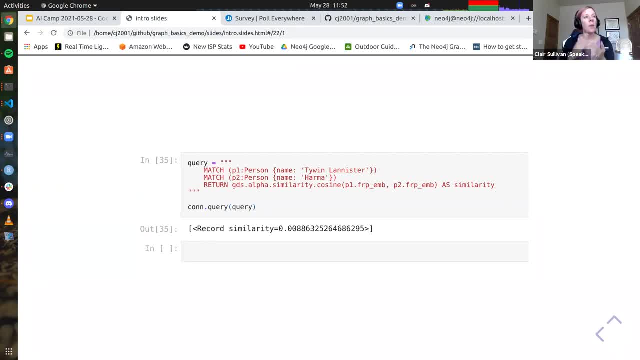 learning, being able to say node classification. I want to know is: you know what is the node? Is my node a person, a place or a thing? Or you know link prediction Is Tywin, Lannister, part of house Tyrell. Spoiler alert: no, But, but the idea of being able to do 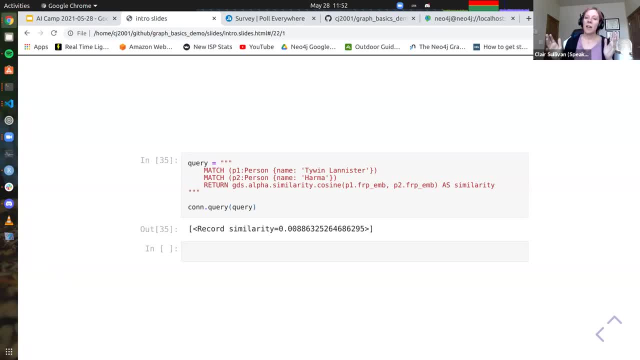 those classic machine learning problems. just with these embeddings you can do it in your own preferred package. Or there's also some of these things that are built in functions to Neo4j. Other things like that are built into NetworkX, But again being able to do it in a database. 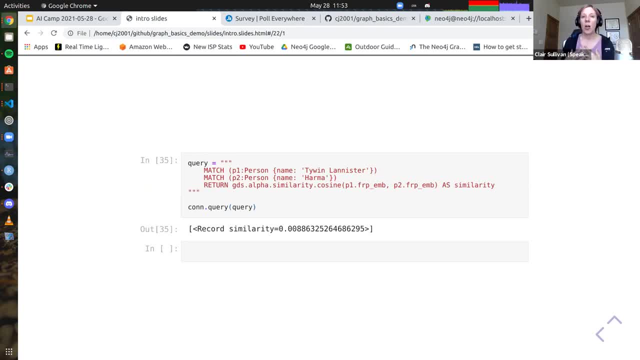 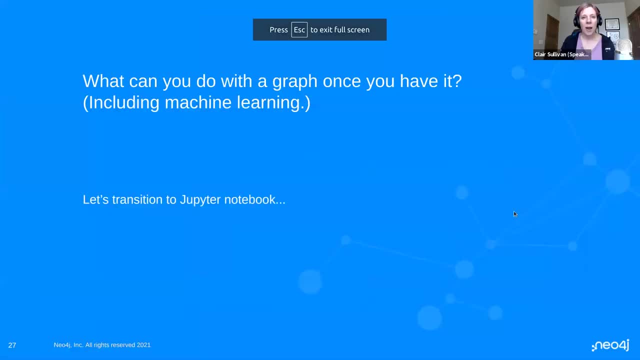 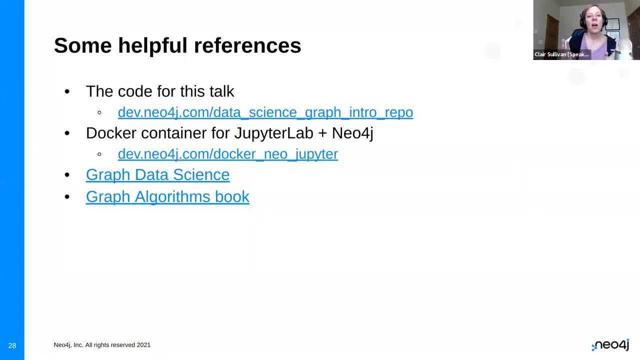 as you know from some of your larger data problems, generally helps. They're generally more scalable. Okay, So let's go back now to our Google slides, And I'm going to wrap things up here. Okay, First off, the links. Okay, You're going to want to go get this. 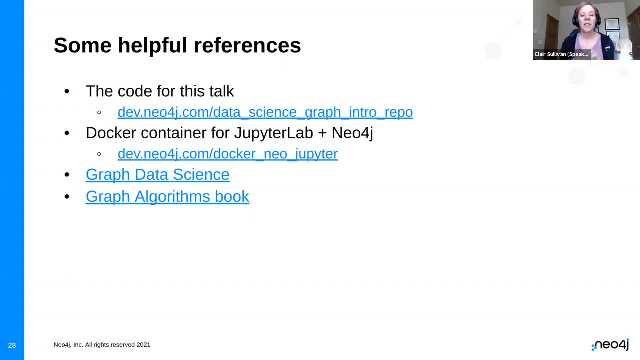 data science graph- intro repo. Okay, That's, that's on my GitHub And for those of you who can't write that down fast enough, I'm going to try to leave this screen up for a while. You can go and find me on Twitter. My Twitter handle is Cjlovesdata1.. I think. 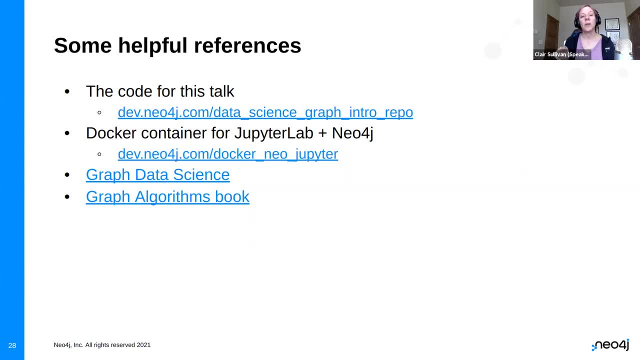 that's on my last slide here, And I've actually tweeted out the link to that first repo. The second repo is something that I didn't talk about too much, which is how I'm running this. A lot of data scientists we know like running things in Docker containers. This demonstration. 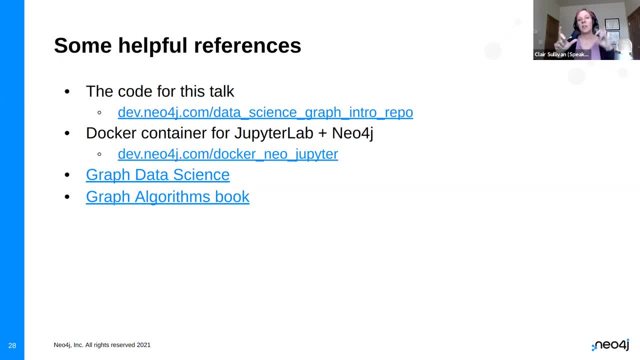 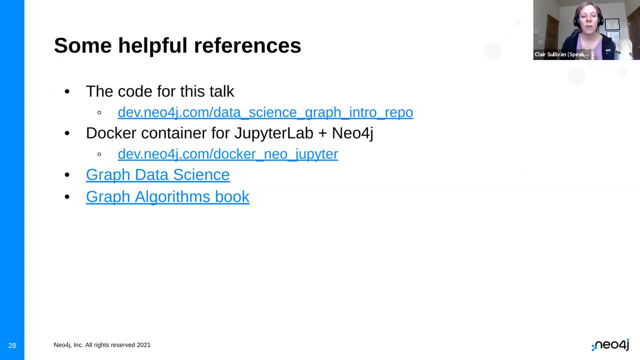 link. it'll eventually get you to the repo where you can do that yourself. I mentioned the graph data science library. There's a link to the API docs there, And then there's also this book here: graph algorithms. Hang on, I have it right here. It never leaves. 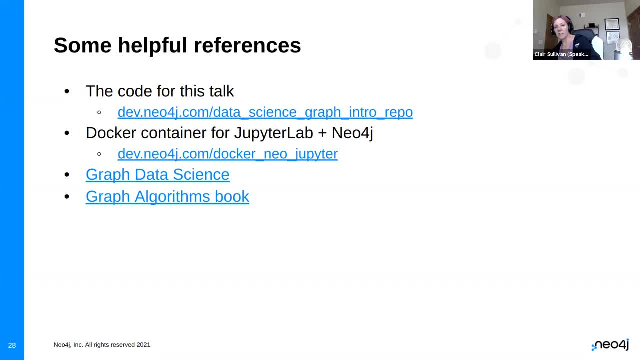 my side because it's really wonderful. So graph algorithms is. it just kind of goes through everything and describes it, you know, describes all of these algorithms, how they work. It's a great resource put out by O'Reilly and it's actually available for a free download through. 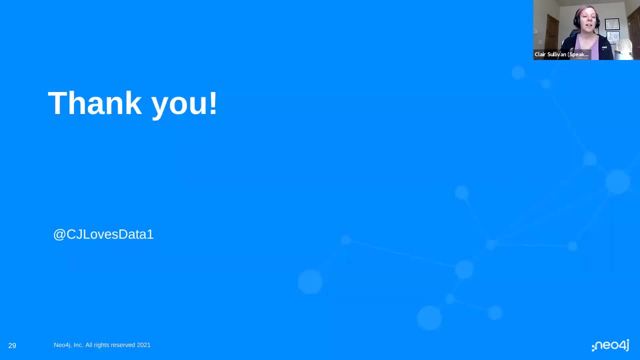 that link, And so I think that's my last side. There's my Twitter handle again. You can just go and look at what my most recent tweet was. I think I automated it to come out within one minute from now, I believe, So you can go grab those repo links from there Again. 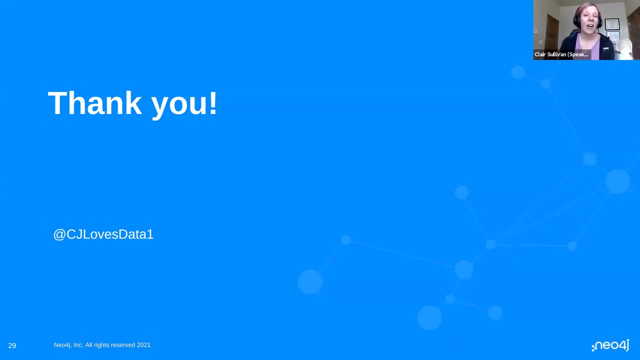 I want to thank you. Thank you for attending and sticking it out And, I guess, at this point, the best way to take questions. Bill, do you think it's voice or is it in the chat? I think there's some questions in the chat and I think we can just go through them from. 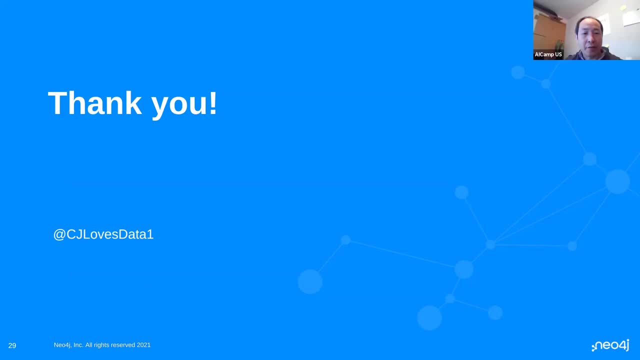 the top, From the top. I just want to remind everyone. if you have questions, please feel free to post in the room chat. By the way, my question is: do you have any questions? Yes, If you have any questions, please type in the chat. Make sure you select to everyone. 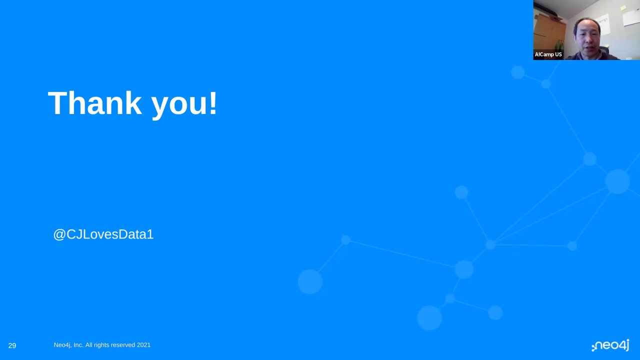 so we can all see the messages, the questions, not just to the host. If you prefer to speak to us questions, raise your hand and I will admit you to speak. Okay, I'm scrolling through to find the first question. Glad that everybody's introducing. 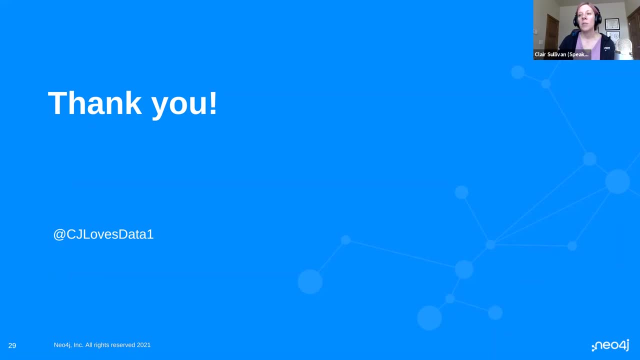 themselves posting links here. How is Neo machine learning different from neoclassical deep learning? I'm going to stop here, Okay, I'm going to stop. Okay, So there's a question? Oh, this was a direct message. I'm sorry This wasn't in the full chat. So inputs and 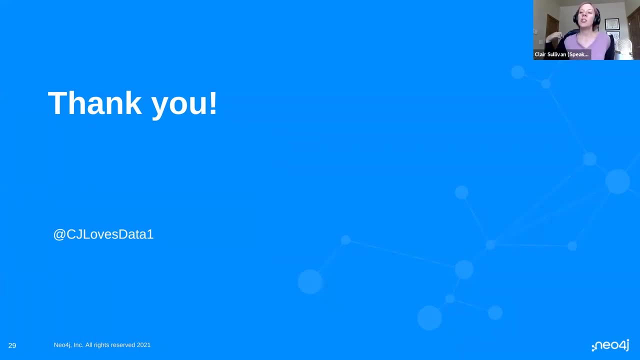 groups. I'm going to need a little more information here from you on this one, Arthur. if you're still on the phone or on the call, Sorry, I'm dating myself now, So I just going to talk in general terms about 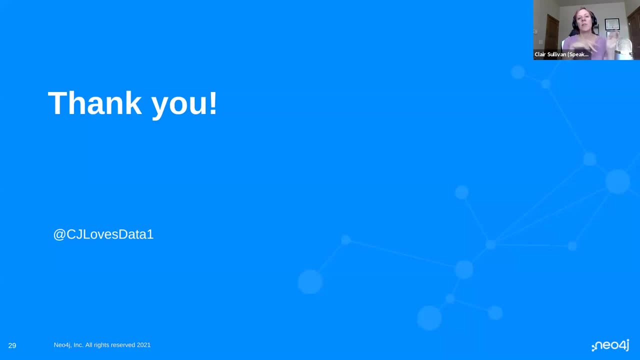 terms about the machine learning that's built within the Neo4j versus what you can do with deep learning, And it boils down to where do you want to do the calculation? So node classification, for instance, is a built-in machine learning function in Neo4j, So I can let Neo4j do that. 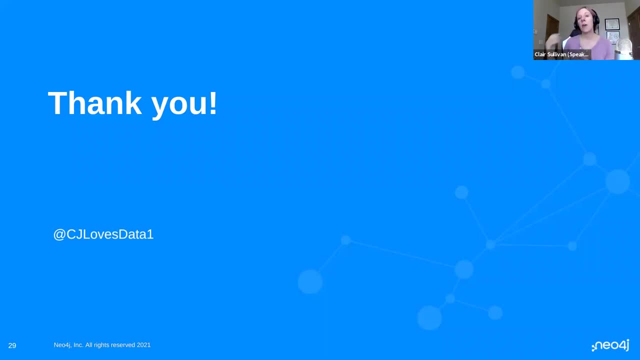 I could also do that if I have the embeddings in my own deep learning function. So the key here is: I've got to get embeddings. Now you could pull the entire graph down into Python without embeddings and you can run your own embedding software on it. There's the group at Stanford. They are 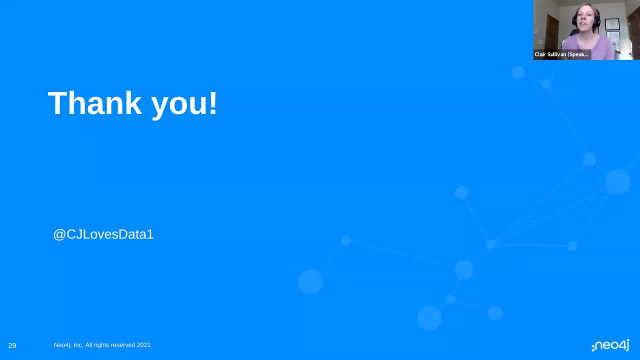 legendary at this. They're the ones who have invented a lot of these embedding algorithms and you can run their stuff and it works pretty well, But running it in Python. as we all know, Python is not a compiled language, So therefore Python can be pretty slow in. 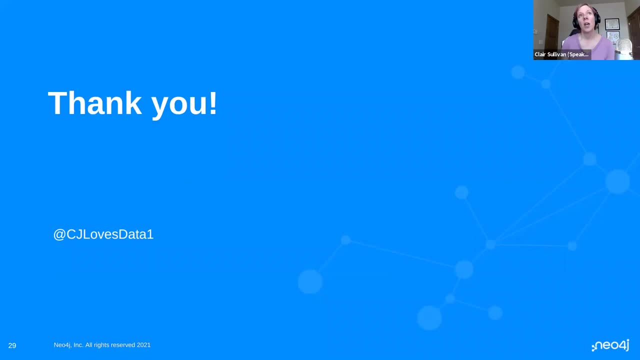 doing this. So my view is, you know, in the case of Neo, let the graph database do what it's good at And it's good at calculating embeddings. So I would suck those embeddings down from Neo if you want to do your own pipeline or there's node classification and link prediction that exist. 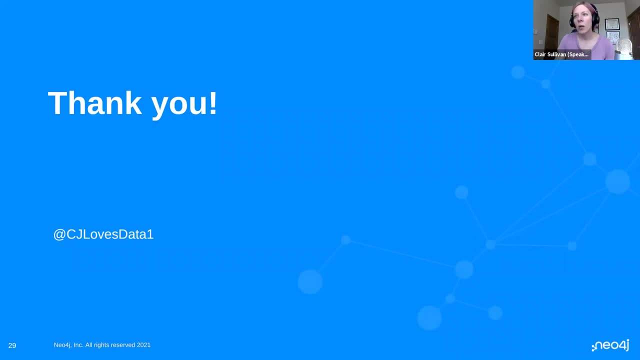 within Neo already. Okay, Let me go through. Let's see What's the next question. I attended the NLP class. Great to stay current, Oh, okay. Yes, NLP is a subject near and dear to my heart. Okay, What? 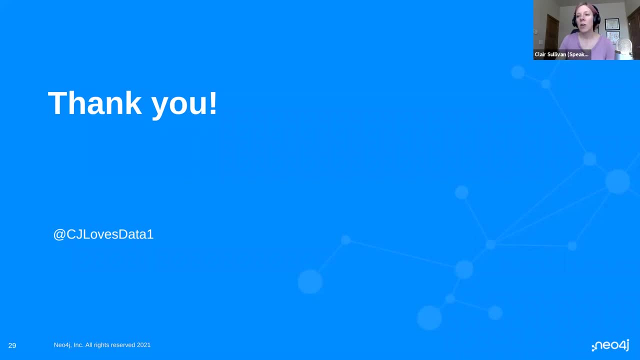 channel on Slack. What is churn? Okay, Churn is stop using the product. It can be even deleting your account. Let's see What is MNIST. It looks like a lot of people were able to answer that one, So let's see Scrolling through. Storm coming- Not today, but I still have snow. 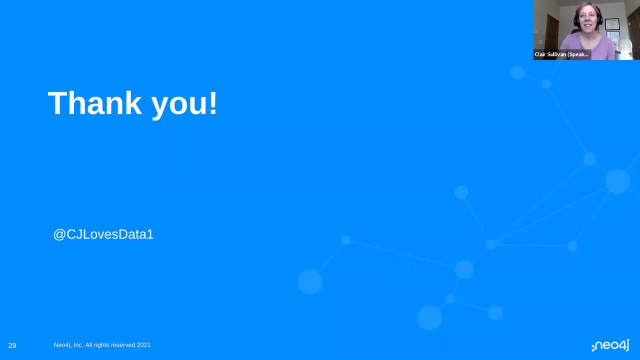 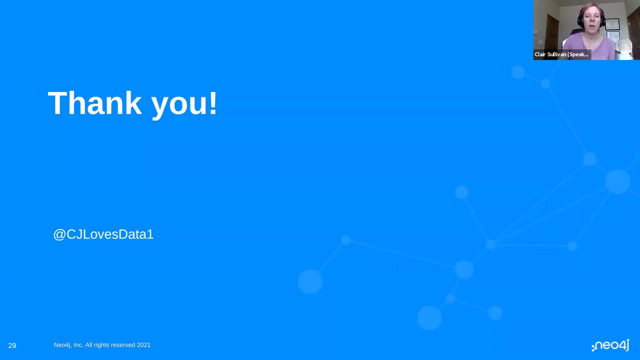 question. And where have you seen good, significant lift in performance from it? Okay, Glad you asked this. So common ways: there's two ways that you could come up with these features or these vectors or embeddings, whatever you want to call it. 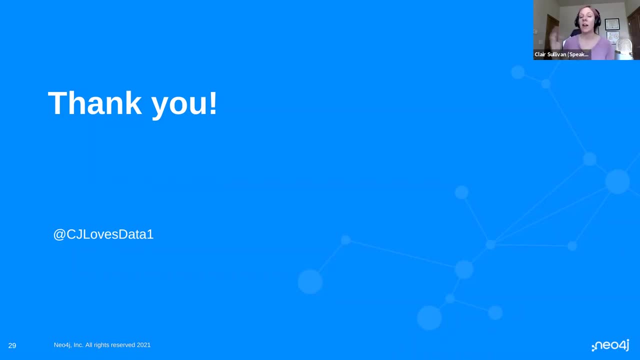 The first. you know, a lot of times we go and we get our own features right. We say, okay, I've got these users and I want to know what dates did they create their accounts And are they, what's their age? And you know you can start assembling these features yourself And that 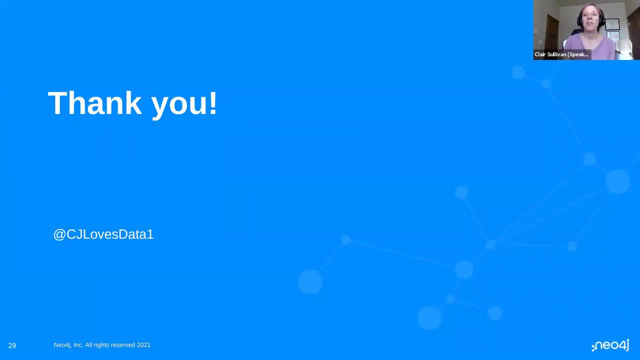 works totally within a graph database, within graphs of any sort. The catch with that is: think about how big I can get. I can get a lot of data. I can get a lot of data. I can get a lot of data. I can make my embeddings. You know, I showed you a four-dimensional vector I could have. 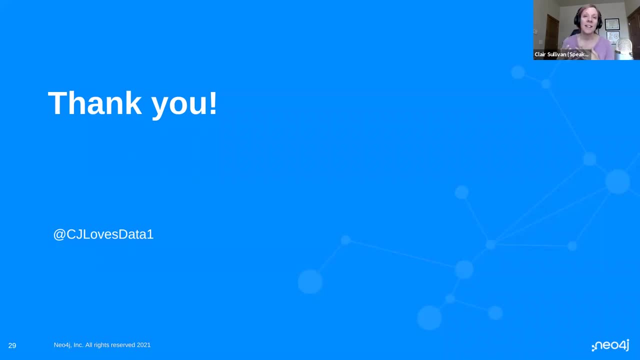 limitless number of dimensions. Now, obviously that's not a good idea. You need to consider how many data points are within your data set. So you want to have fewer embeddings by a fair bit than what you have in your data set. So let's say I had enough data points to create 128 dimensional. 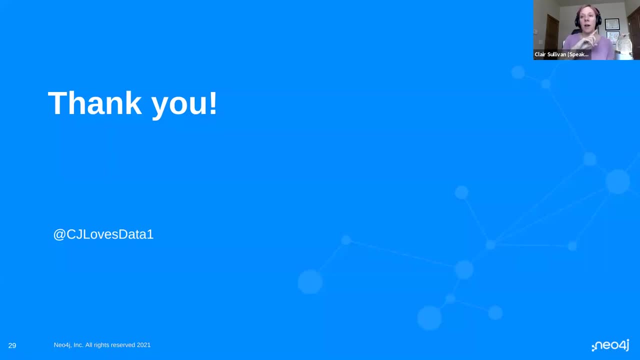 vector. If you want to compete with the common ways to featurize data, then I have to come up with you know, like 128. And then I have to come up with you know, like 128. And then I have to. 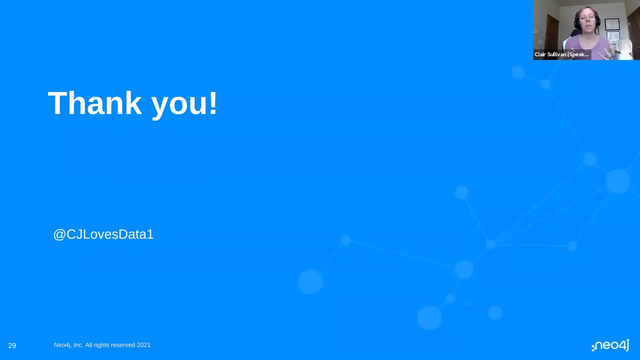 create 128 different things, different columns, that I'm going to bring into my table. So where have I seen good lift and performance from it? This is a complicated question And I'll tell you that people are still answering this question. But if you were to do something like, go on to. 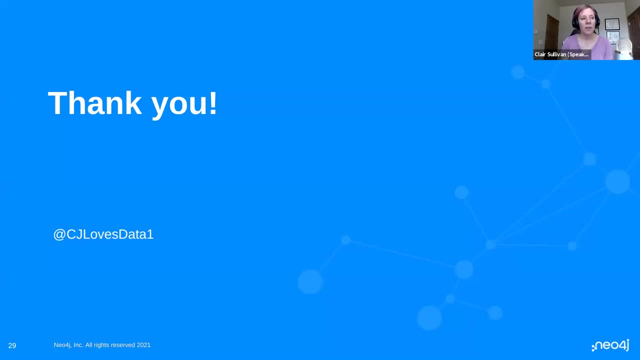 Medium and there's a post out there you're going to. I'm going to enter this guy's name in the chat. His name is Christophe Nays. Okay, And Christophe wrote this great article where he looked at, kind of one of the common 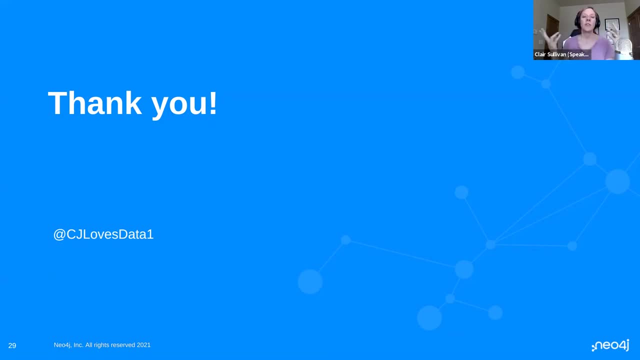 graphs and it's called the CORA data set. It's looking at different cross references within a whole bunch of research articles And what he was looking at there's this deep learning package called graph neural networks by DGL deep graph learning, And what he was able to show was 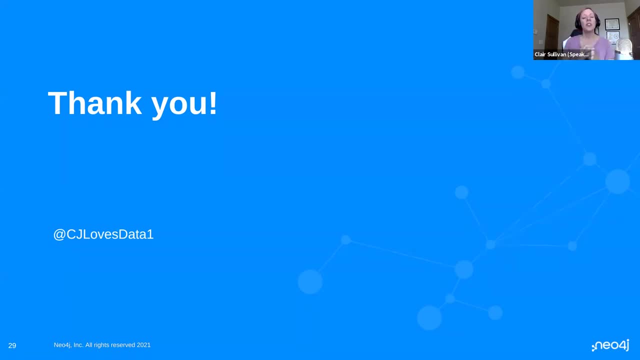 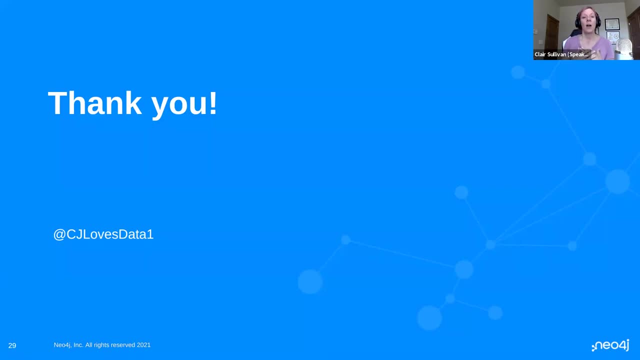 150 nodes within a graph- huge accuracy, So so, yeah, I would definitely call that a significant lift in performance. Let's see. need help with using the repos, Will you guy? Okay, Any mention of computer vision application using graph neural network? Yes, if you go into. 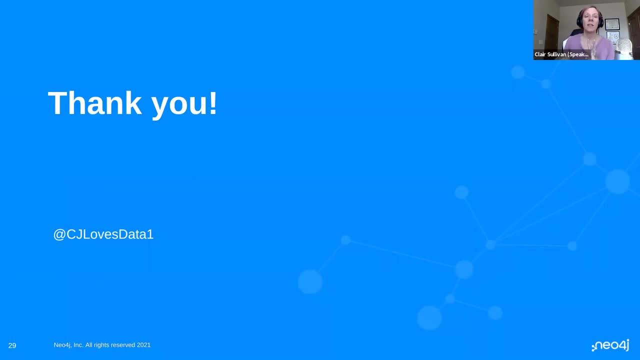 if you grab this repo, go into the slides. there is, it's not on. it might be on the MNIST page. it might be on the. there's a link In there that shows people doing imaging image analysis with graphs, If you Google it. 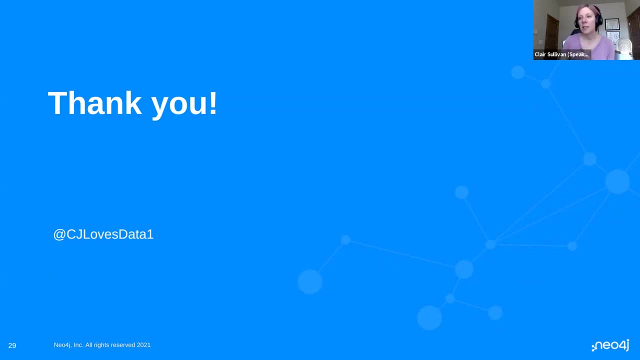 there's some really great posts out there. Let's see. at the end you did a variety of database manipulations, but I expected to see results as graphs because, okay Yeah, I could have shown these all as graphs, You know, let me just quickly go back to my screen here. And I have 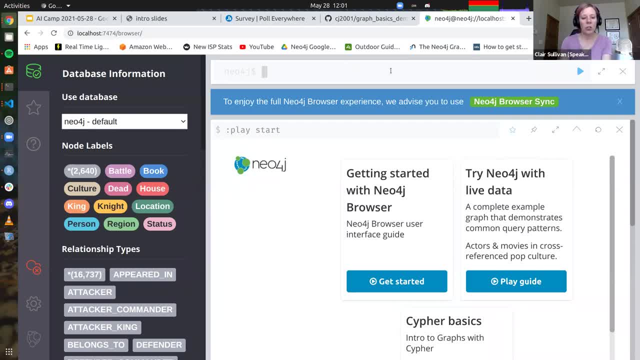 uh, let's say I were to show. um, I'm going to match a person, I'm just going to do this really quick here, So forgive my horrible typing. Um, and I'm going to say that they have what did I call it Community? 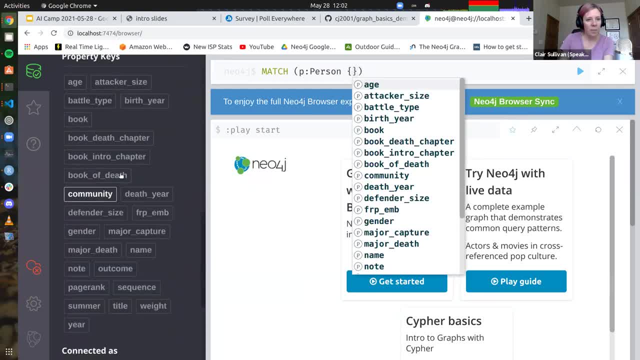 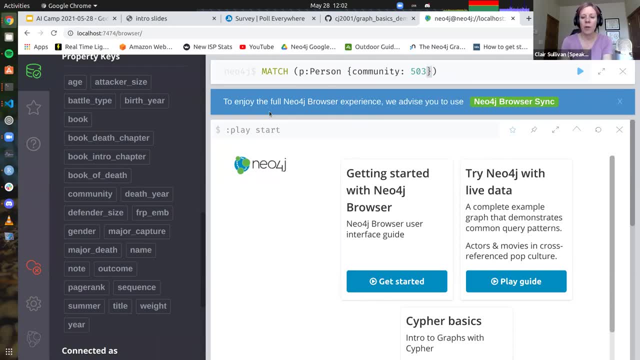 ID something: um community, maybe match um community. Um and I, if I remember correctly, 503, was a Stark and um, they're going to be connected through, let's say through interacts. Now, this is probably. you know the horrors of doing this live and 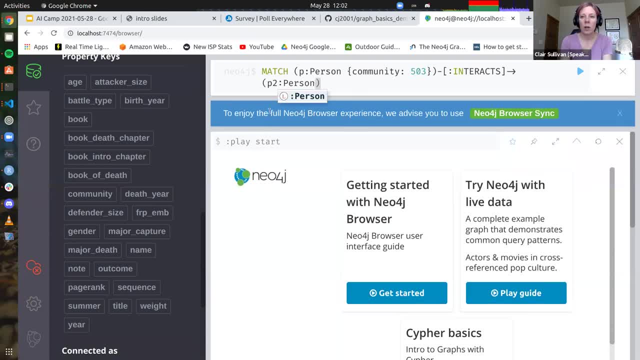 they're going to interact with some other person. we're going to call P2.. Um, and we're going to then return P and P2, and we're going to order by: uh, let's go P, but their page rank Um. 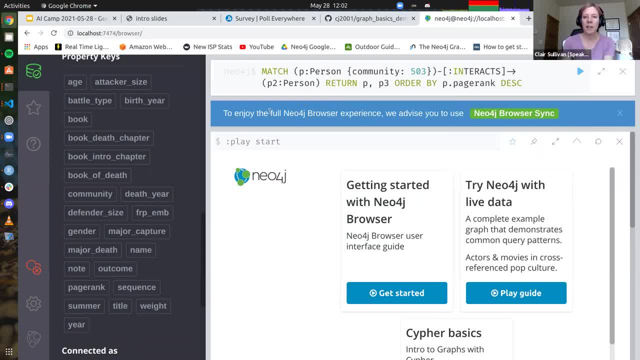 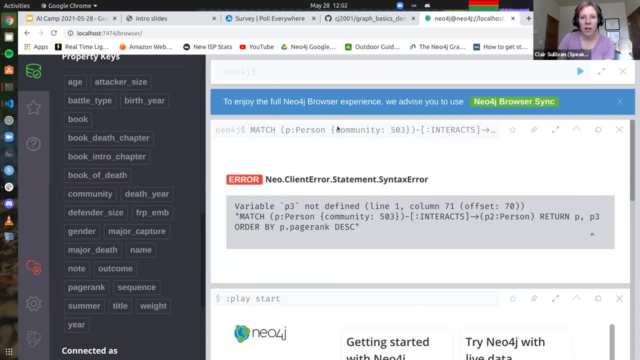 and we're going to say order by that descending. So I hope you can kind of see a little similarity now watch: this is going to blow up just cause that's my live lock. Um, P3.. Yes, Cause I put a. 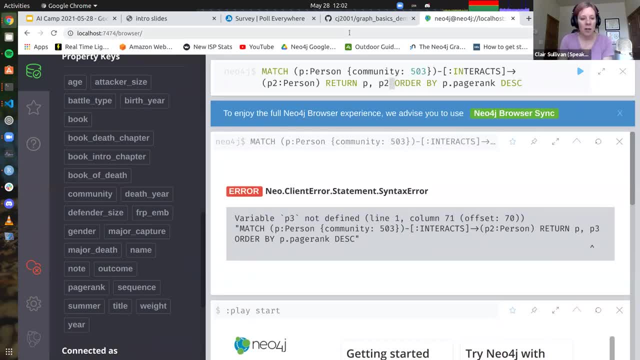 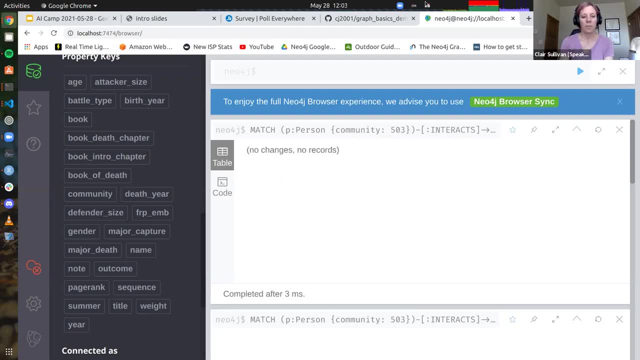 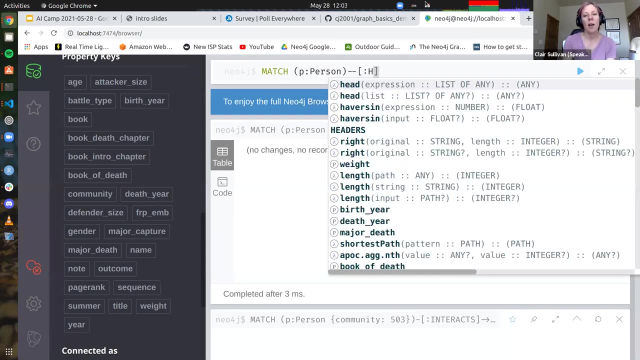 typo in there. Sorry, You guys are getting to watch me fat finger this, Okay, Uh, let's see no changes in records. Okay, Well, let me just get the people Um okay, And we're going to say connected to um H house. I'm going to return P and. 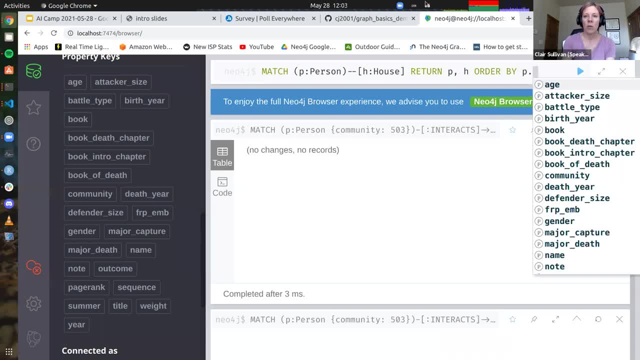 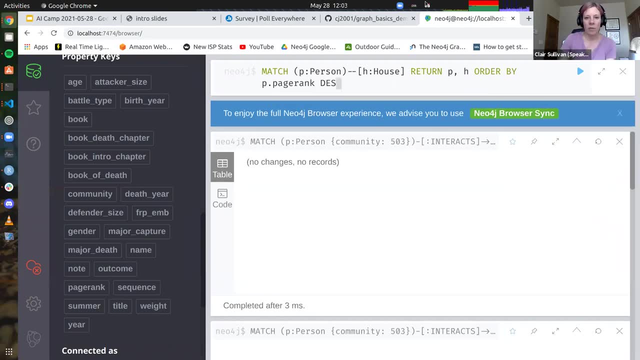 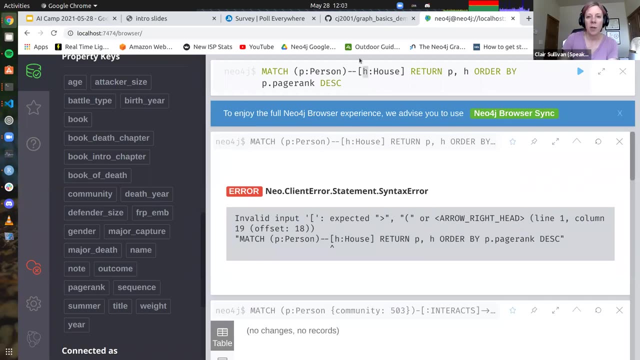 H or by P page rank descending. Let's see if that works, Okay So, oh, yes, So this is great. I love typing while you get to watch me screw up, but that was because I tried to say house was an edge. 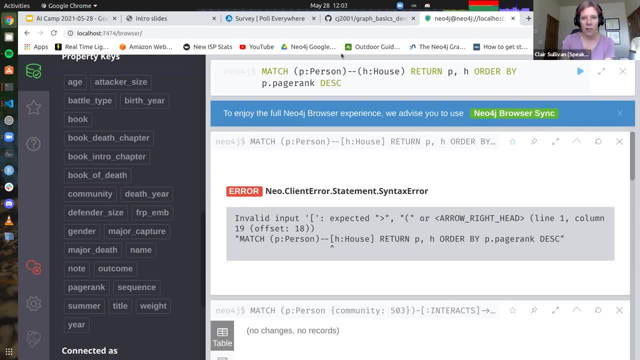 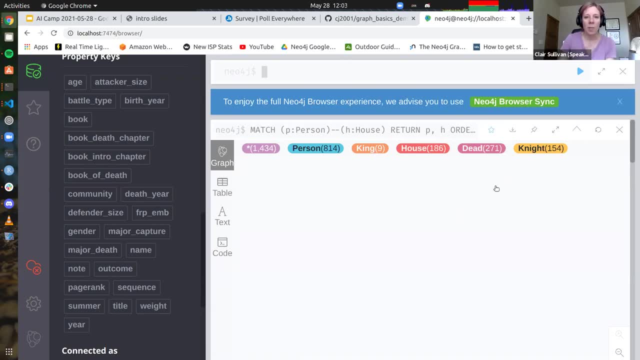 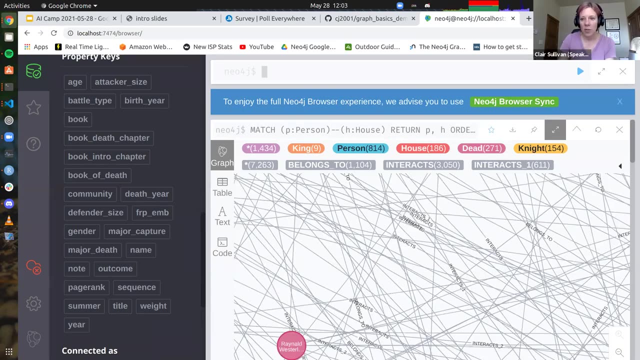 by square brackets rather than a node by round brackets. Where'd it go? Okay, So here I can see. I have a graph. Um, it will someday pop into existence. Sometimes these visualizations are kind of slow. Let me try to blow this up a bit. So. 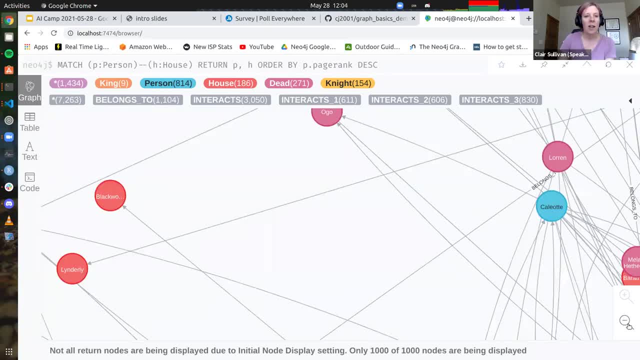 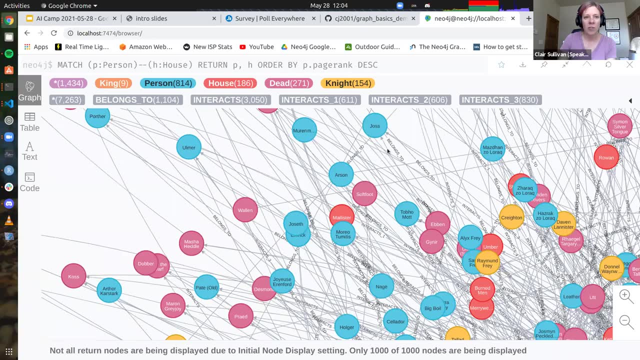 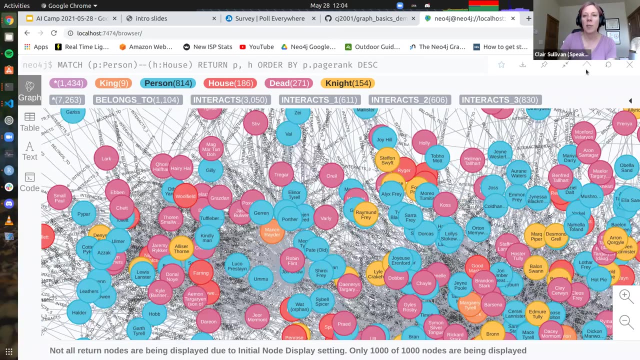 you know I could start now filtering on um. you know I I only grabbed the top page rank folks here um because I only have 1400 people who are being plotted here. I could say I could limit this. 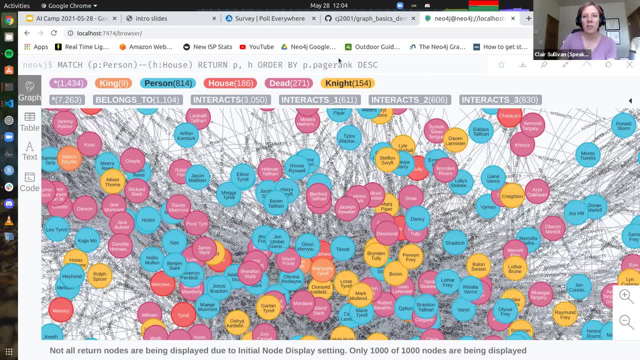 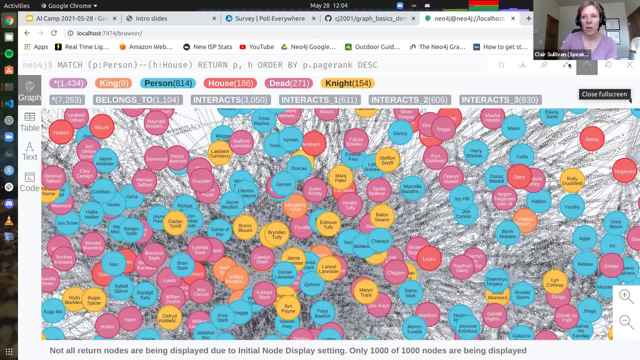 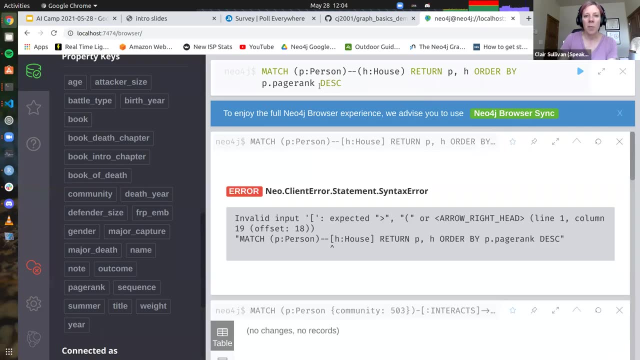 Um, in fact, let me do that because this is going to turn into a mess real fast. Um, come on, Okay, Let's say let's get rid of this, Cause sometimes those images can take up a fair bit of memory. I'm going to say: limit this to 20 hits, Okay, And we're just going to go on that. 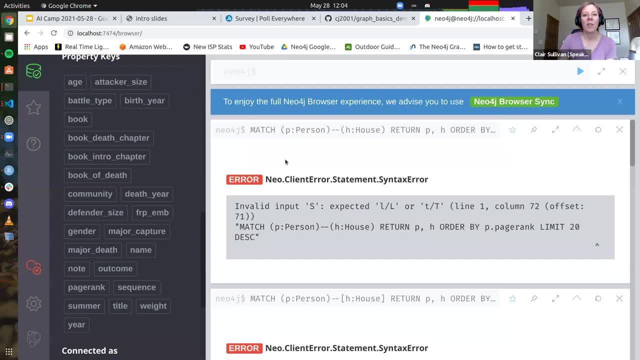 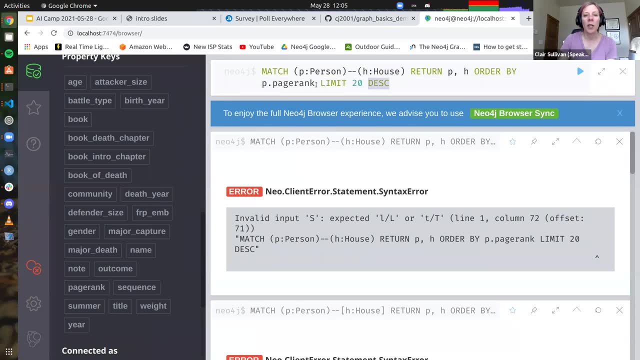 Cool, Of course. Um, Oh, yeah, again, typos. Um, hopefully, though, um, as I go through my various typos, you're getting the point here. Um, you know, and I could order this in any number of things that I calculate, uh, no limit. Okay, Again, I'm really sorry that. 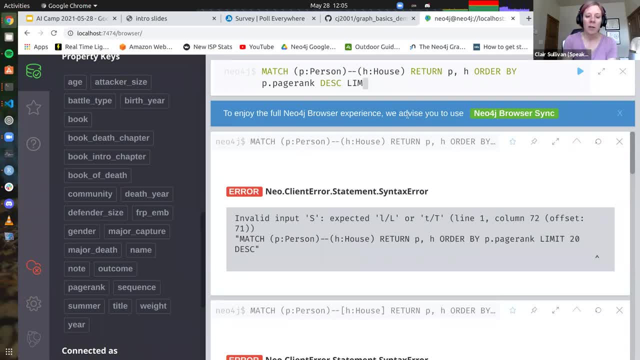 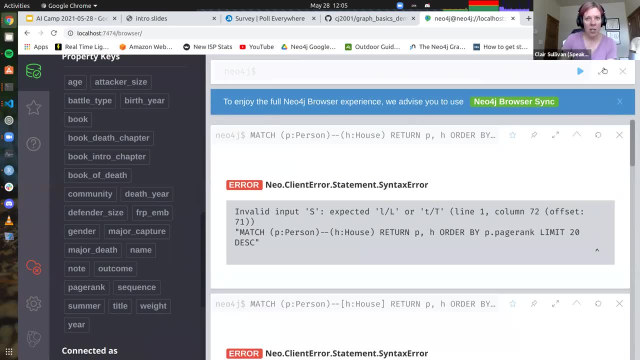 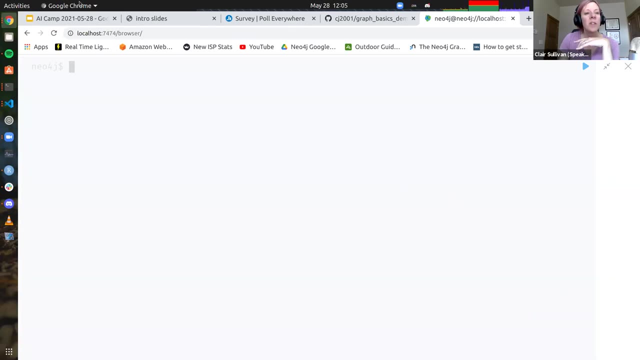 you're watching me screw up my typing. Okay, Let's see if there's connections between our top 20 and houses, And it looks like there will be. once um. once it renders fully Um, sometimes the memory gets a bit bogged down. 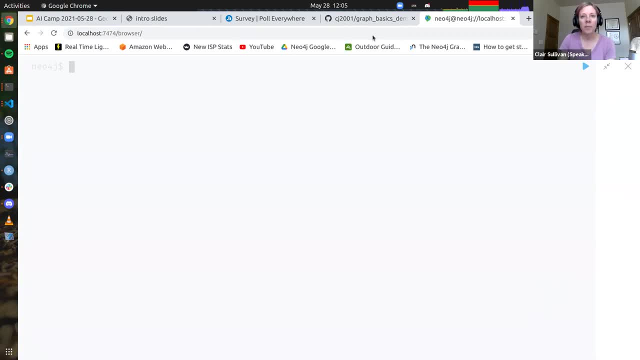 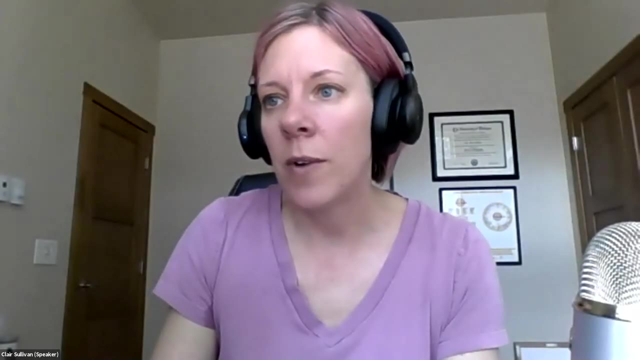 in here and I just have to refresh browser. Um, okay, So let's, I lost my question window, So I'm going to stop sharing. Um, I'm going to get back to the chat. Um, I'm going to get my question window back, Okay. Um, how is Neo ML different? Okay, We answered that one. 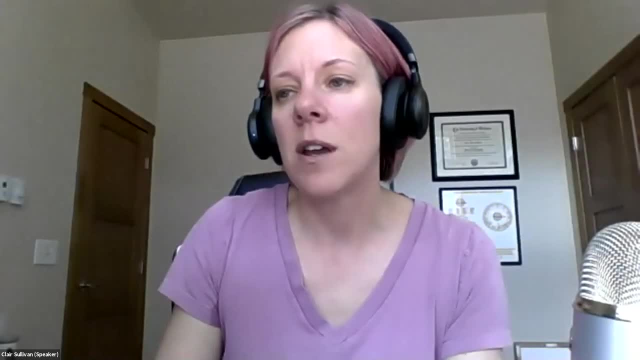 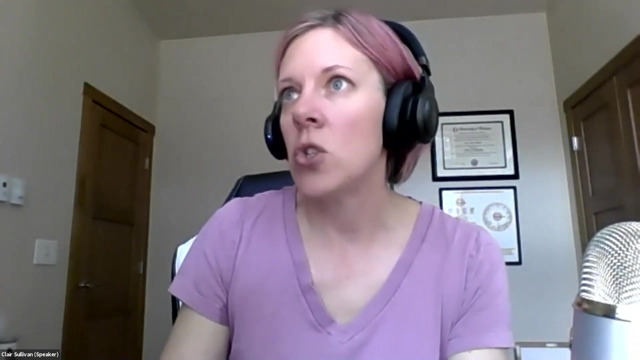 already. Uh, Cora something. Uh, okay, Research guy in medium. Can you please mention this again? Okay, So, um, the research guy in medium is. his name is Christoph, And if you give me two seconds I can probably actually drop the link in. 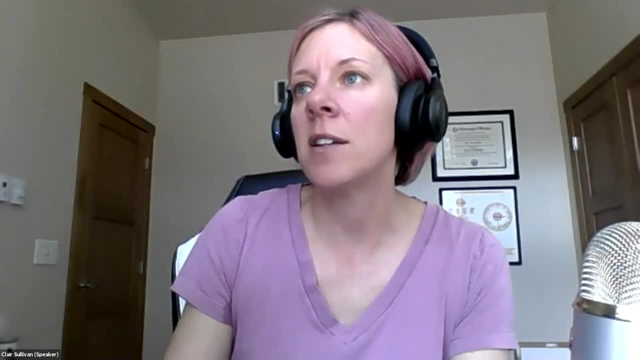 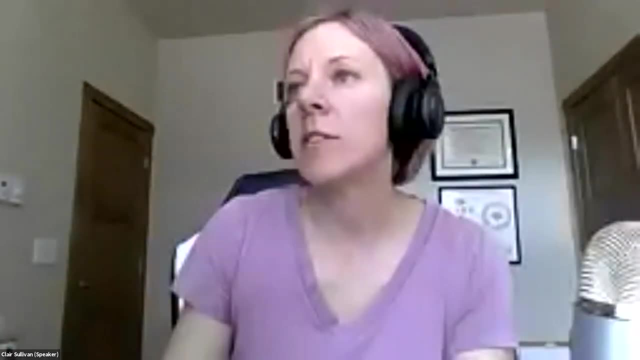 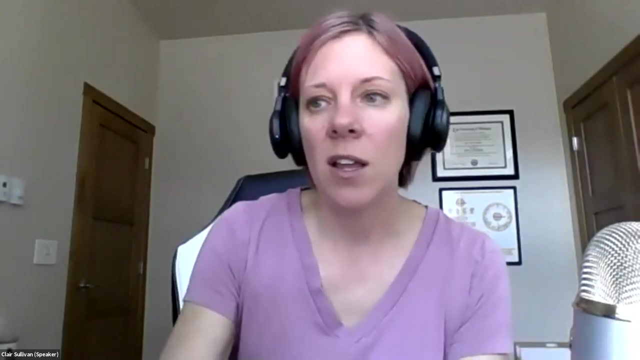 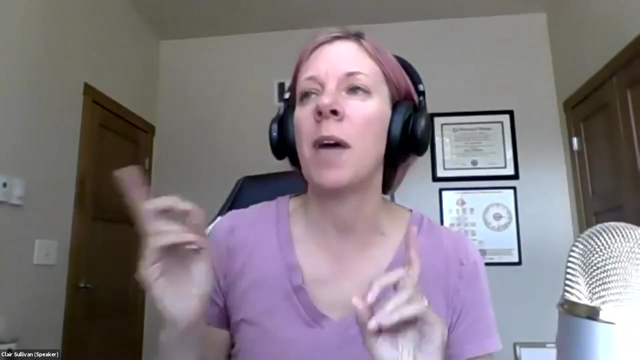 Slack to his presentation. Um, okay, This here, give me a sec. This is the starter post he has on using DGL And he looks at um several other deep learning algorithms, um, in other posts. Um, oh, that's deep minds graph debt, Sorry, DGL is his next post, So if you go, look Christoph up. 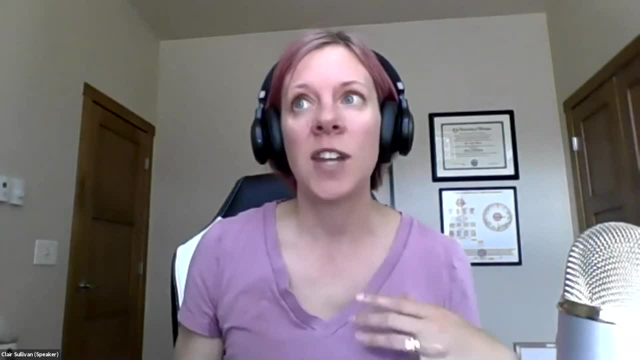 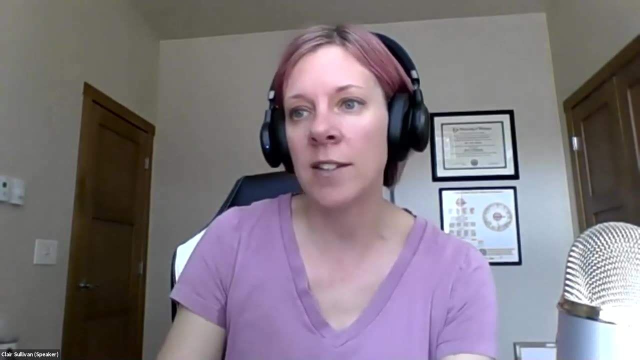 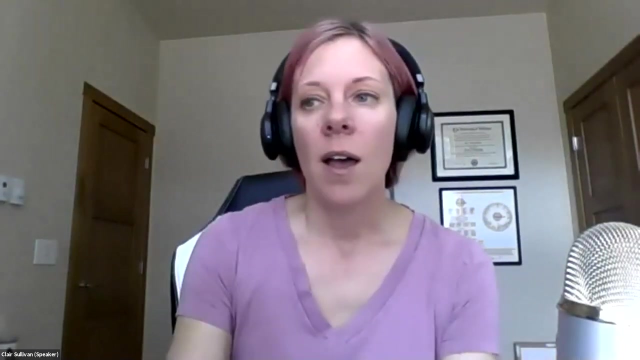 on medium, what you will find is that post and, um, his DGL post, And those are two great places to get started on. Where is the post last name? Um, there you go. Somebody just posted that, uh, Christoph nays. Okay, Um, so are there any last questions, Cause my window isn't. 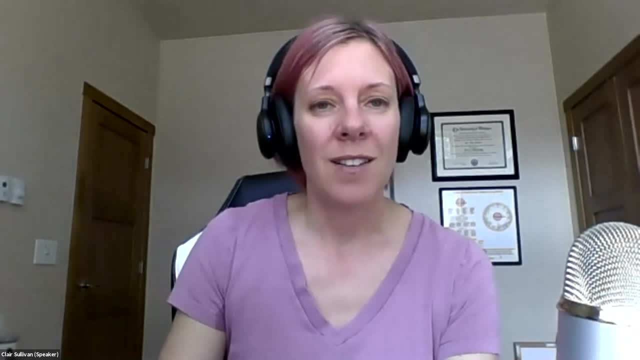 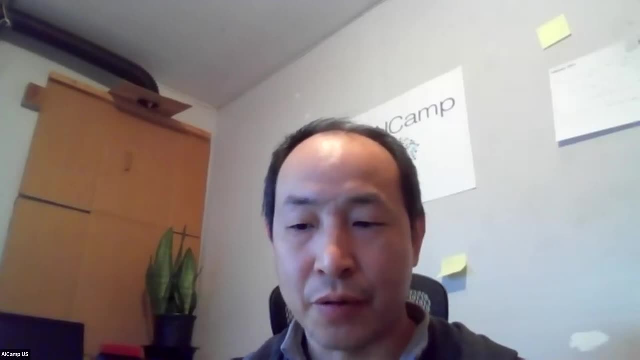 scrolling any lower. So I assume that means: uh, that was the last question. Uh, great, Yeah, I think I. that's all our questions, Uh, but again, if anybody have, we have a few minutes over time, but that's fine. Uh, if anybody has last minute questions, uh, you feel free to. 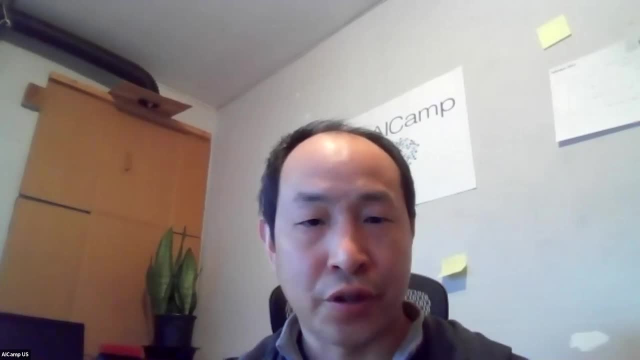 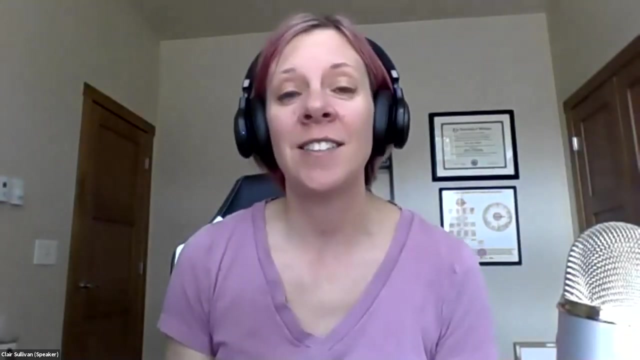 post in the chat And also I actually unmute all of you. Um, you know, you can unmute yourself if you prefer to speak to us questions. I see all the all of you saying thank you, You're welcome And thank you all for attending It's, it's really. 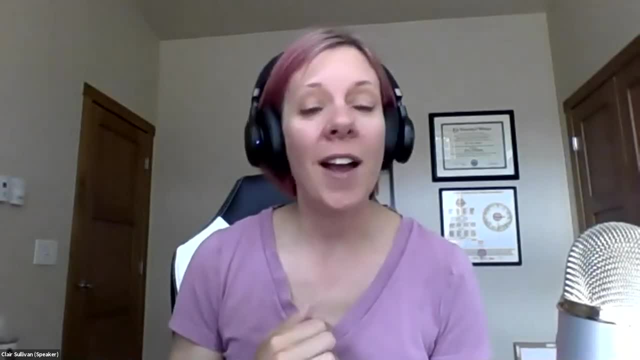 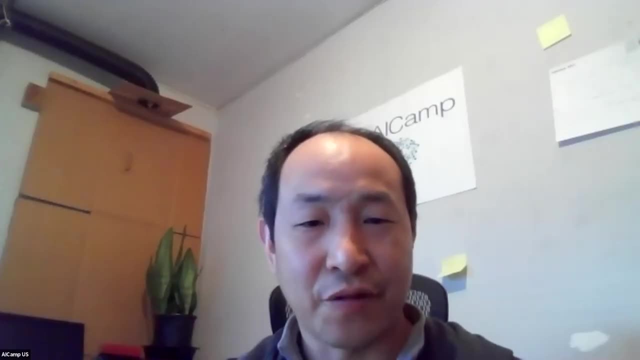 great again seeing so many people here who might be interested in graphs, and so many different countries represented. So thank you, Great, Great, Thanks a lot. Thanks, Claire, for the great presentations. Uh, I know there's online events, but I still want to give you a kind of 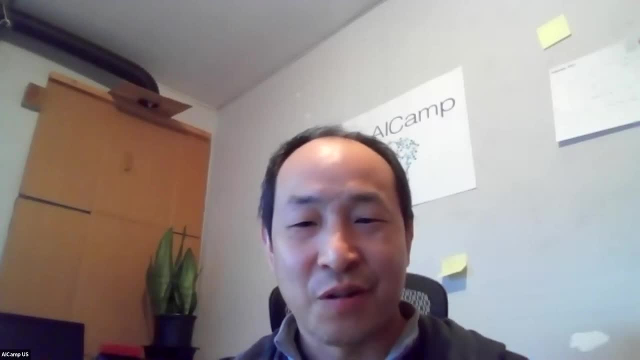 a visual applause, a round of applause. So for the folks still on the line, if you can turn on your cameras, if you want or turn on unmute yourself, let's give Claire a round of applause. Thank you very much. Thanks a lot everyone for joining us And again, the